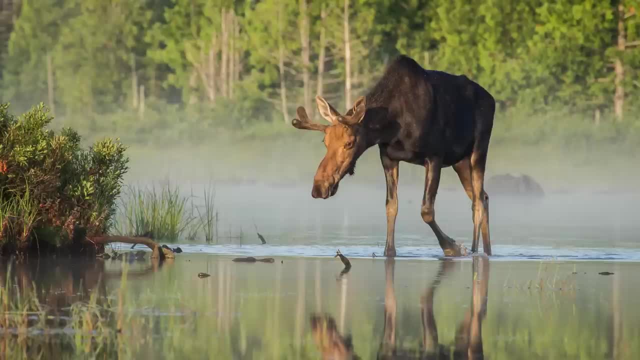 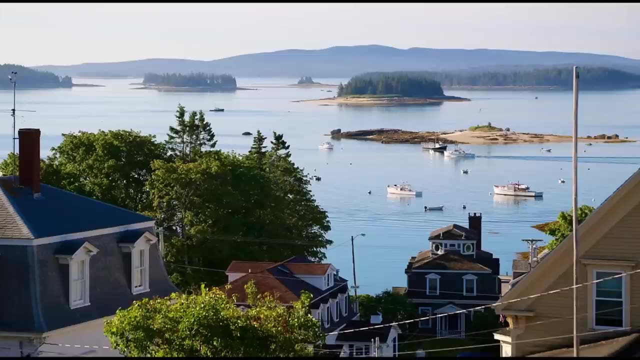 far removed from any city or town. Thousands of moose roam wild in the forest that surround beautiful mountains and lakes, while the small fishing villages that line an island-filled coast look like they've barely changed as the decades have gone by. It's home to one of the only 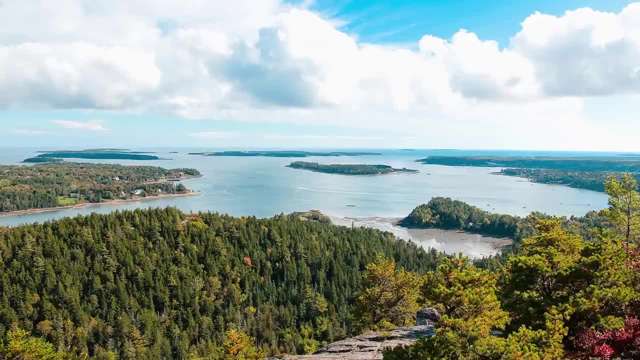 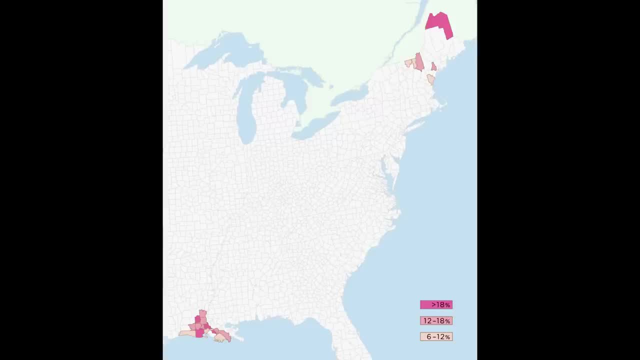 national parks in the eastern US, borders more Canadian provinces than US states and has the country's highest proportion of French speakers, most of whom live in remote towns along the border, With a strong maritime tradition, a beautiful landscape and an 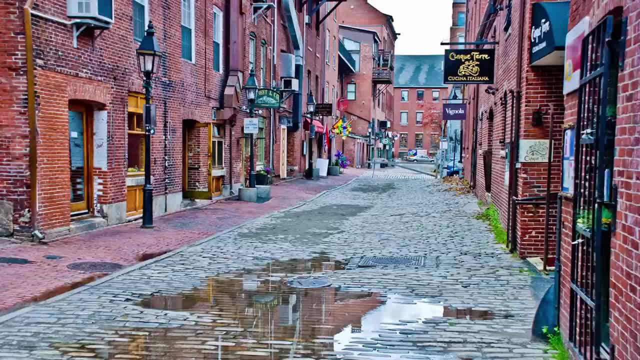 interesting culture. Maine is a unique and fascinating state and the 24th place I'll cover in The US Explained- a 56-part series on every state, territory and federal district in the country. Hello and welcome to. That is Interesting. I'm your host, Carter. This is The US Explained. 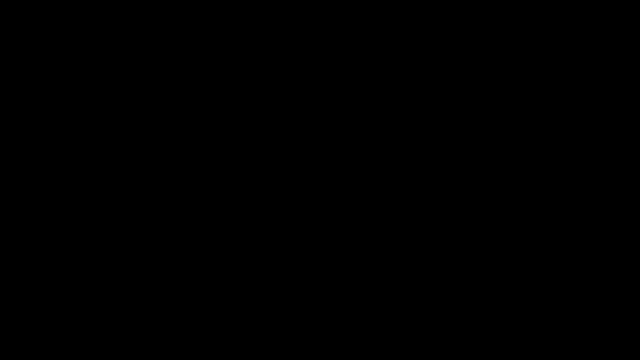 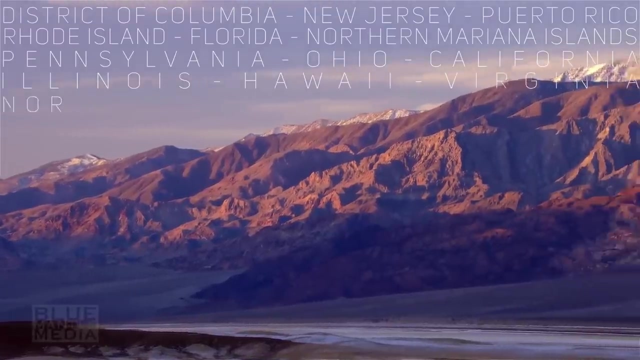 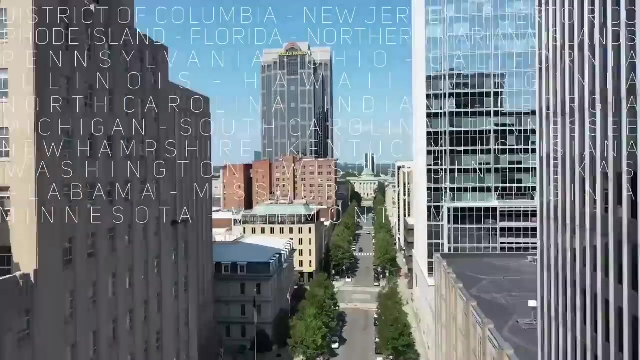 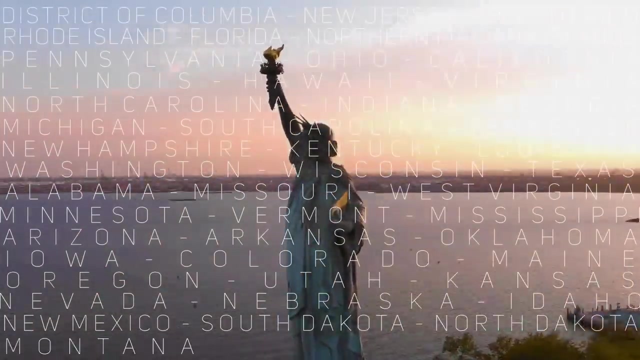 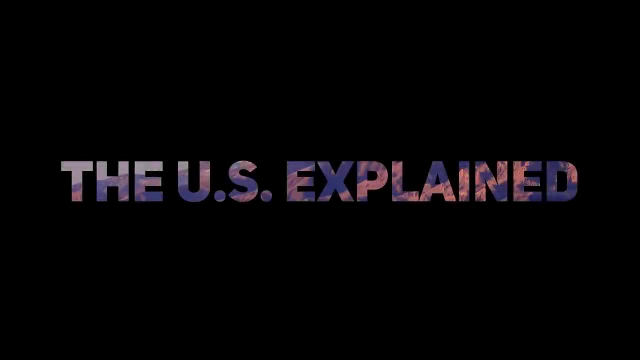 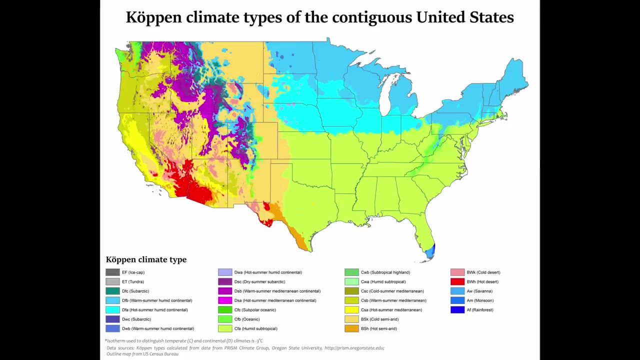 episode 24, Maine. That is Interesting. I'm your host, Carter. This is The US Explained episode 24, Maine. According to the Kepin climate classification, Maine sits almost entirely in the warm summer, humid continental climate zone, with high humidity, four distinct seasons. 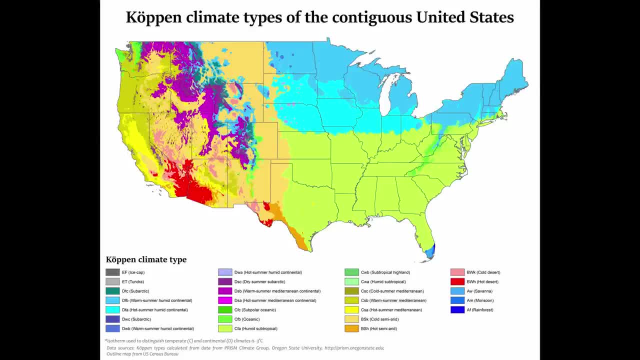 warm summers and very cold, snowy winters. It's a similar climate to that found in New Hampshire, Vermont and upstate New York, all the way through Michigan, Wisconsin, Minnesota and North Dakota. The few exceptions are parts of a few coastal islands which have 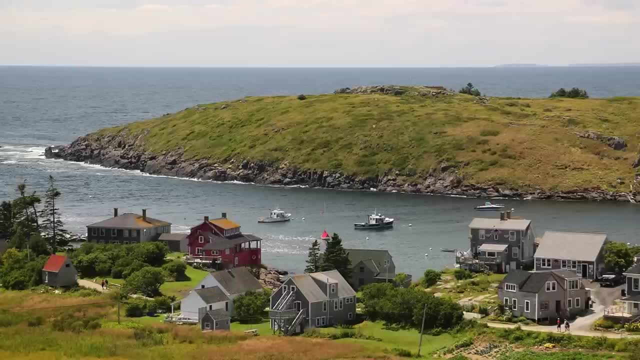 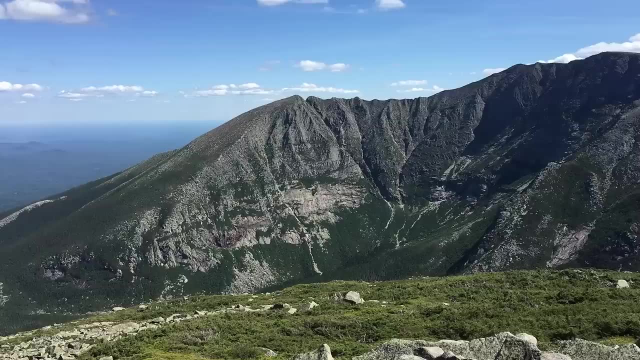 oceanic climates more moderate due to the effect of the ocean, and the very tip of Mount Katahdin, which, at 5,269 feet or 1,606 meters, is the highest point in the state and marks the end of. 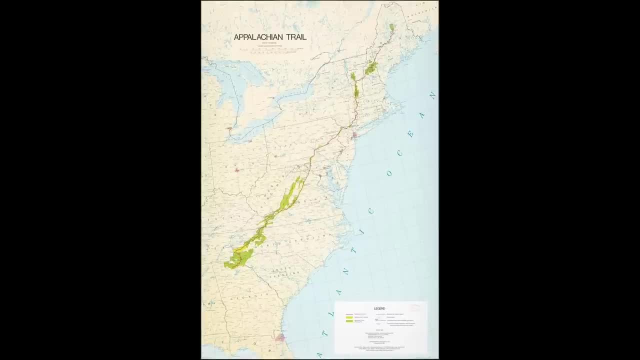 the famous Appalachian Trail, which stretches well over 2,000 miles to the southeast, to its start at Springer Mountain in Georgia. That is the highest point in the state and marks the end of the famous Appalachian Trail, which stretches well over 2,000 miles to the southeast, to its start at 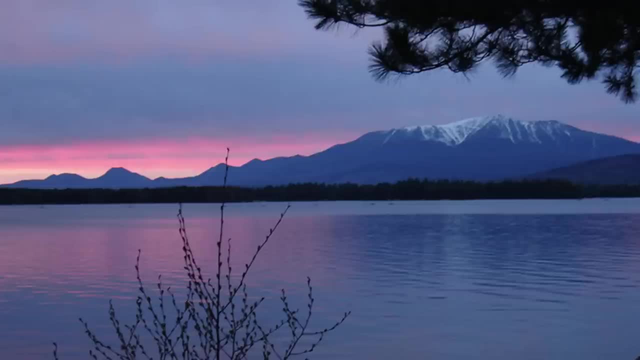 Springer Mountain in Georgia. That is the highest point in the state and marks the end of the famous Passing through 14 different states along the way. Katahdin's peak is in the significantly colder subarctic climate zone, a climate zone found in very few parts of the contiguous US. 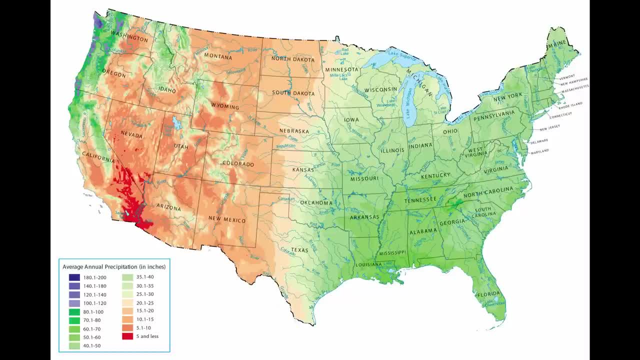 Maine receives, on average, 45.49 inches of precipitation per year, pretty much on par with the part of the country it's in. The state's rainfall is pretty consistent across its regions and it's the 17th rainiest state in the country. 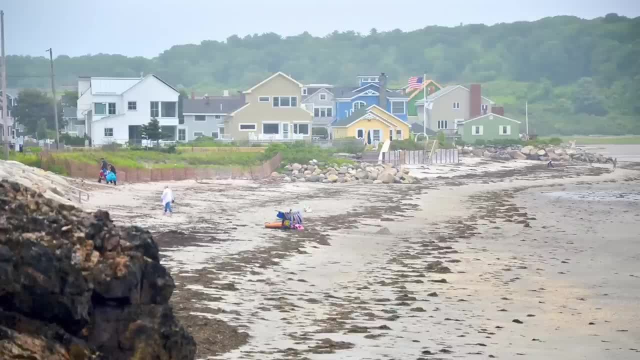 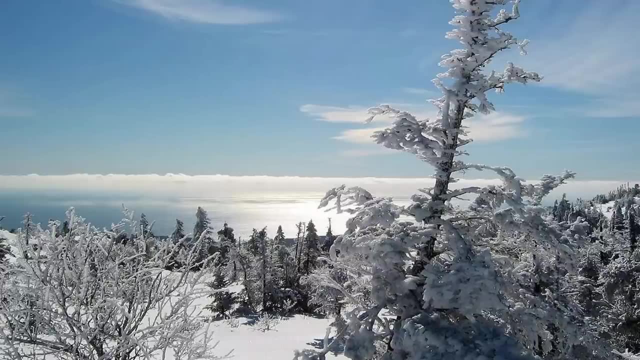 On top of that, it has the second lowest average annual sunlight of any state in the lower 48, only Washington gets less sun than Maine, And with an average temperature of 43 degrees Fahrenheit it's the country's fourth coldest state on average, surpassed by only Alaska. 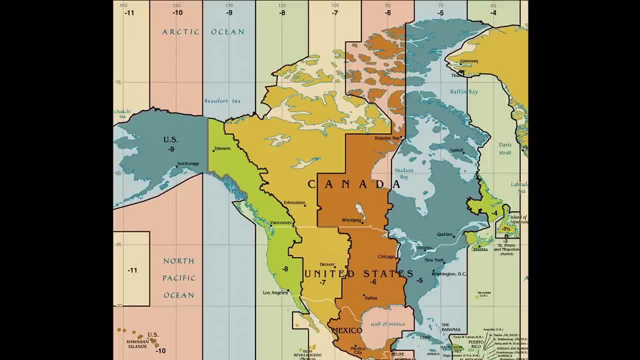 North Dakota and Minnesota. The entire state is located in the eastern time zone, but the neighboring Canadian province of New Brunswick is an hour ahead in Atlantic time. Maine and New Brunswick have a lot of border communities, especially along the St Johns. River in the north, so I'm sure that can be a bit of a hassle. The state is even considered switching to a lot of border communities, especially along the St Johns River in the north, so I'm sure that can be a bit of a hassle. The state is even considered switching to a 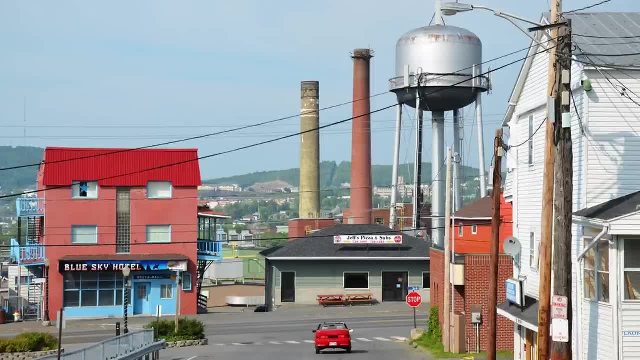 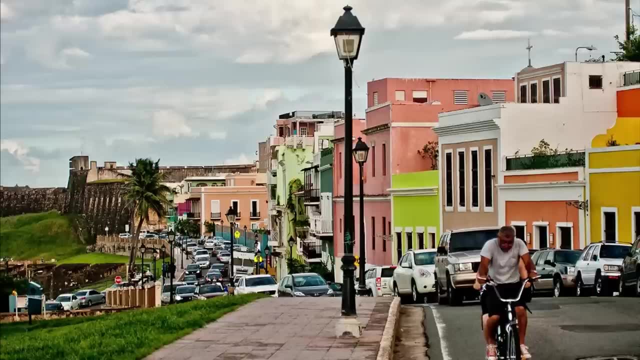 Atlantic time in the past, Though, by their location across the international dateline, Guam and the Northern Marianas see the start of the new day first, and by direction of travel, Puerto Rico and the Virgin Islands are further east. Maine is the easternmost point in the 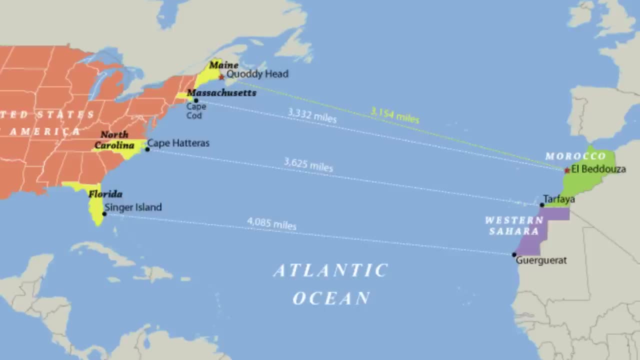 contiguous US so far east that, interestingly, despite being significantly further to the north, it's actually the closest point in the lower 48 to the continent of Africa, as well as, unsurprisingly, to Europe, though each of these points are in different parts of the. state. The honor of the contiguous US's easternmost point goes to Sail Rock, a tiny rock just off the coast of West Quadi Head, a point guarding the entrance of Passamaquoddy Bay near the town of Lubeck. 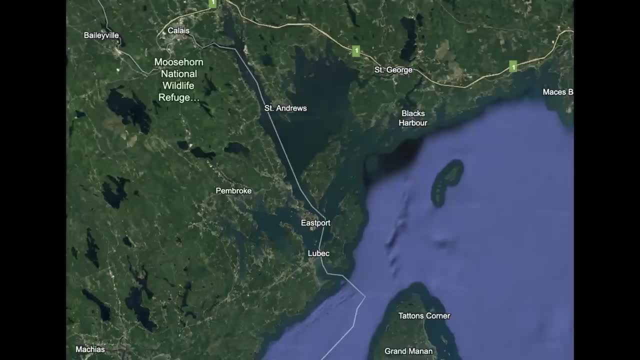 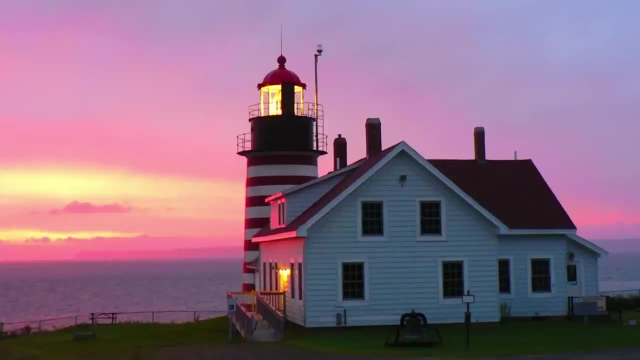 and the mainland of the country's easternmost point. For a few weeks each year, the West Quadi Head Lighthouse is the site of the continental US's first sunrise For about half the year. that spot is Mars Hill, the hill in northern Maine along the border with New Brunswick and most famously for the 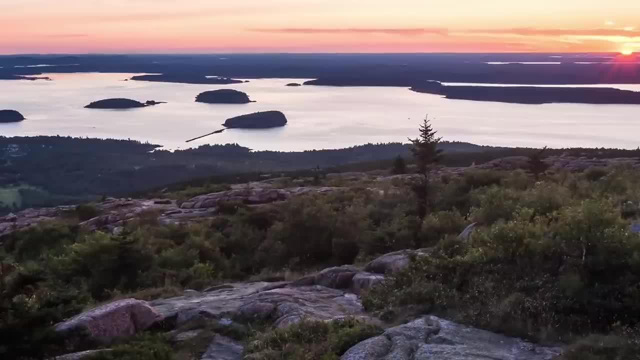 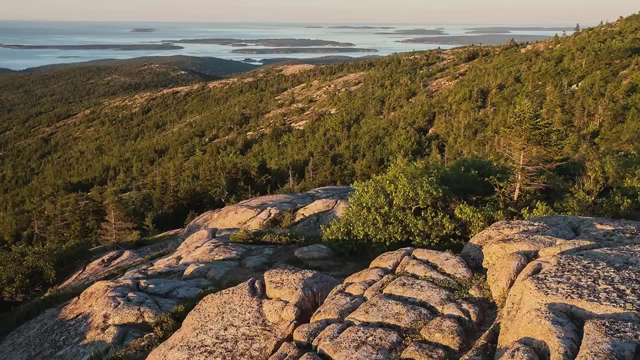 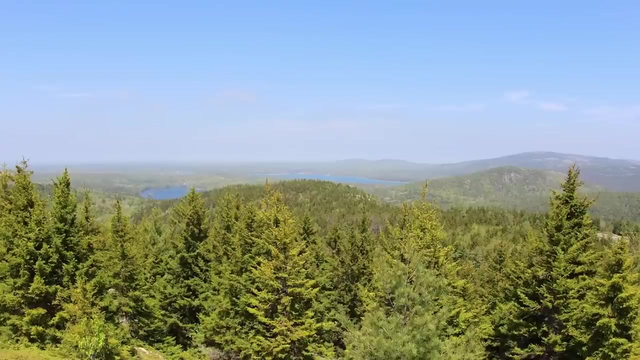 rest of the year. the first sunrise is at Cadillac Mountain, a peak on Maine's Mount Desert Island in Acadia National Park. that, at 1,530 feet or 466 meters, is by far the highest coastal point on the Atlantic coast of the lower 48. Maine is nicknamed the Pine Tree State. it's filled with 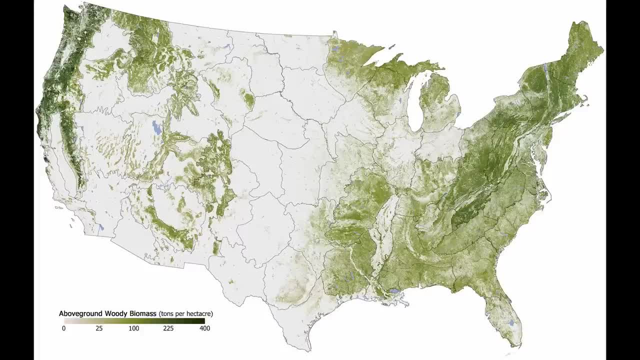 trees, including many pines, and in fact is the most forested state in the entire country, With over 89 percent of the entire state covered in trees. no state or territory surpasses it. Forest takes up nearly all of the state, the one major exception being the agricultural potato. 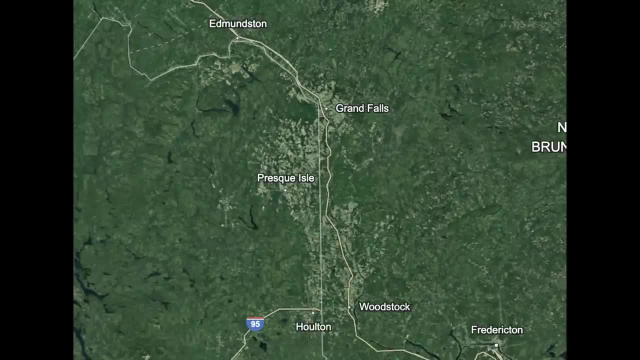 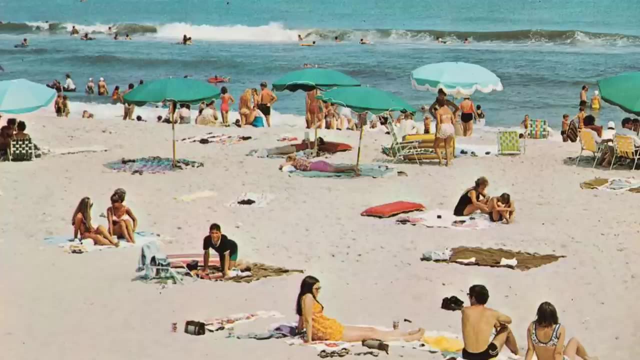 growing part of Aroostook County along the Canadian border. You'll also hear Maine referred to as Vacationland. The state actually ranks pretty low as the country goes in terms of tourism numbers at 44th out of the 50 states in DC. but this stat alone can be pretty misleading. 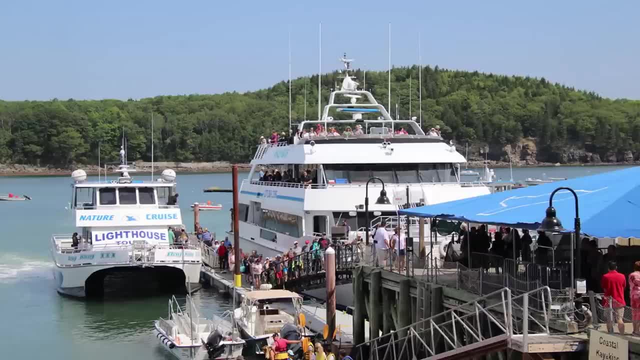 First off, the 15 million people recorded as visiting Maine each year is still huge in comparison to the state's roughly 1 million residents. On top of that, the state's population is pretty low and tourism numbers are pretty hard to track. in general, The best tourism agencies. 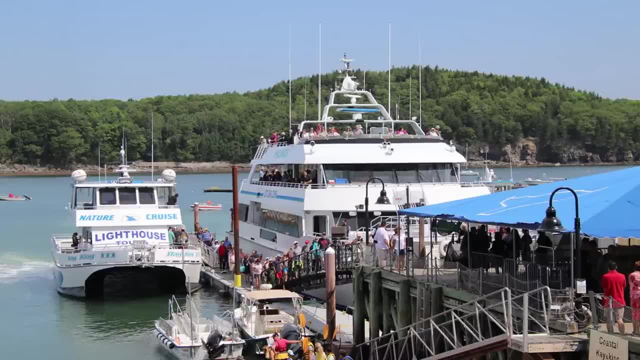 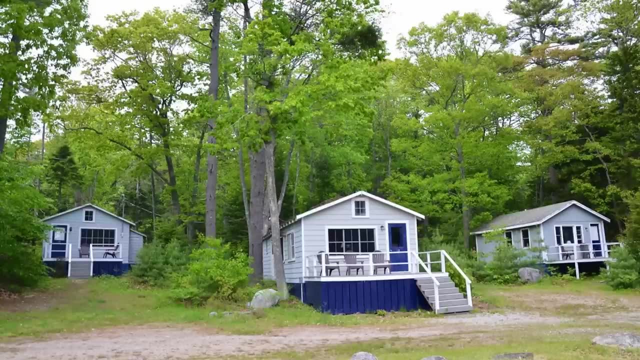 can usually do is look at hotel and other lodging reservations, But in Maine this overlooks a major element of local tourism that has a huge impact on the state. second homes: Maine has the highest proportion of vacation homes in the entire country: 19 percent, or nearly a fifth of all houses in the. 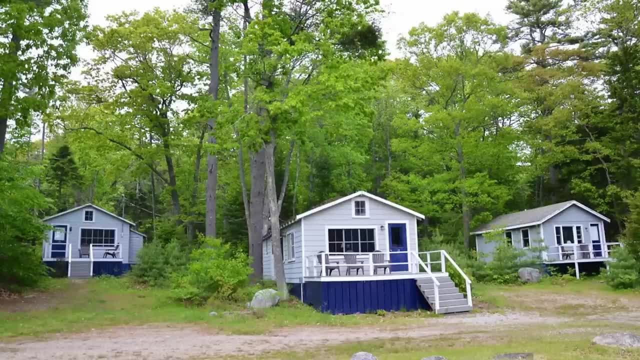 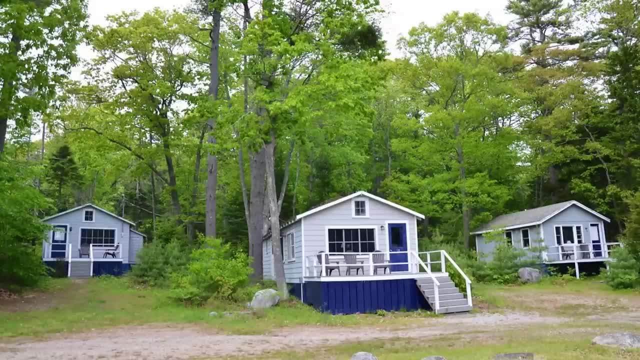 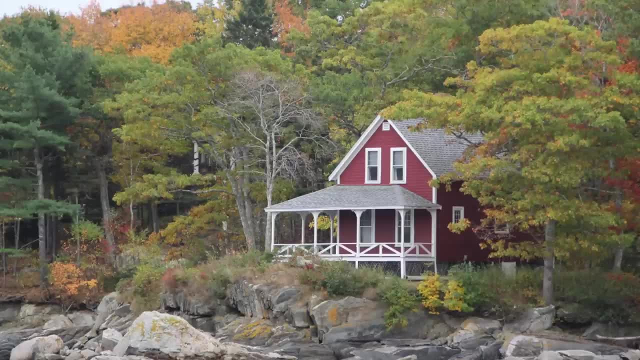 they might even consider themselves more part-time residents than tourists, though i'm sure many locals might disagree. but as they typically visit more frequently and stay for longer periods of time, they have far greater economic impacts on the state and the towns they stay in than tourists who might just visit for the weekend and have a significant cultural impact on the state. Second homes are often owned by people from major cities like Boston and New York looking for a rural getaway, as the state and its beautiful scenery are fairly close to both cities, with Boston in particular only about an hour and a half away, But a large number as well are owned by people from Portland, Maine's. largest city. On top of that, Maine is a popular tourist destination for Canadians as well. Major Canadian cities like Montreal and Quebec City are fairly close to the state, and tourists from Quebec have been vacationing in Maine beaches like Old Orchard Beach, some of the closest beaches for most residents. 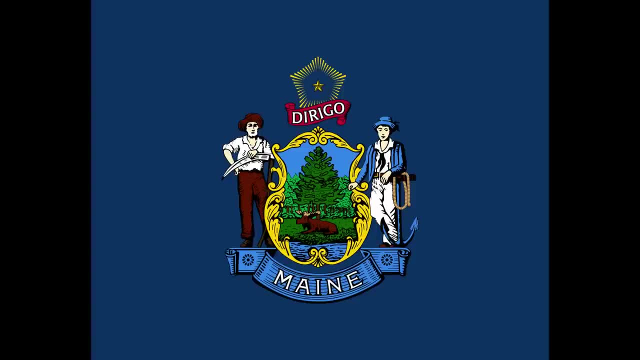 of the province for generations. Maine's flag shows the state seal on a blue background. It's not a bad seal. it shows a moose and a pine tree flanked by a farmer and a sailor, as well as Maine's name and its motto, Derigo- Latin for I direct. but 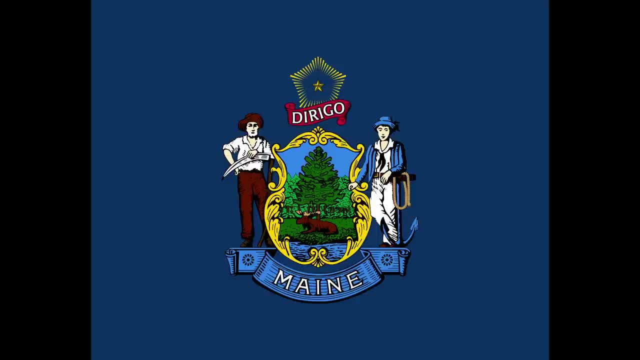 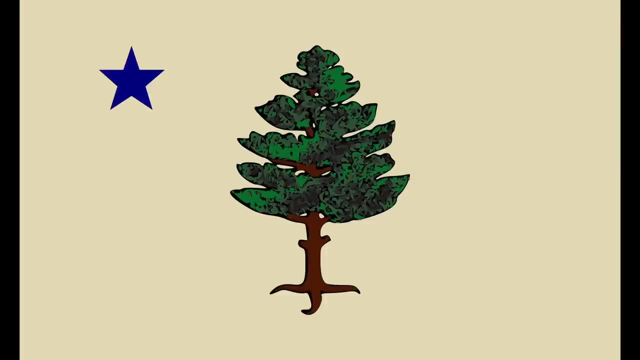 it's difficult to distinguish from the countless other state seal on blue background state flag designs. The state's former flag, which shows a pine tree and blue star on a beige background, is, in my opinion, a much better design. It's pretty popular among Mainers. you'll see it on bumper. 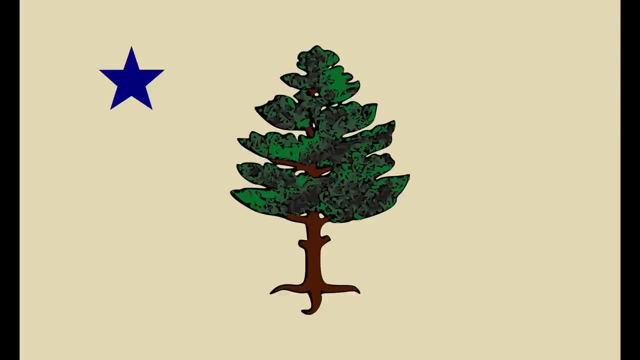 stickers and clothing designs, and people frequently fly it. There's been a push to make it the state flag once again and after it was approved by the state house, the governor decided to put it up for referendum. so the people of Maine will. 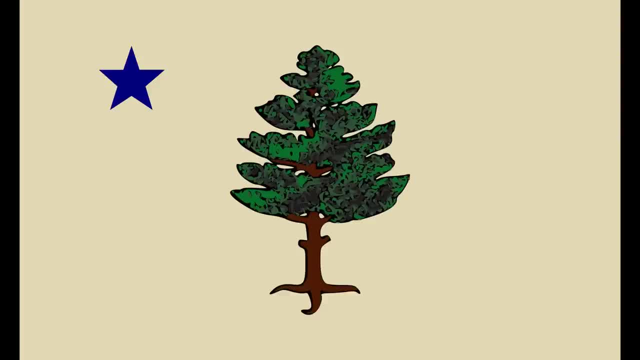 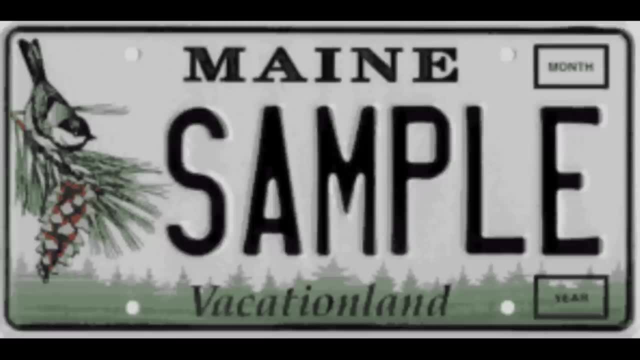 vote on whether or not to adopt it in November of 2024.. The state's license plate shows a chickadee sitting on a pine branch, a forest, and the words Maine and vacation land. Maine is one of just a few states where the origin of its name is unclear. 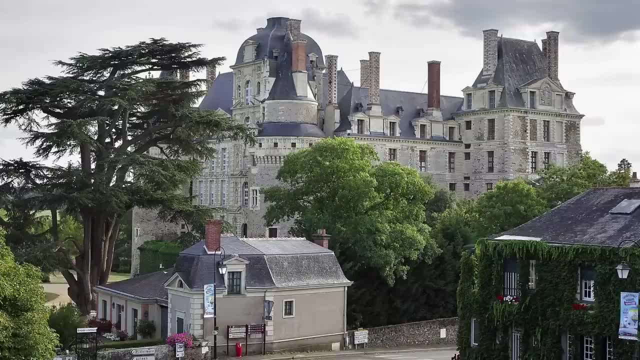 One theory is that it takes its name from Maine, one of the old provinces of France which was supposedly home to property of Henrietta Maria, the French-born British queen. The state has a strong French history, so this would make sense At the same time, Ferdinando. 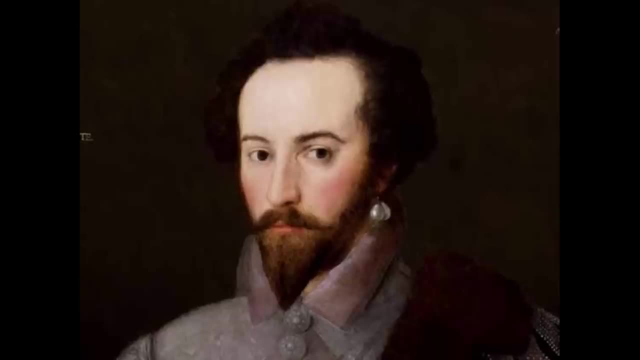 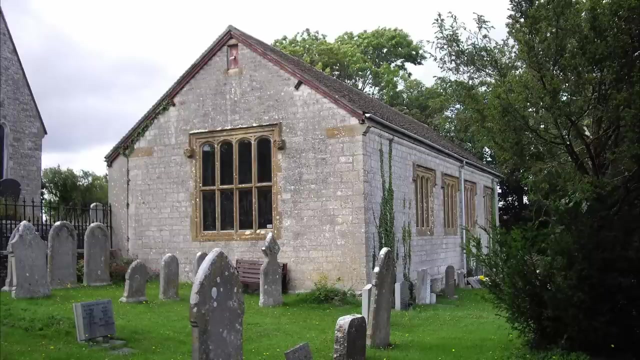 Gorges, who received the colonial charter for what would become the province of Maine, was from a family with a property in the English town of Broadmain, making it a possible contender for the origin of the state's name. The most common theory, though, is that fishermen off. the region's island-dotted coasts are considered to have lived in Maine for many, many years. The most common theory, though, is that fishermen off the region's island-dotted coasts are considered to have lived in Maine for many, many years. The most common theory, though, is that fishermen off the region's island-dotted coasts are considered to have lived in Maine for many, many years. The most common theory, though, is that fishermen off the region's island-dotted coasts referred to the land that wasn't an island as the Mainland, or simply the Main. This was. once a fairly common synonym for mainland. The mainland colonies of Spain, for example, were often called the Spanish Maine. All of these theories are pretty plausible, so it's pretty difficult to tell which is the true origin of the name If you're from Maine. 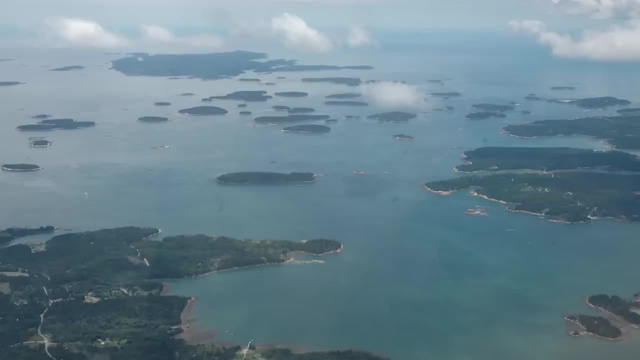 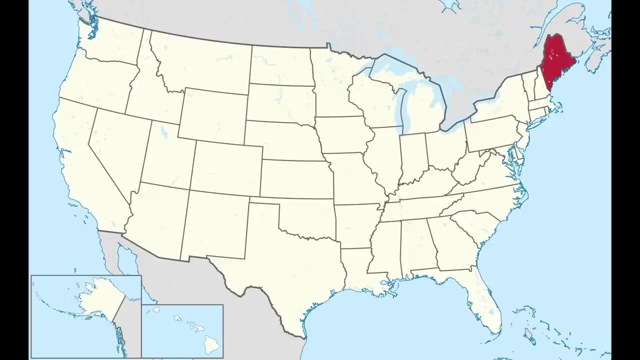 I'm curious as to what you think. Leave a comment and let me know where you stand on the name origin. As states go, Maine is fairly small. With a land area of 30,843 square miles, or or 79,883 square kilometers, Maine ranks 39th out of the 50 states in land area or in other. 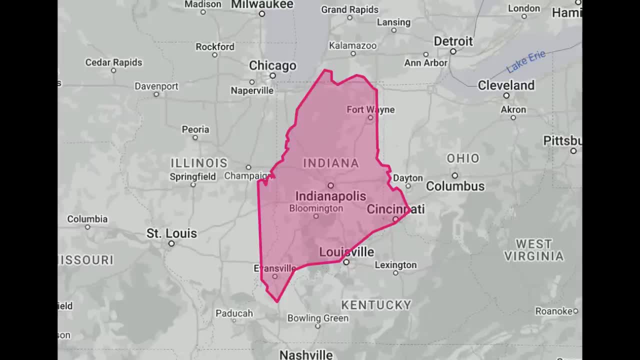 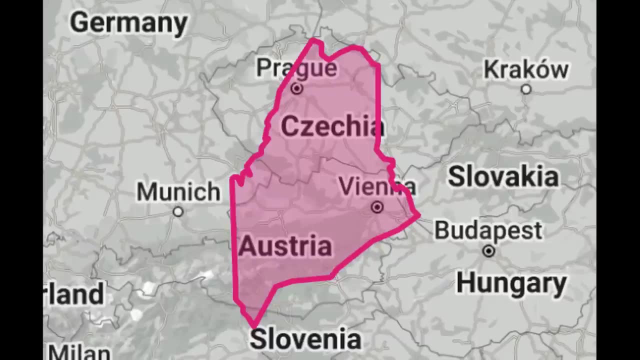 words is the 12th smallest state in the country, Smaller than Indiana but larger than South Carolina. It's similar in size to countries like Austria or Czechia. At the same time, compared to many of its neighbors, Maine is actually quite large Out of the 17 states. 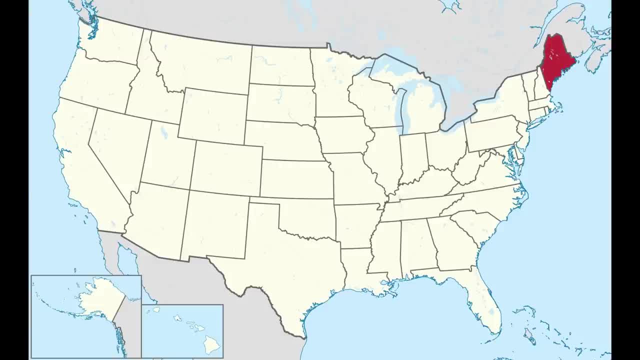 sitting on the eastern seaboard, not all of which are coastal. Maine is larger than 10 of them and smaller than six. In the northeastern US, it's the third largest state. Only New York and Pennsylvania are larger. It's larger, too, than neighboring New Brunswick, as well as the other. 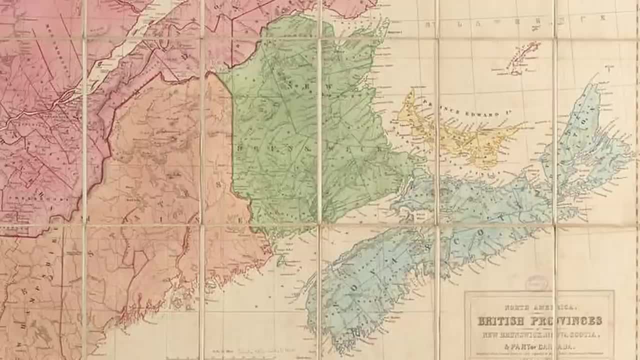 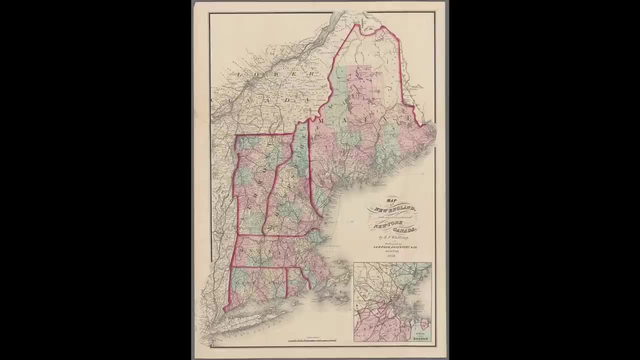 maritime provinces of Nova Scotia and Prince Edward Island, all three of which Maine shares some close cultural similarities with, Perhaps most strikingly, the other five states of New England, New Hampshire, Vermont, Massachusetts, Rhode Island and Connecticut are collectively only slightly larger than Maine. 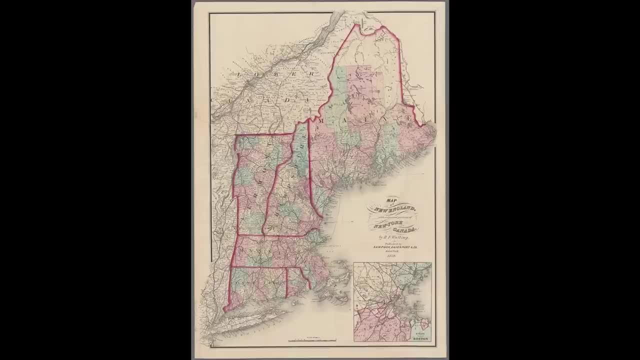 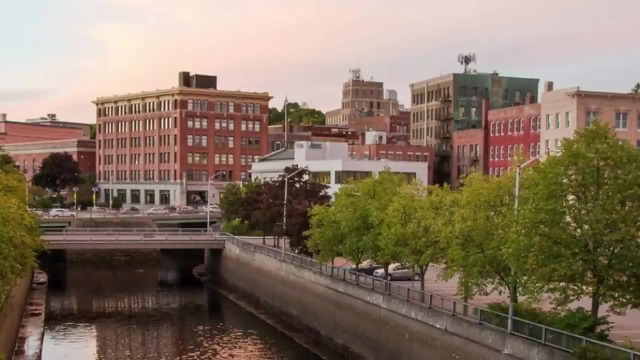 The Pine Tree State alone takes up 49.2% of New England's total land area- nearly half of the entire region. In terms of population, Maine is among the smallest in the country as well. It's home to only 1.39 million people, placing it at 42nd out of the 50 states. with fewer people than neighboring New Hampshire but more than Montana, a similar population to Estonia or Trinidad and Tobago. It's one of a number of states with a smaller population than the US and it's a small state. It's a small state but it's. home to the US territory of Puerto Rico, which in fact has a population more than twice the size of Maine. There are 34 different urban areas in the country, cities and their suburbs with larger populations than Maine, all the way down to Kansas City, Columbus and the Hampton Roads. area of Virginia. Only eight states- Montana, Rhode Island, Delaware, South Dakota, North Dakota, Alaska, Vermont and Wyoming- are home to fewer people than it. Out of the New England states, only the significantly smaller Vermont has fewer people than it. 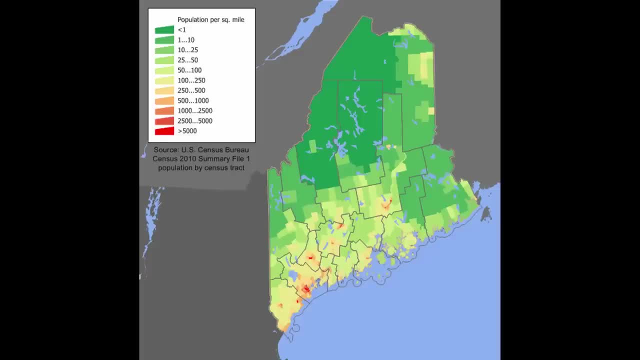 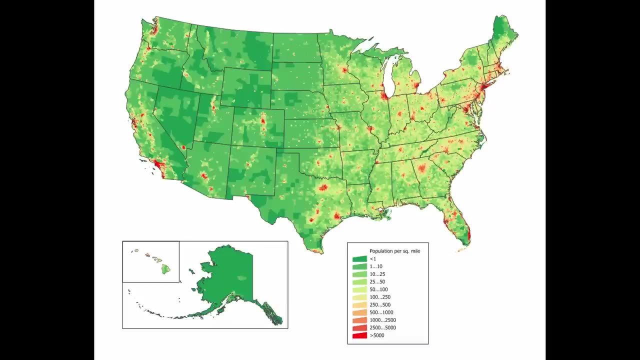 Taking up a small, but not too small, land area, while having a very small population. Maine has one of the lowest population densities in the country as well, with its 44.2 people per square mile or 17.1 per square kilometer, placing it at 38th out of the 50. 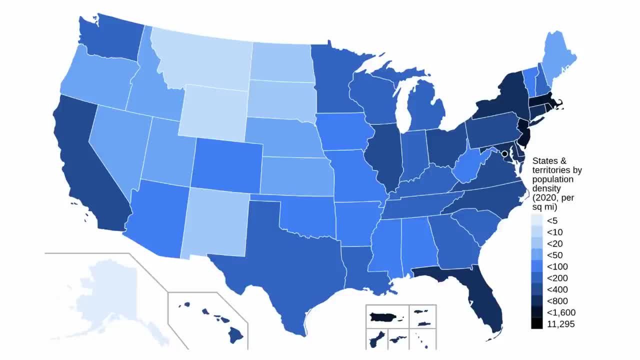 states. All the states with a lower population density are huge western and Greek plain states. the one sitting furthest to the east is Kansas. This gives Maine not only the lowest population density on the east coast but in the entire eastern half of the country Not a single state. 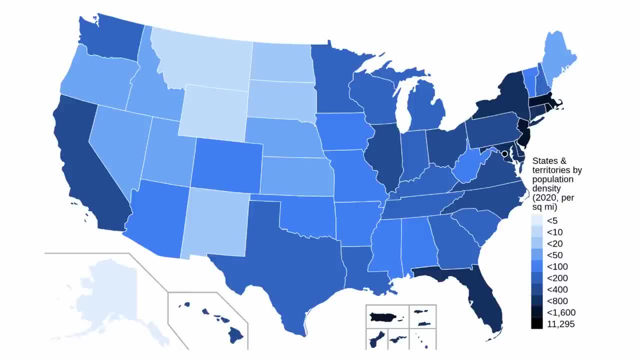 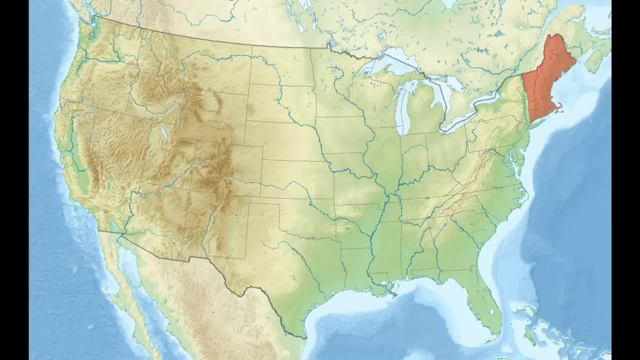 east of the Mississippi, or in fact fully east of the Missouri River, is as sparsely populated as Maine. It's located at the very northeastern tip of the United States, in the region known as New England, when with New Hampshire to its west, it borders only one other state, fewer than any other. 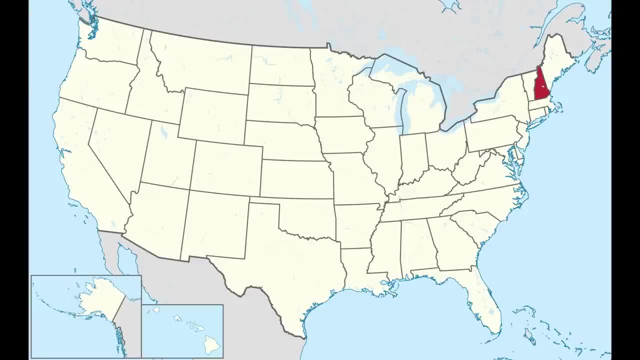 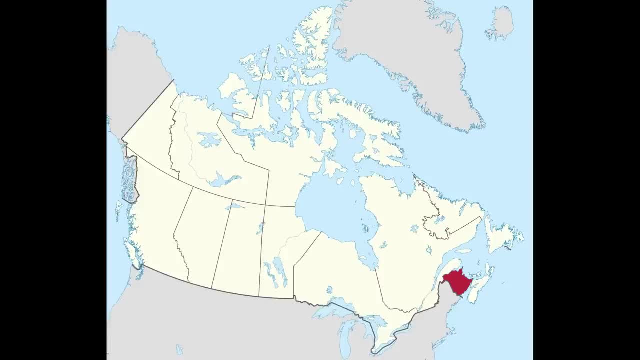 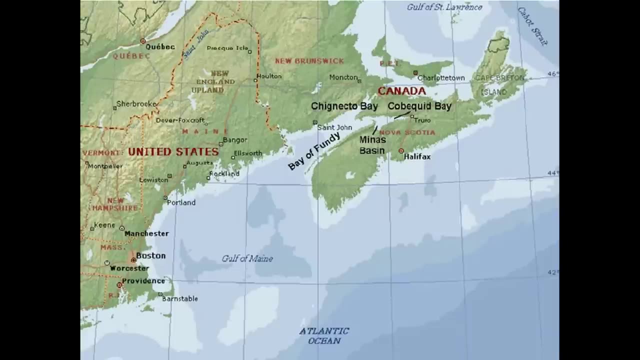 state in the lower 48, or any other state that has a border with other states at all: The Canadian province of New Brunswick. to its east, The Atlantic Ocean, specifically the Bay of Fundy in the Gulf of Maine, the enormous body of water between Nova Scotia and Cape Cod, sits to its 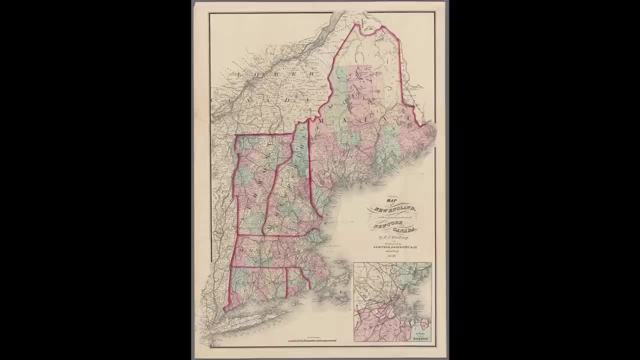 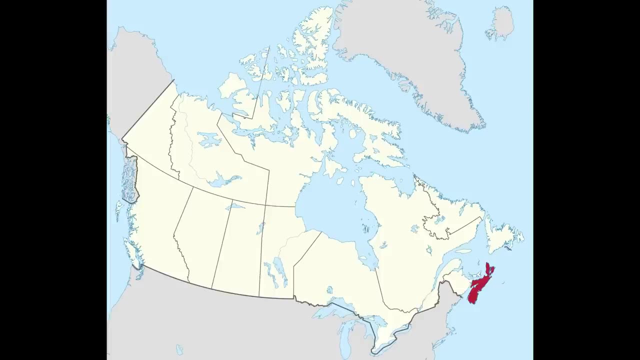 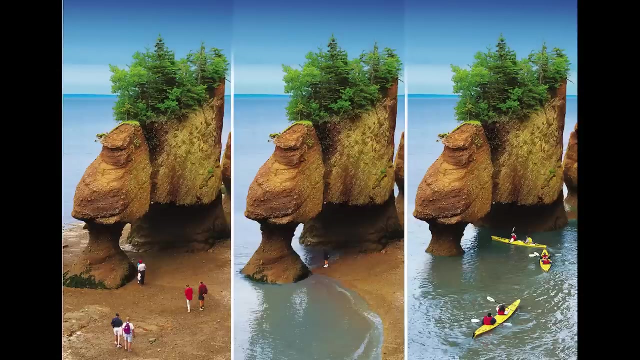 southeast. On top of that, states like Massachusetts and Vermont are close by, and the Canadian province of Nova Scotia is only about 48 miles, or 78 kilometers, across the Bay of Fundy. The Bay has one of the largest high tides in the world. From low tide to high tide, the waters of the Bay is 50 feet and at low tide large swaths of land that were once underwater are opened up. Maine's border with New Hampshire began to the mouth of the Piscataqua River in the Gulf of Maine and continues as a water border through the Isles of Shoals, a small offshore archipelago split. 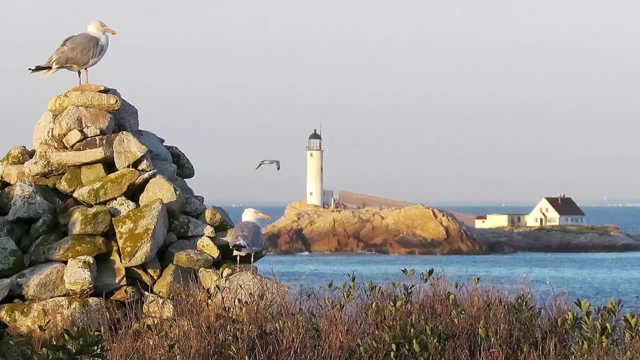 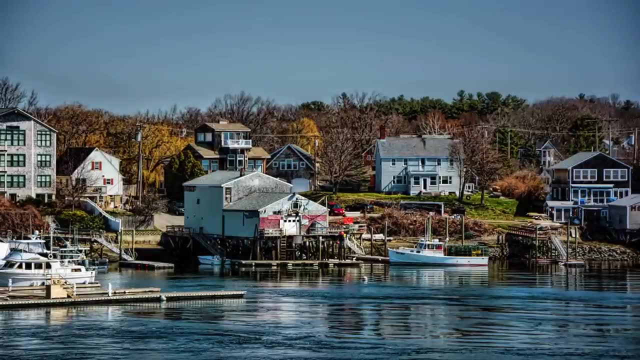 between the two states and home to the Shoals Marine Lab. At the mouth of the Piscataqua sits New Hampshire's third largest urban area, Portsmouth, and the main town of Kittery is right across from its city center. Interestingly, the Portsmouth Naval Shipyard. the oldest naval shipyard in the country isn't actually in Portsmouth but in Kittery, sitting on an island in the middle of the river that belongs to Maine, Following the Piscataqua in one of its tributaries, the Salmon Falls River, to its headquarters in a 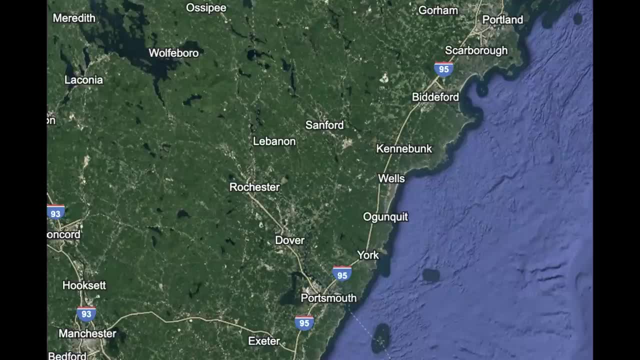 small lake called Horn Pond. the area around the border is a relatively populated part of both states, with larger New Hampshire towns like Rochester and Dover, not far from border towns in Maine such as Berwick. From Horn Pond the border follows a straight line roughly north for 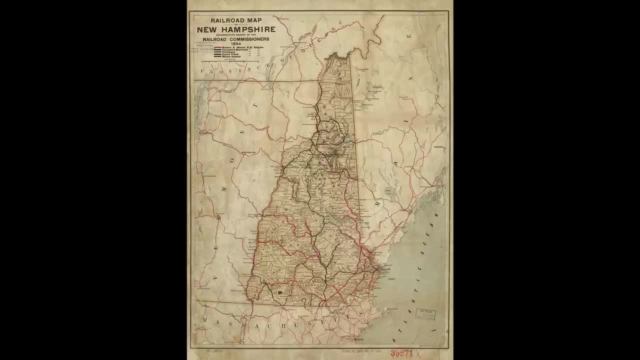 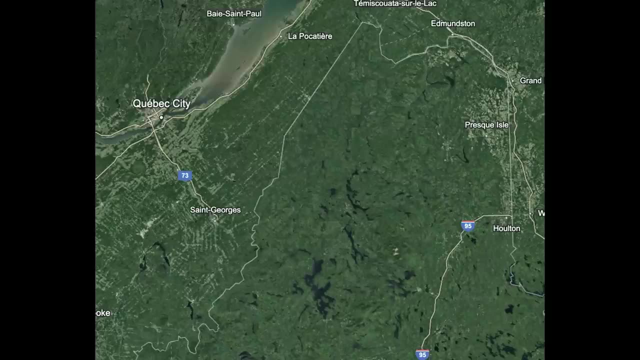 193 kilometers to the northern ridges of the Appalachians, where it becomes an international border with the Canadian province of Quebec, weaving northeast along the mountaintops and continuing down in the flat valleys and rolling hills of the other side, eventually following a. 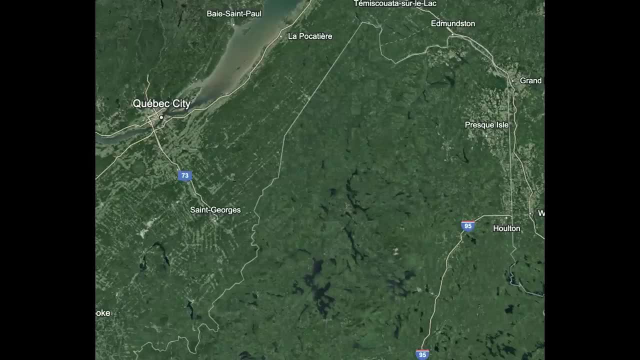 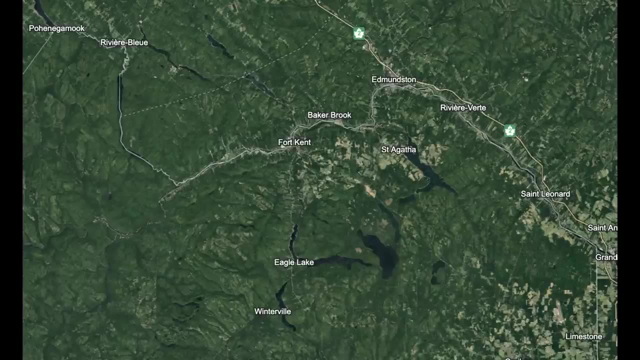 series of diagonal lines to the St Francis River, at the town of Escort, across from the Quebec town of Ponagamook. The border follows the river as it weaves to the southeast and at a point along the St Francis it changes from a border with Quebec to a border with the United States. The border is: 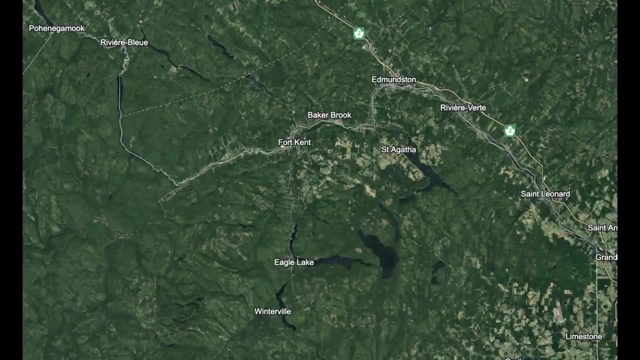 connected to a border with New Brunswick. The St Francis then flows into the St John River, which the border follows all the way to the town of Hamelin. The area around the river is where most of northern Maine's population lives, mostly in cross-border river towns: The town of Mattawaska. 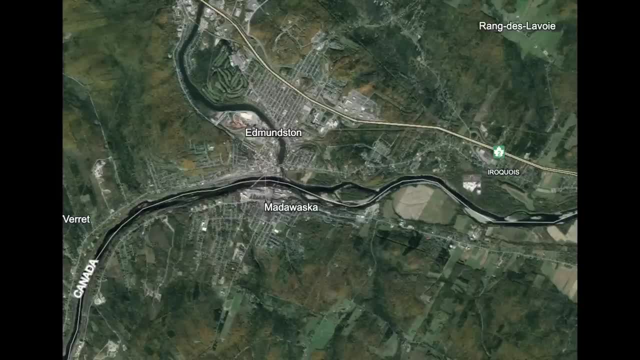 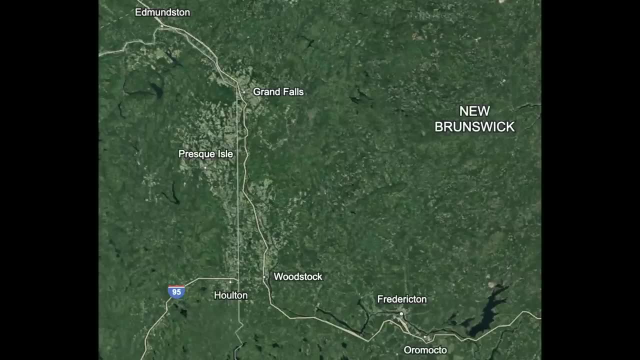 for example, sits right across from Edmonston, New Brunswick's sixth largest urban area. From Hamelin, Maine's border with New Brunswick continues south for 77 miles, or 124 kilometers, until it reaches a stream called Monumental Brook. 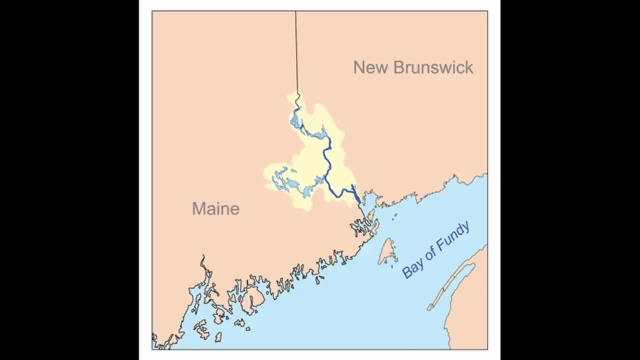 which it follows along the border with New Brunswick. The river then flows as it turns into the St Croix River, following the river's winding course through lakes and forests and passing through the town of Callas, the Canadian town of St Stephen. 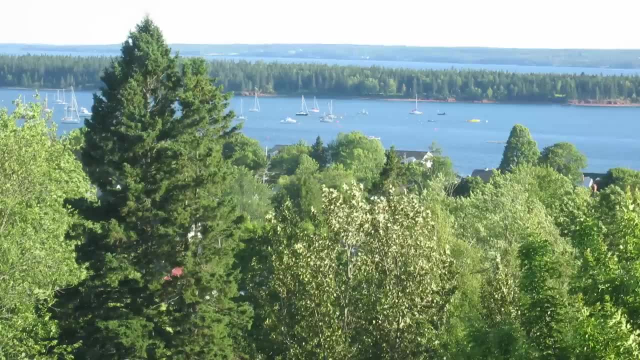 New Brunswick. on the other side, The river widens into Passamaquoddy Bay, emptying into the Bay of Fundy and there, at West Quoddy Head, the US-Canada border, the longest land border on. 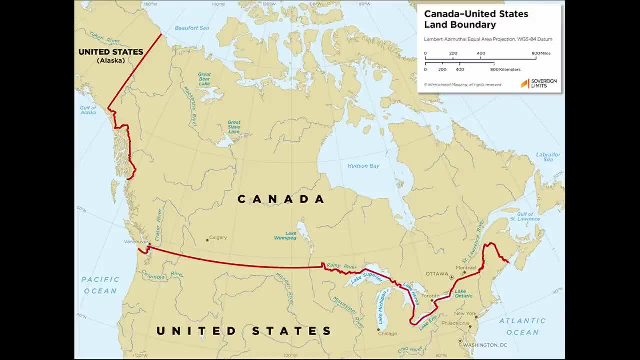 Earth reaches its eastern end. having stretched nearly 4,000 miles from Point Roberts Washington in the west, The bay, filled with islands and lined by peninsulas, is home to the St Francis Bay, which is home to the towns of Eastport and Lubeck, which sit just across the water. 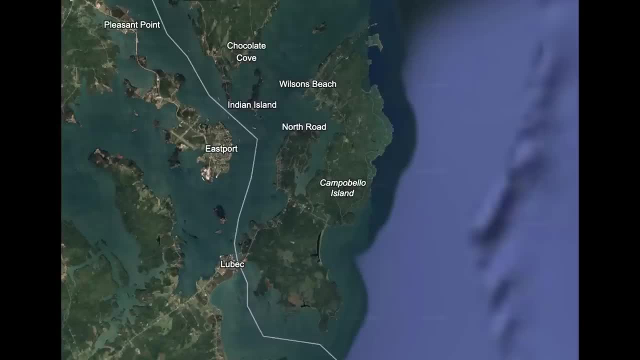 from Canada's Campobello Island, Franklin Delano Roosevelt's vacation home, and a community cut off by land from the rest of Canada. Canadians living there must cross an international border to leave. as the only bridge goes to Maine, It's proved a major logistical challenge for 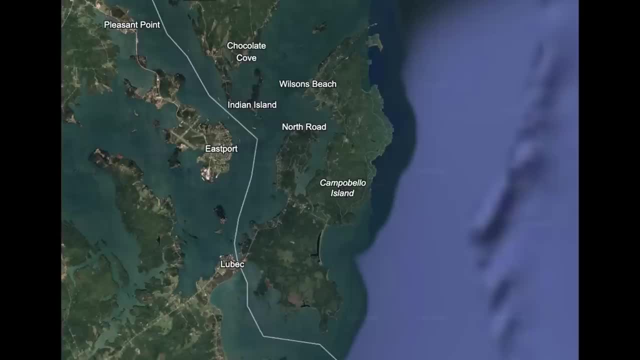 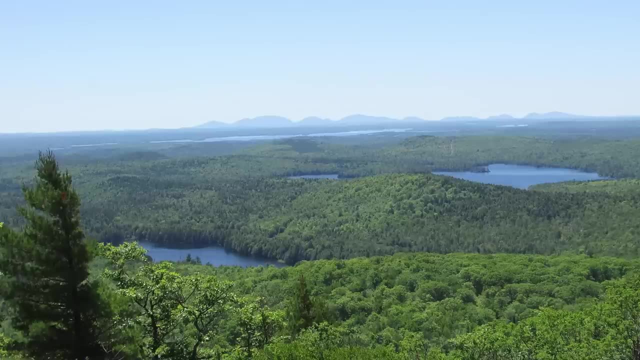 locals, and there have even been proposals to sell it to the United States or even trade it, for the similarly isolated Washington town of Point Roberts, Maine is dominated by a rugged landscape. Most all of the state is covered in rolling hills and mountains. Though 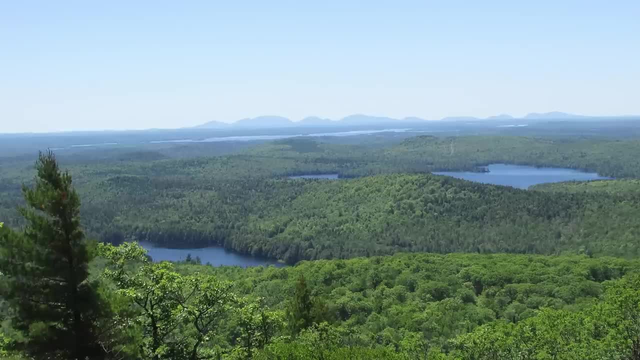 they're smaller closer to the coast. the state lies beyond the northern edge of the coastal plain that stretches across most of the east coast, and this leaves consistently little flat land. It's the only east coast state where mountains dive right into the ocean. something. you'd usually have to go to west coast states like California, Oregon, Washington, Alaska or Hawaii to find The higher peaks of the Appalachians, though cut northeast from New Hampshire into New Brunswick and Quebec. The more you travel west, the more. 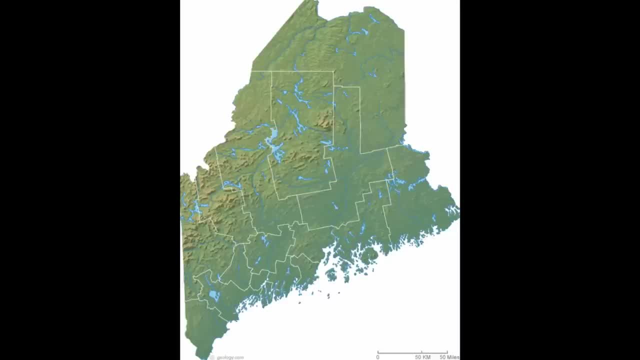 you'll see the south coast and the more you'll see North Carolina, which is the easternmost, and are at their highest in the state, from Mount Katahdin, the endpoint of the Appalachian Trail, to the New Hampshire border. Because of this, most of Maine's major rivers originate in this. 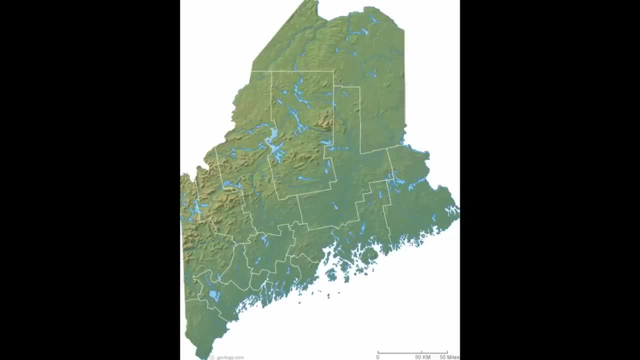 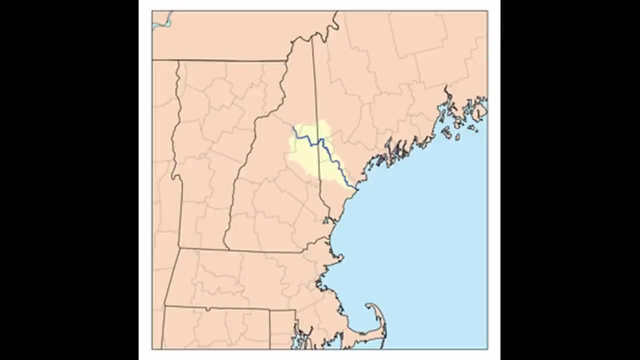 highly elevated northern and west-central part of the state and typically flow north to south. It's home to six major rivers, many of which are quite large. The Saco flows in from the White Mountains of New Hampshire and flows into the Atlantic near Biddeford, Most of western Maine. 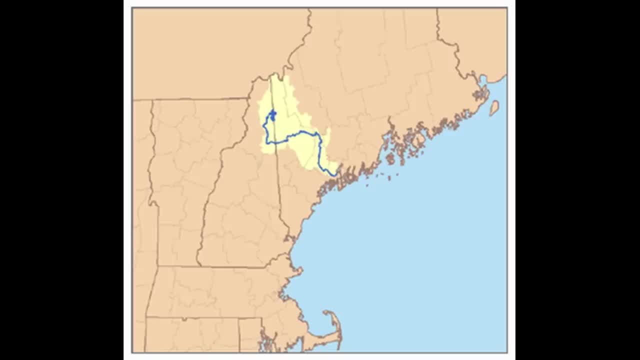 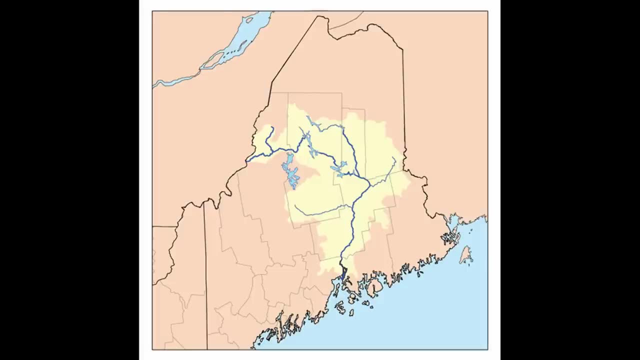 is in the watersheds of the Kennebec and the Androscoggin, which flows into the Kennebec and together into the Atlantic. near the town of Bath, Much of the central part of the state is in the watershed of the Penobscot River, which empties into the huge, island-filled Penobscot Bay. 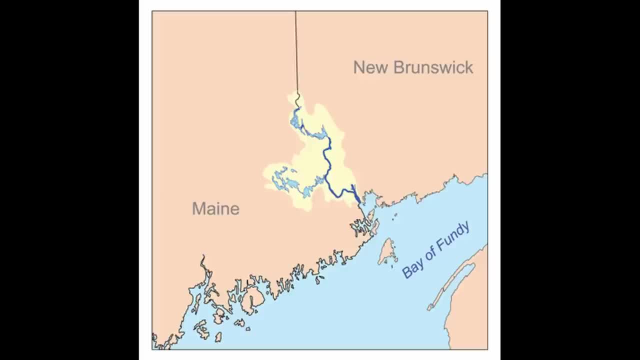 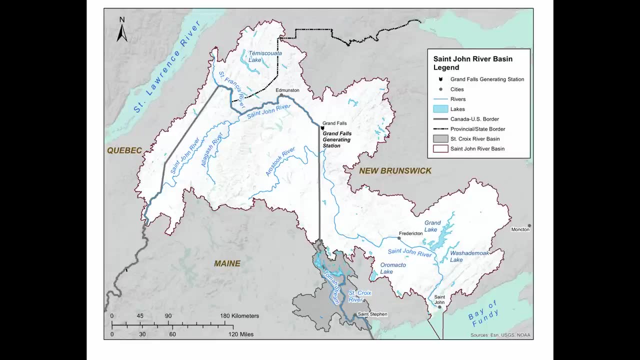 the largest bay in the state south of Bangor. In the east, the St Croix forms much of the border with New Brunswick, but the longest river in the state, though not the longest fully within it, is the St John. The river begins in the state and- a rare exception- flows south to north. 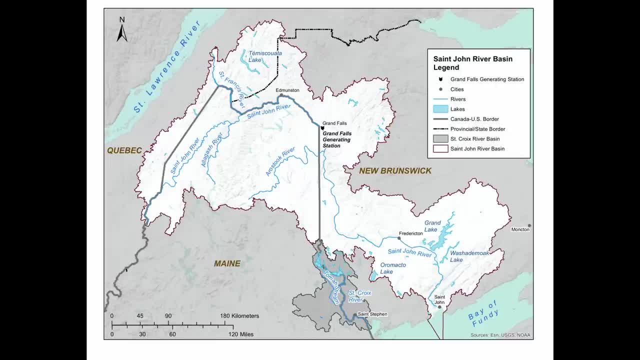 forming the Penobscot River. The Penobscot River is the longest river in the state, forms much of Maine's northern border, then enters New Brunswick and turns south, meeting the Bay of Fundy in the province's capital city of St John, Across the entirety. 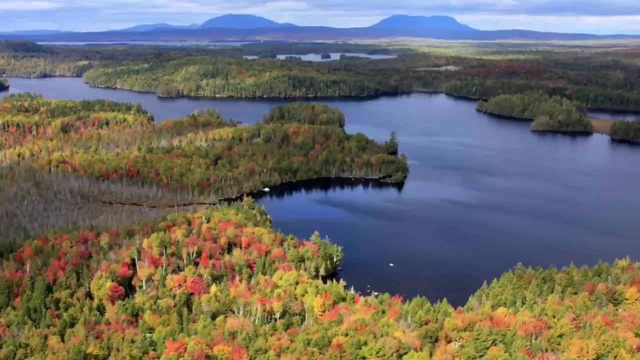 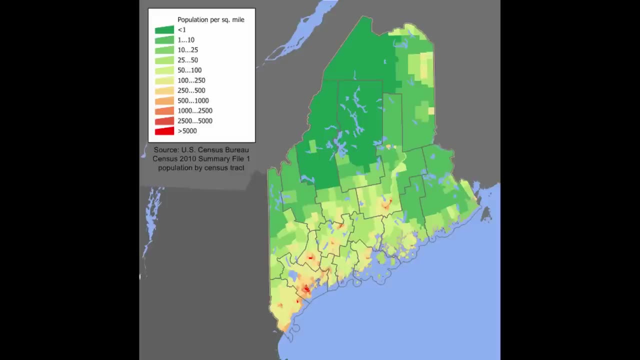 of the state you can find lakes, both large and small, and most of the landscape is heavily forested. Most of Maine's population is concentrated along its coast and in the flatter lands and river valleys reaching not too far inland. Around 80% of Maine's entire population lives in a relatively 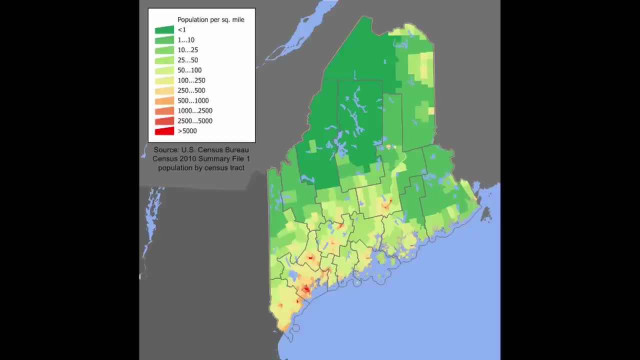 small section of the state, a corridor stretching from Kittery and the New Hampshire border northeast to Bangor and the coastal town of Bar Harbor. The coastal region along the New Hampshire border is sometimes referred to as the Maine Beaches and it pretty much encompasses York. County. York County is the second most populous county in the state, but its population is fairly spread out instead of centered in a single town. as it grows rapidly with development spreading in from New Hampshire and Massachusetts, This is the most visited part of the state, bringing in 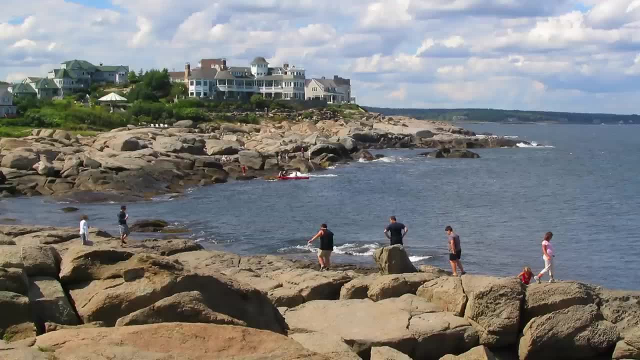 nearly a quarter of all tourists who come to Maine and is where many of the state's numerous vacation homes are located. The state's most visited part is the New Hampshire Beach, which is located in the middle of the state. It has, as its name suggests, the largest and some of the most popular 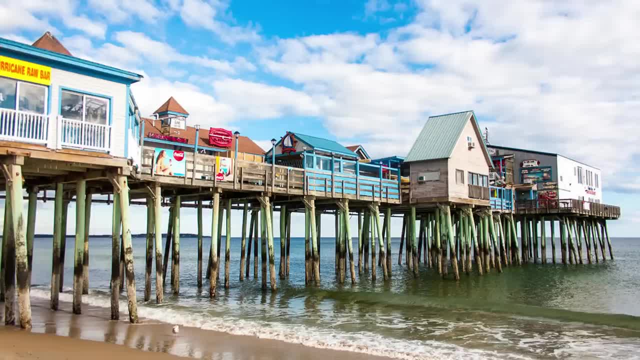 beaches in the state. Places like Argunquit and Old Orchard Beach are major destinations. It's the most touristy part of the coast. Here you'll see boardwalks, amusement parks, piers and beachfront condos, as opposed to the more remote fishing villages further along the coast. 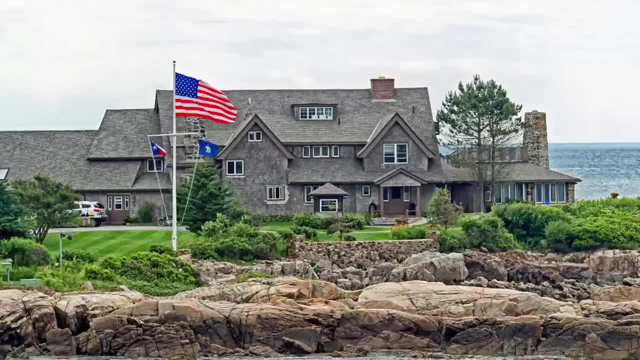 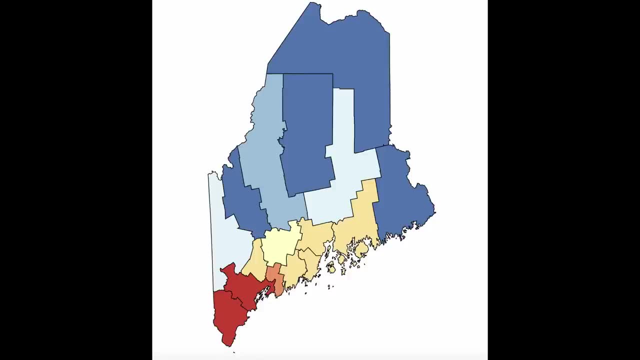 It has some high-profile visitors. The Bush family frequently vacations at their family compound in the wealthy beach town of Kennebunkport. While most of the Maine coast has seen its population grow, it's not the only beach town in Maine that has seen its population grow. It's also seen 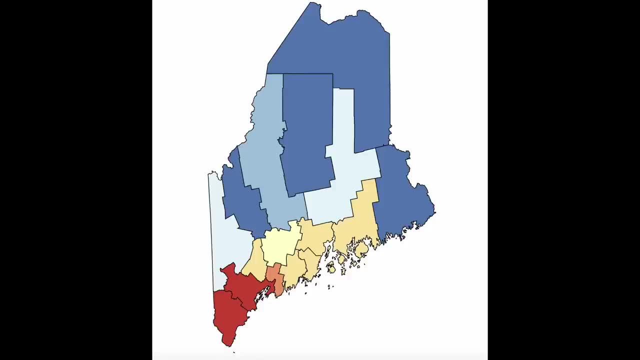 some high-profile visitors. The Bush family frequently vacations at their family compound in the wealthy beach town of Kennebunkport. While most of the Maine coast has seen its population grow, the Maine beaches, along with the Portland area, are by far the fastest growing parts of the state. 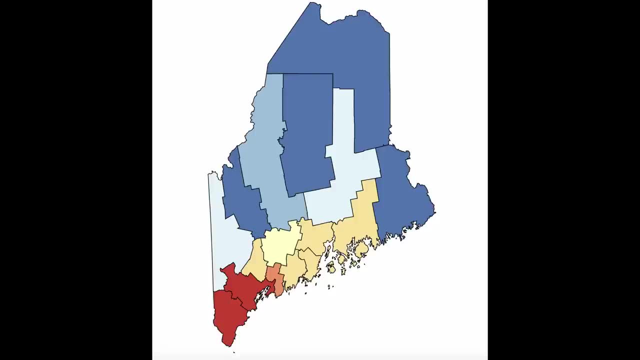 each seeing a near 10% increase in population since 2010.. The growth, wealth and heavy tourist presence is largely due to its location. Kittery is only about an hour and a half from Boston, making the Maine beaches the most easily accessible part of the. 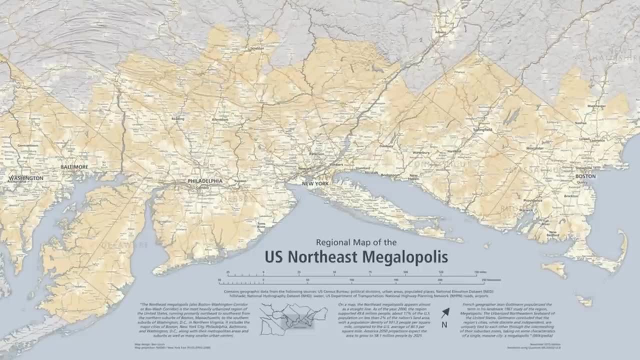 state to the huge population centers of the Northeast. The Northeast megalopolis, the strand of near-continuous urbanization stretching from Washington DC to Boston, or a 17% of the US population lives, is sometimes considered to stretch as far northeast as 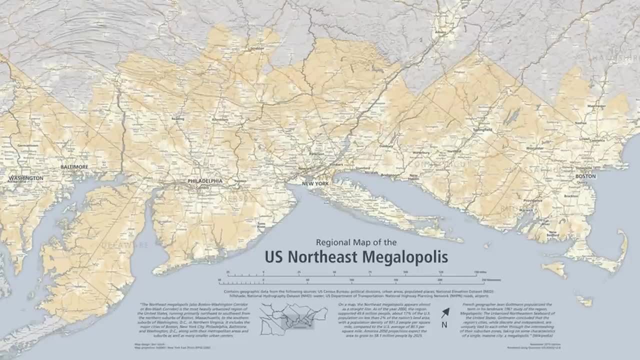 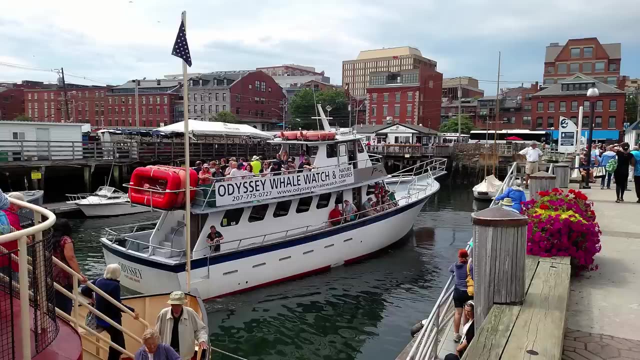 Portland, And as this part of the state continues to grow and urbanize, it's likely that this will become less and less a matter of debate. The fastest growing part of the state, though, is Portland, itself, Sitting on the western coast of Casco Bay. 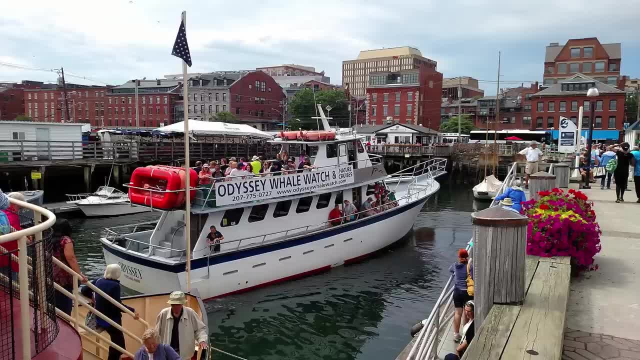 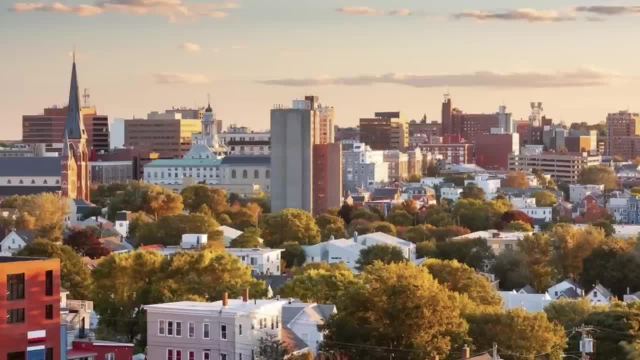 it's Maine's largest city and urban area, with around 205,000 people living in it and its suburbs. Though still a small city, it's by far the most populous and urbanized part of the state, an important part of the state's population, With Portland's urban area home to 15% of the state's entire. 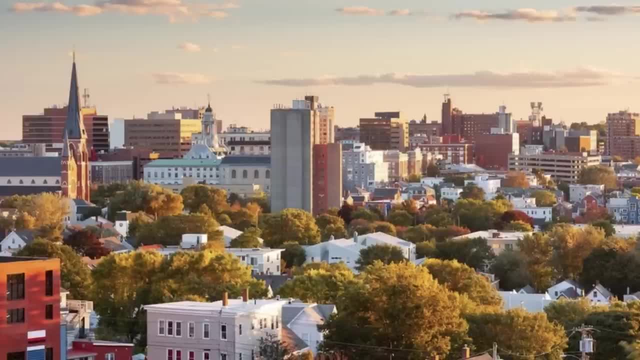 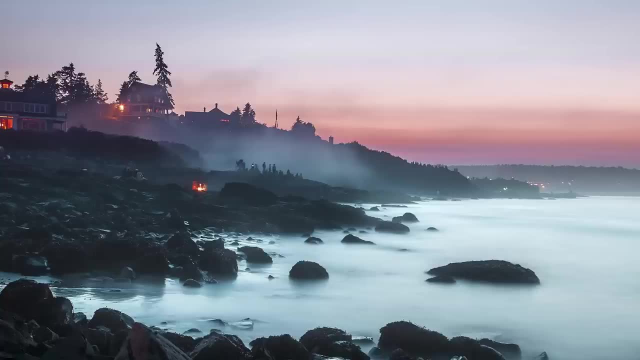 population, it exercises major influence within the rest of the state. Other towns, like Yarmouth, sit on Casco Bay, not far from the city. The mountainous, hilly and rugged topography of the state and lack of a coastal plain has given Maine a coastline that appears jagged and sharp. 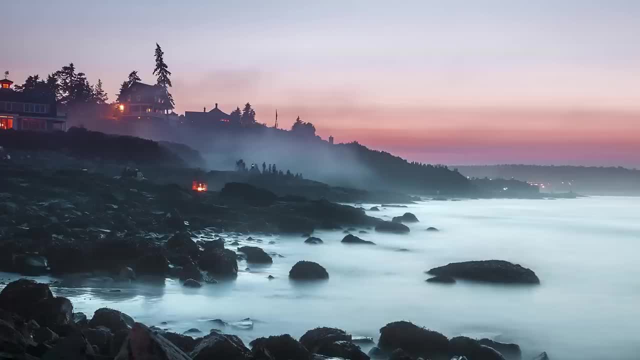 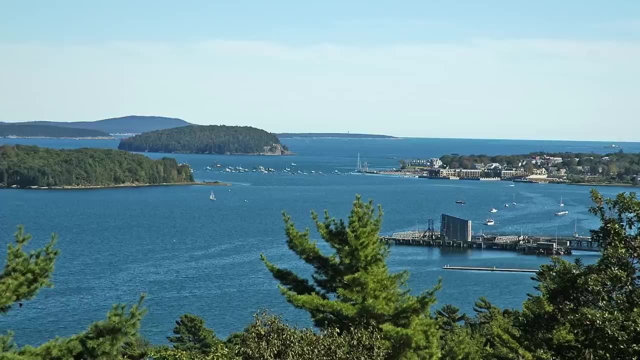 with long bays and inlets cutting deep into the state and thousands of rocky forested islands dotting the coast. Maine is estimated to have well over 4,000 islands, many coastal but many located in the state's numerous inland lakes. Only two other states in the country- Alaska and 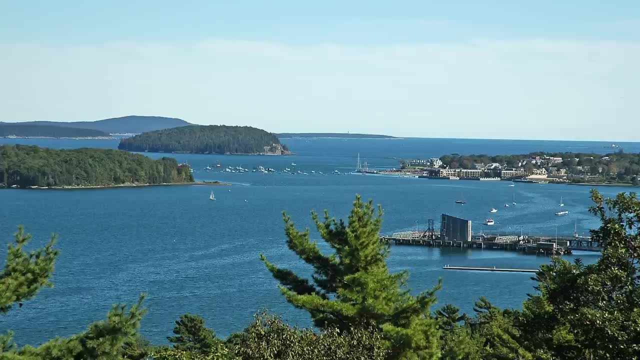 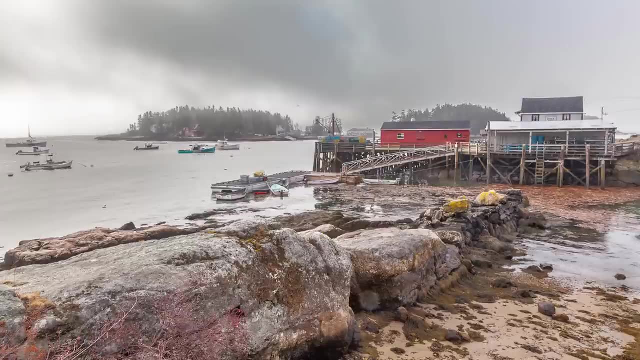 Florida, both of which are significantly larger, have more islands than Maine. These islands, many of which are home to small towns and fishing villages, in large part began at Casco Bay and continue up the entirety of the state's coastline, From Casco Bay to Penobscot Bay. 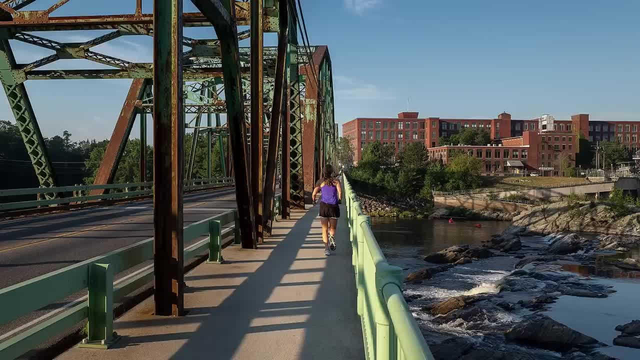 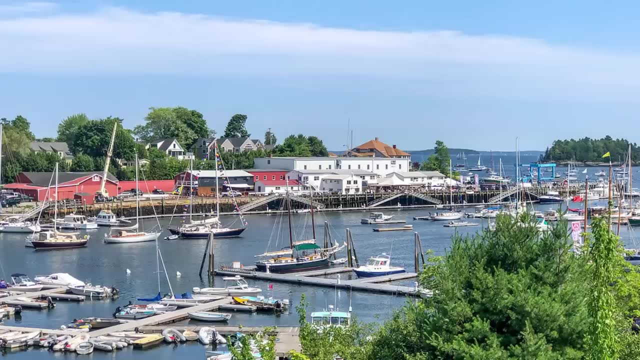 is a region known as the Mid-Coast, home to towns like Brunswick on the Androscoggin River and Bath on the Kennebec, not far away, as well as coastal towns on Penobscot Bay like Rockland, Camden and Belfast. 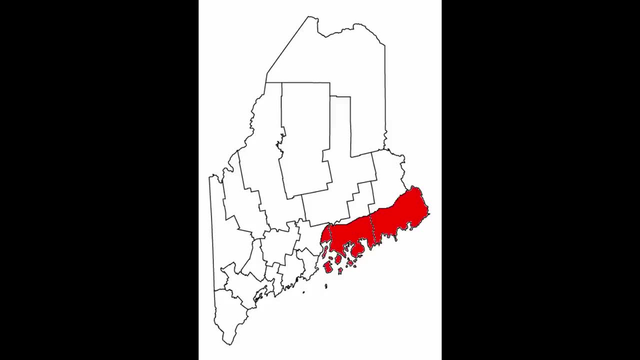 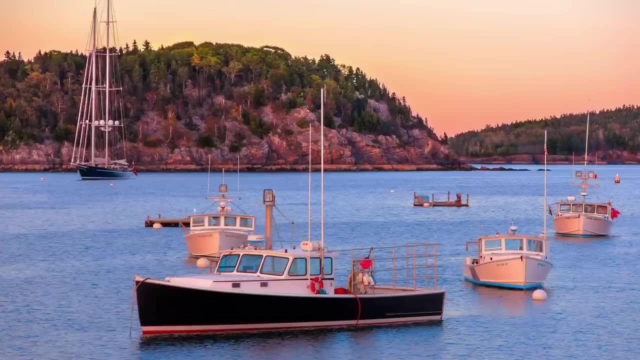 Beyond it, the easternmost part of the coast is known as the Down East and is even more sparsely populated. It's home to Mount Desert Island, the sixth largest island in the entire lower 48, and the location of Acadia National Park, The town of Bar Harbor. 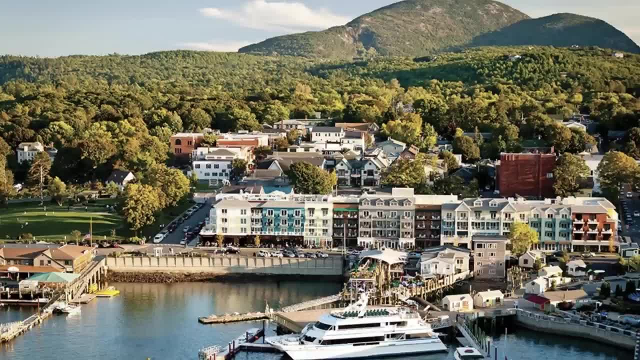 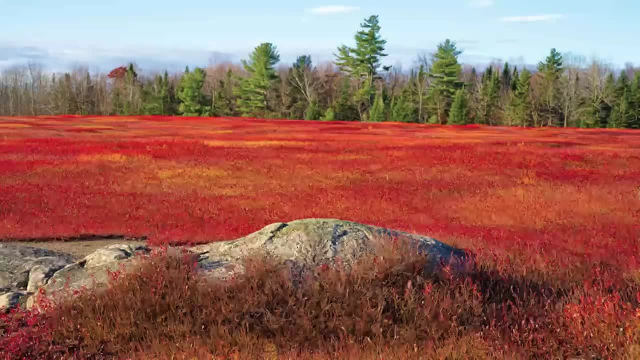 located on the island is a major tourist destination, bringing around 4 million people, with Acadia the fifth most visited national park in the entire country. The island is also home to Jackson Labs, a major genetic research site. These coastal regions are home to a number of blueberry farming areas, port towns and shipbuilding. 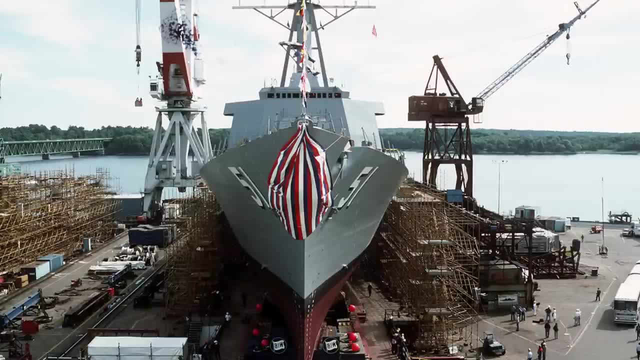 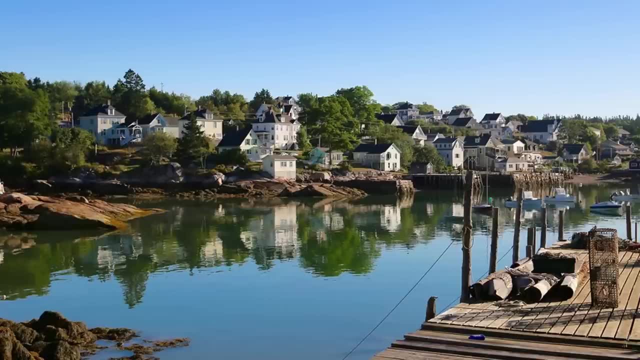 yards like the Bath Ironworks in Bath. Maine has one of the strongest maritime traditions in the country and fishing has been an essential part of the state's history, economy and culture. Fish and oysters are major exports, but the dominant product is, of course, lobsters, One of 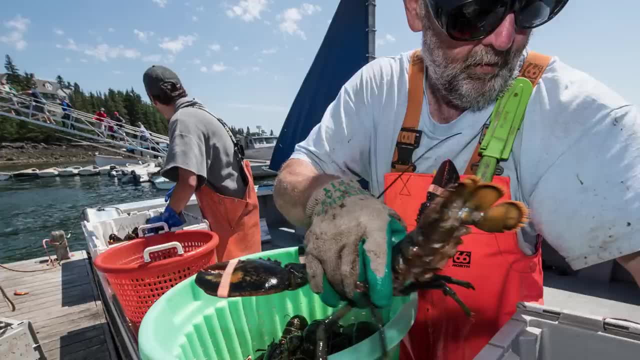 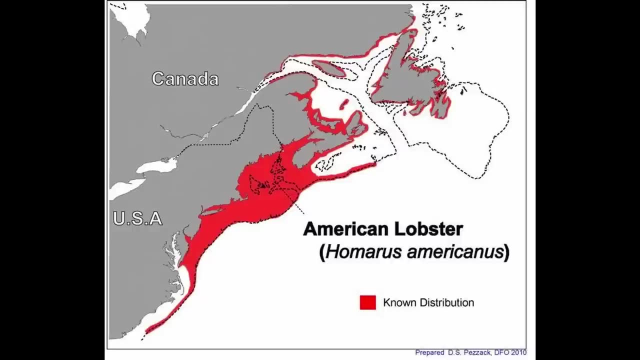 the major seafood catches. lobster is Maine's largest export and the state is the largest lobster producer in the country. With the waters off the northeastern US home to huge lobster populations, Maine brings in well over 100 million pounds of lobster each year. 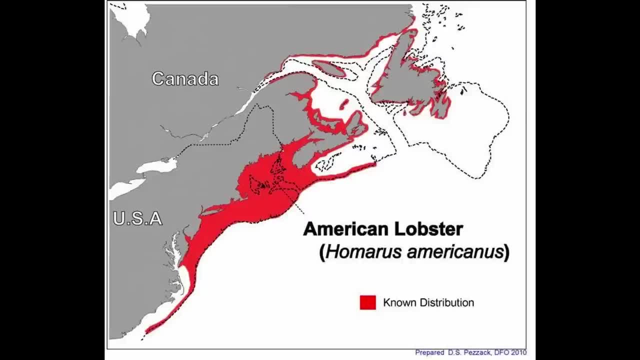 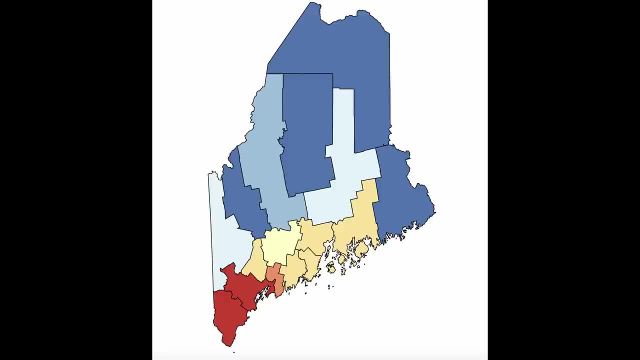 The lobster fishing is huge across the state's coast. it's especially dominant in the Down East. While most of the coast is growing, the far northeast area around the Canadian border has seen its population decline over the last decade. Moving inland, the land climbs upwards. 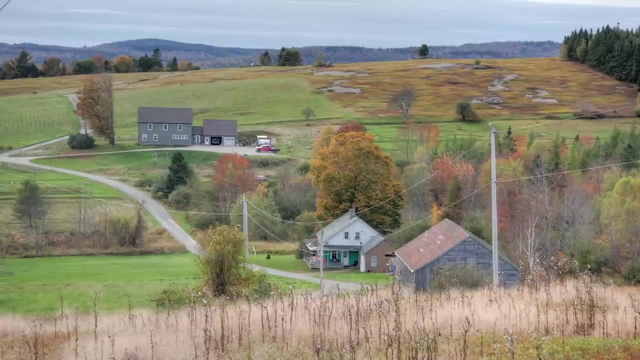 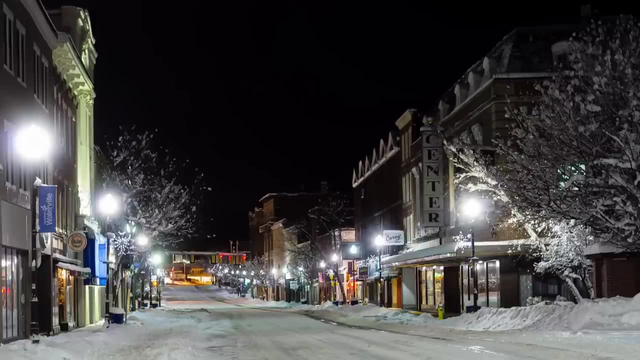 It's still home to a population that, relative to the rest of the state, is fairly large. These were historic lumber and milling towns that grew along the rivers, such as Waterville on the Kennebec, Augusta, Maine's capital city further downstream, and the state's second and 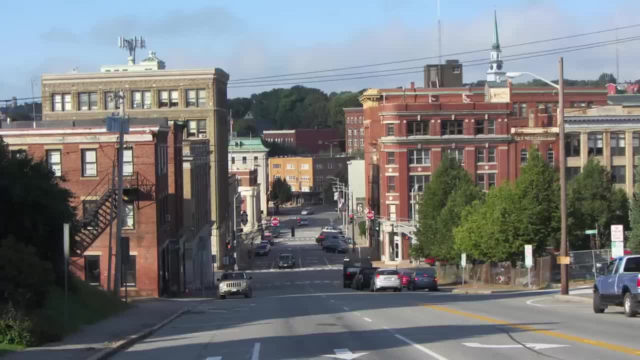 third largest urban areas, respectively home to 61,000 and 60,000 people in them and their suburbs, Bangor in the south central part of the state, along the Penobscot River, and Lewiston, in the southeast, along the Androscoggin River. 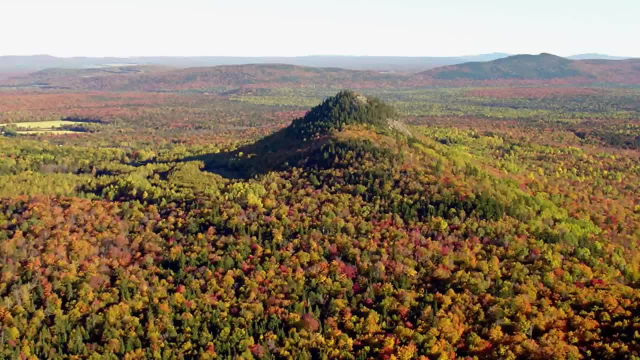 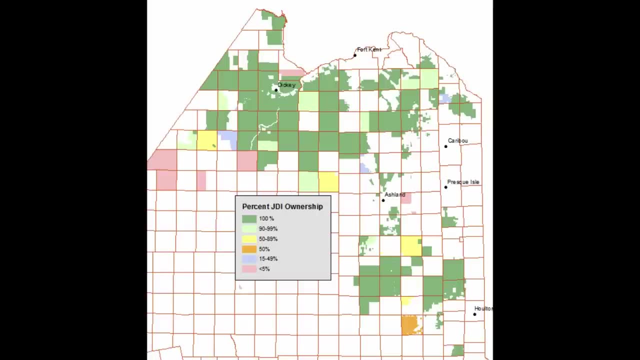 Further north, the landscape becomes mountainous and sparsely populated, not only difficult to inhabit, but much of it privately owned by paper and lumber companies, one of which, JV Irving, owns more than 5% of all the land in the state. 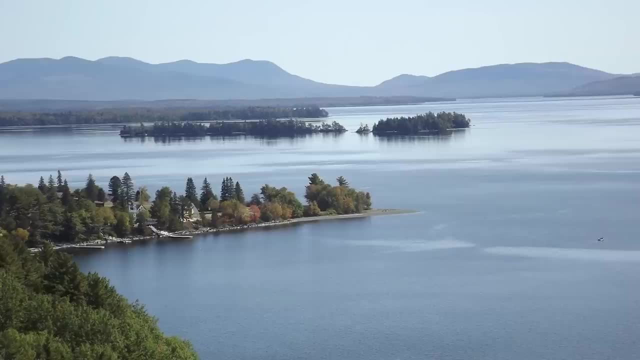 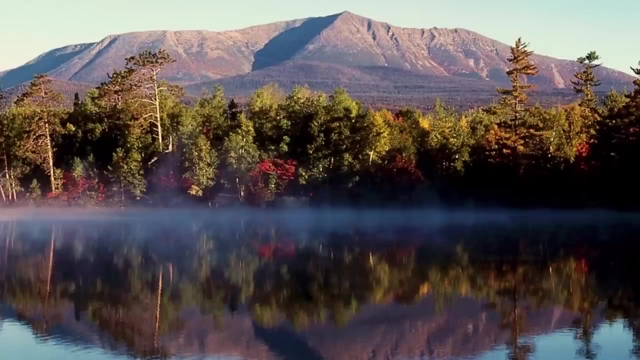 The mountainous north of the state is filled with lakes, including the largest in the state, Moosehead Lake, as well as high peaks like Mount Katahdin, mountain cabins and vacation destinations and ski resorts like Sugarloaf. This is truly a remote wilderness, the likes of which are difficult. 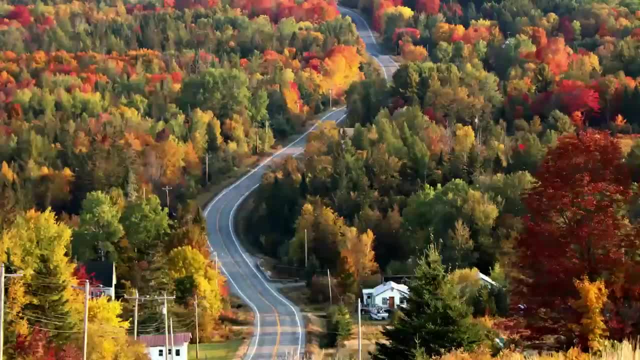 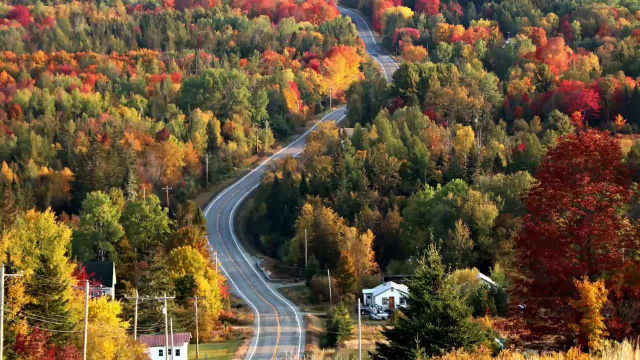 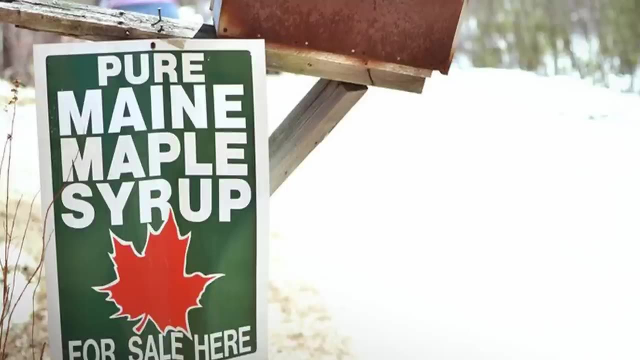 to find on the east coast, a beautiful landscape whose forests turn spectacular shades of red and orange in the fall, home to around 60,000 moose, six times more than any other state in the lower 48.. After Vermont and New York, Maine is the third largest producer of maple syrup in the country. 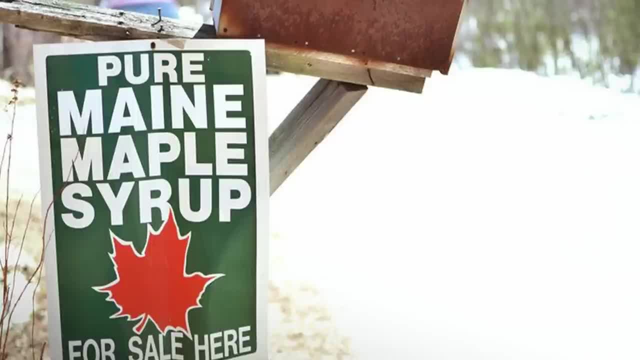 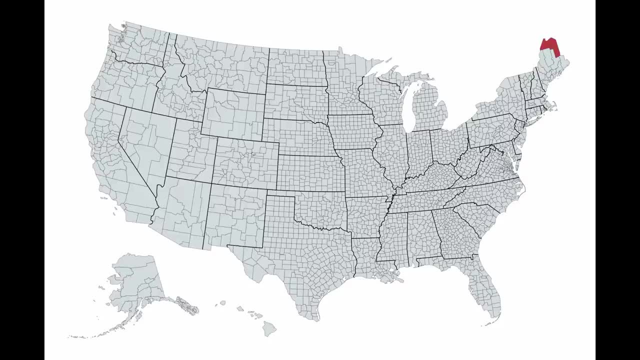 and much of it is from this part of the state. Finally, there's the enormous Aroostook County, the second largest county east of the Mississippi and larger than Rhode Island, Delaware, Connecticut and New York. While the western part is mostly sparsely populated forest, in the north and east towns like Fort Kent, Mattawaska and Presque Isle hug the St John River or sit not far from it. The valley of the St John River is really the only major agricultural region in the state. famed for its potato production, It's the heart of America's Acadian population. 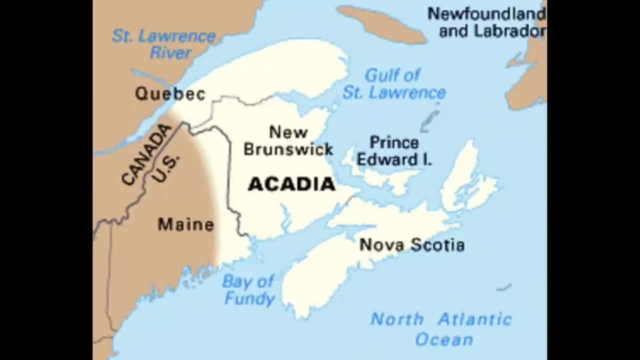 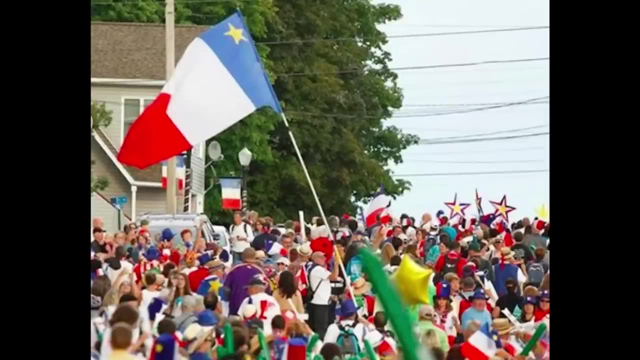 a French-speaking ethnic group descended from an old French colony, which I'll talk more about later. The St John Valley is a population center in New Brunswick too, and many towns sit right across the border from one another. Acadian flags fly throughout the 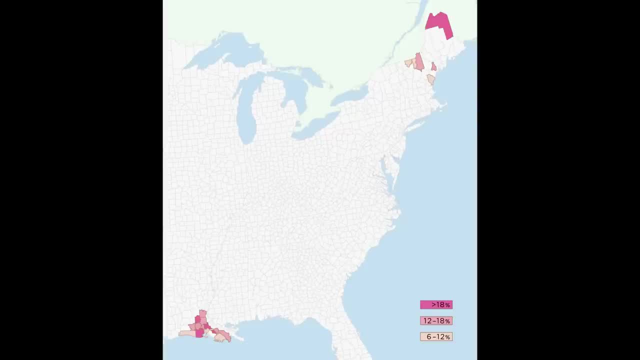 region and Aroostook County has the fourth largest population of French speakers in the entire country, with 22% of the county's population speaking the language, primarily the local dialects of New England and Bwyan French. A number of towns are majority Francophone. 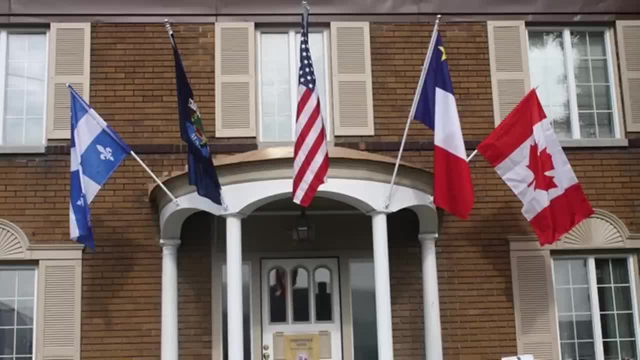 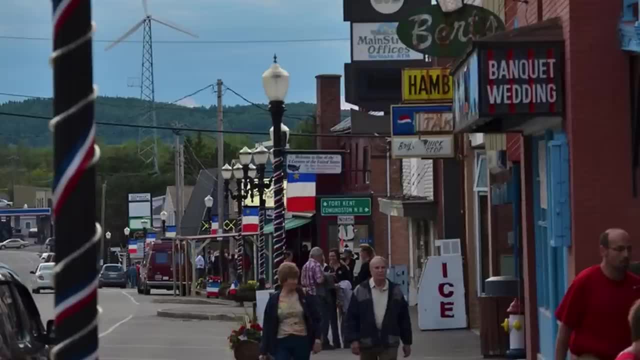 the border city of Mattawaska is the most Francophone town in the country, with 84% of the speaking French. 9 of the 10 most French-speaking towns in the US are all in Aroostook County. It's one of, in my opinion, the most fascinating cultural regions in the country. 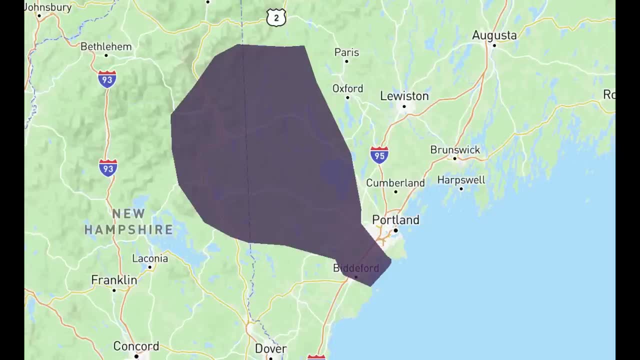 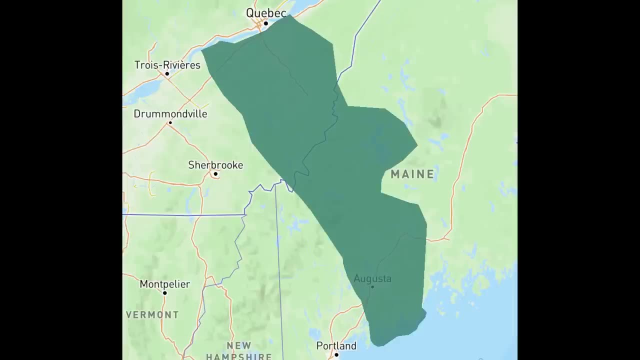 What is today. Maine was originally home to a number of different indigenous peoples. The Pequocket lived in the south, near where Biddeford and Portland are today. Further east from the mid-coast, north into the mountains, were the Nanran Suak. 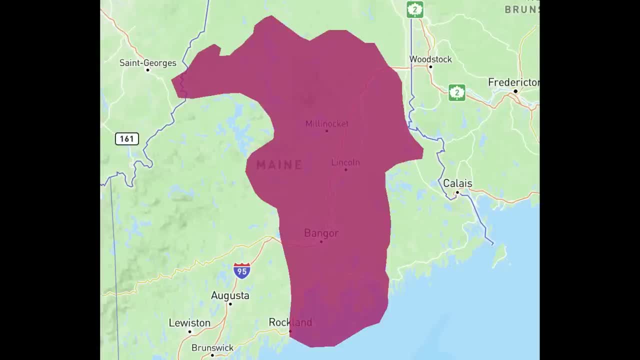 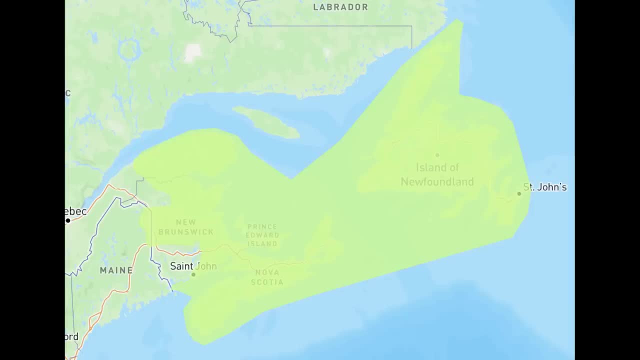 From Penobscot Bay and Mount Desert Island. north were the Penobscot. the Passamaquoddy lived throughout the down east, the Wollastawiek and the Mi'kmaq people in the far north of Maine. 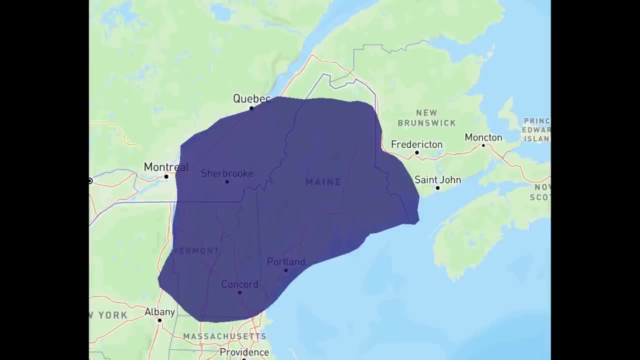 and the Abenaki throughout most of the state. As European colonists arrived in North America, they brought with them diseases such as smallpox, which the native people of the continent had not been exposed to and, as such, had little immunity. Disease decimated the continent's indigenous 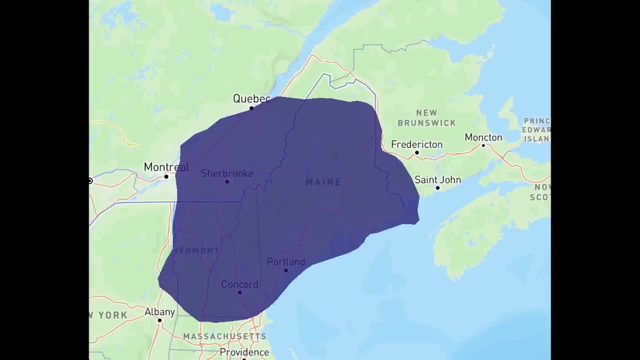 population, killing 90% of them, and those that survived often died at the hands of colonists. as Europeans expanded their settlement westward, It's unclear who the first Indians to reach the region were. Greenland Vikings explored the North American coast. but the southernmost settlement found as of yet is in Newfoundland, thought to be the Vinland Colony. A Norse coin from the era known as the Maine penny was found near Penobscot Bay, but it's unclear whether it made its way there from exploration. 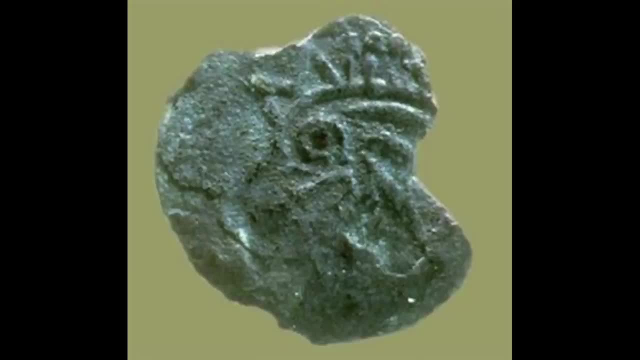 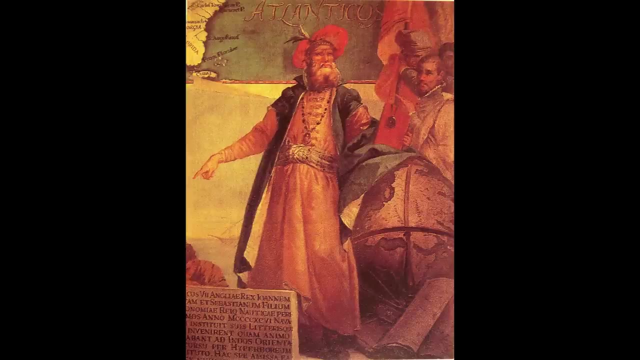 a lost settlement or simply as a part of regional trade routes. Venetian explorer Zwan Choboto, known to the English, whom he sailed for as John Cabot, visited Newfoundland and possibly made it to Maine, but regardless of whether or not he did, 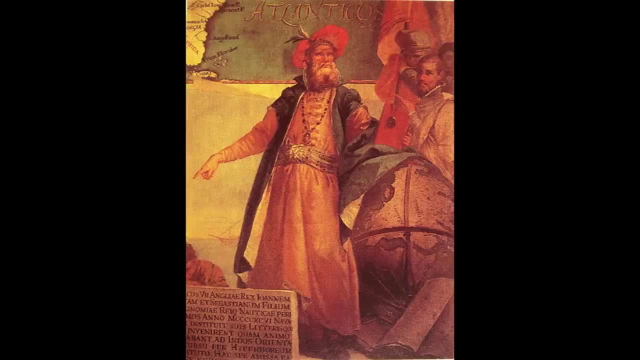 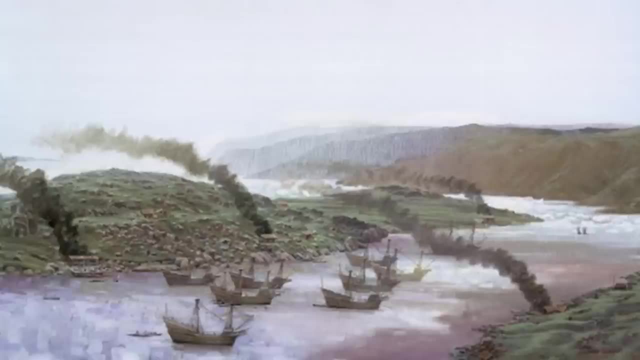 his voyage sparked interest in the rich fishing waters of the region, and fishing vessels from a number of European countries, particularly English, Basque and Portuguese fishermen, began making the voyage to the region, Though it's uncertain whether any went as far as Maine. 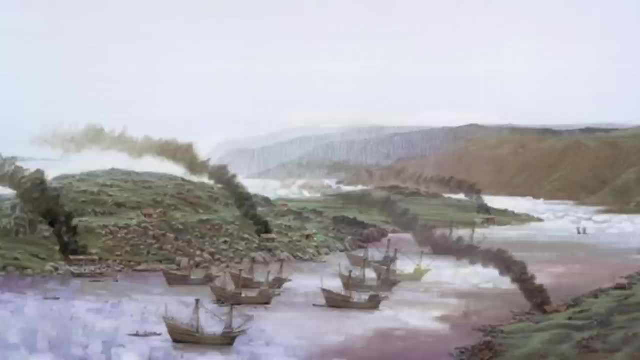 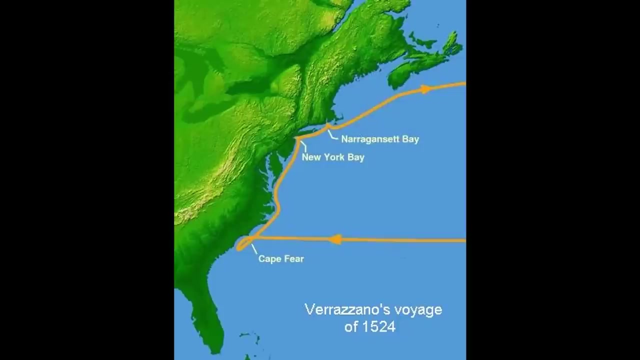 fishing villages were founded throughout Newfoundland and Canada's maritime provinces well before any formal colonial ventures reached this part of North America. The first documented European explorer to reach the region, though, was Italian explorer Giovanni de Verrazzano, who sailed for France and reached Maine in 1524.. 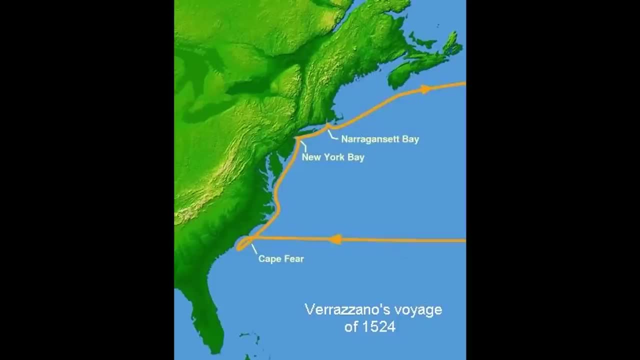 European colonization in the region, however, wouldn't fully begin until the 1600s, when it would become the site of some of the earliest French and English colonial ventures in what would become the United States. In 1604,, a group of French colonists led by Samuel de, Champlain and Pierre Duguay landed on a tiny island past Macquarty Bay, on what is today the main side of the US-Canada border. They named the island St Croix and called their colony Acadia, But a harsh winter and scurvy outbreak killed many of the settlers, who fled just a year later across the. 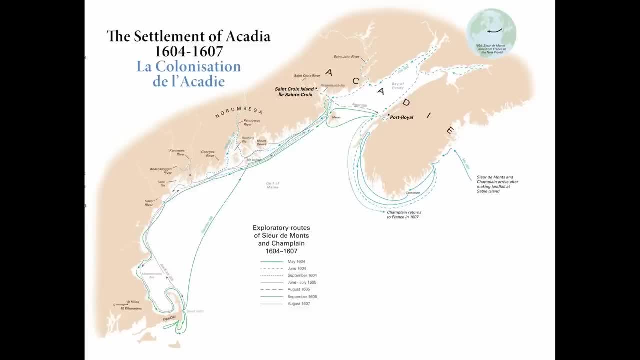 Bay of Fundy to what is now Nova Scotia, founding a town called Port Royal, which would become the Acadian capital. At the same time, the English were becoming increasingly interested in establishing colonies on the North American mainland, something they'd attempted a few decades before with the 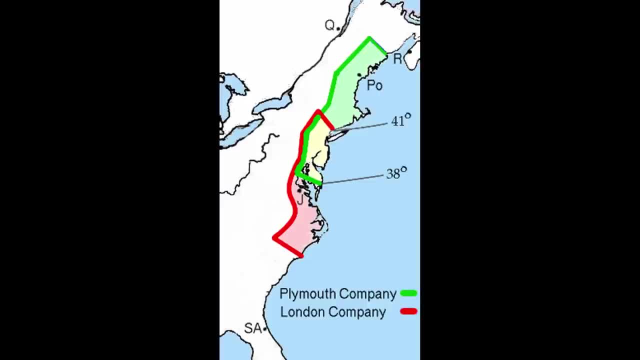 failed Roanoke colony. The English referred to the entire coast between the North American mainland and the French colony of Acadia and the Spanish colony of Florida as Virginia and established two colonial companies, the Virginia Companies of London and Plymouth. 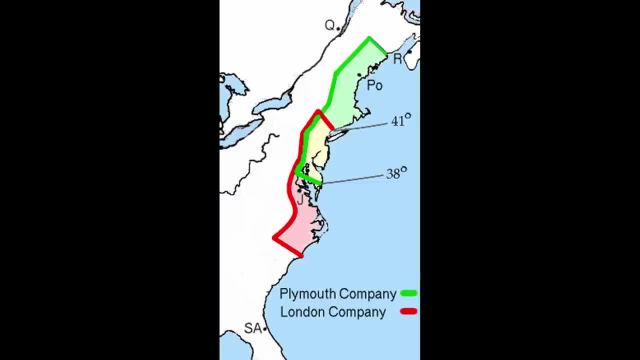 respectively to begin settling the coast In 1607, each of the colonies brought settlers to the land they called Virginia. The London Company founded Jamestown near Chesapeake Bay, while the Plymouth Company went to what is now Maine, founding the Popham colony. 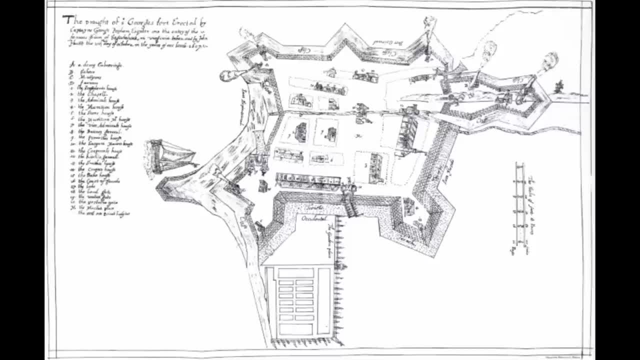 slightly after Jamestown, at the mouth of the Kennebec River. It was the third English settlement in what would become the united states. but the popham colony lasted only about a year before it ran out of food and the settlers deserted it. returning to england with popham, no. 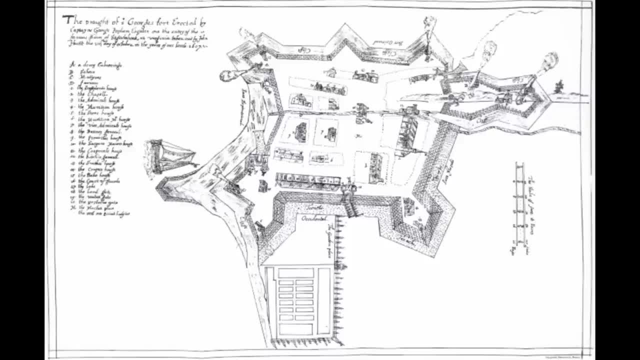 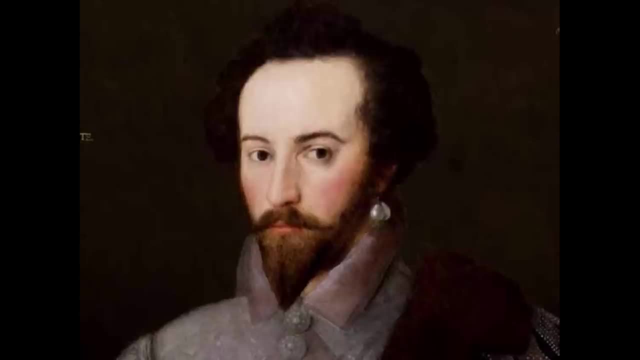 more, the name virginia came to refer to not the entire eastern seaboard but just the area around the remaining colony of jamestown. in 1622, english king james the first granted two noblemen, john mason and ferdinando gorges, a charter to found a colony between the merrimack and kennebec rivers. 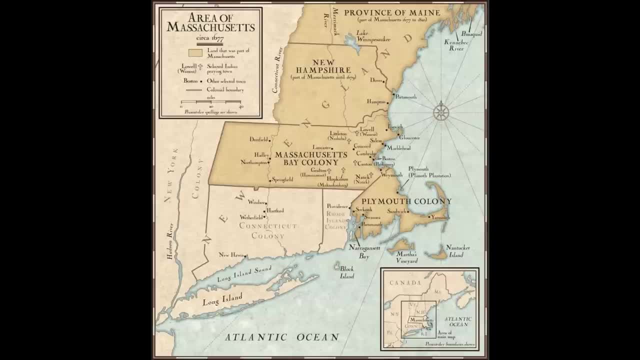 which they called the province of maine. seven years later they split their colony in two on the piscataqua river. mason took the southern section, calling it new hampshire and gorges the north, which he named new somersetshire gorges, later founded another colony within his lands. 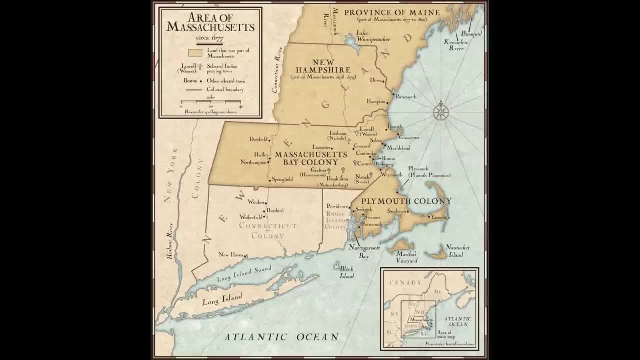 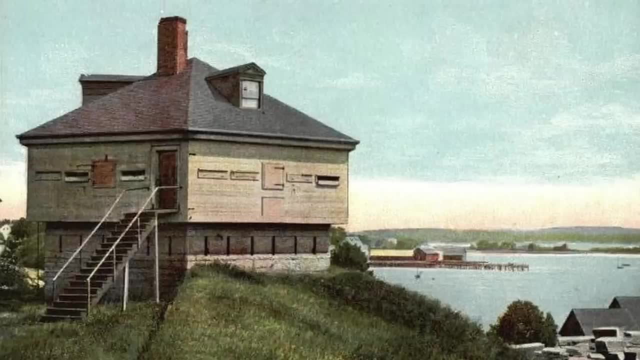 called ligonia, but both colonies were still collectively called the province of maine. english fishing villages later sprung up along the coast of the colonies, such as kittery, saco, agamemnicus, later york, which was the first town officially in the united states to have a colony within the province of maine, which was the first town. 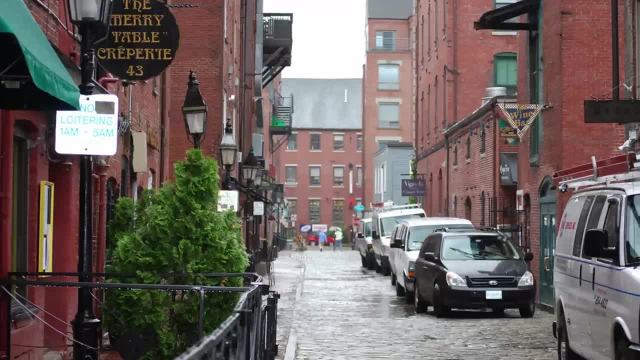 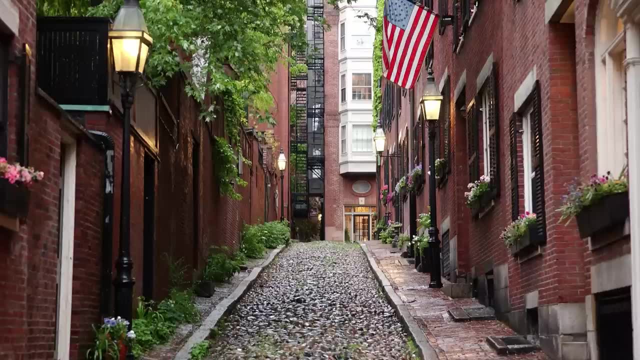 incorporated in what would become the us and casco, which would become portland. to the south, though, the massachusetts bay colony, centered on the port city of boston, was growing populous and powerful, with a population 12 times the size of maine. in 1652, they used a border dispute to claim: 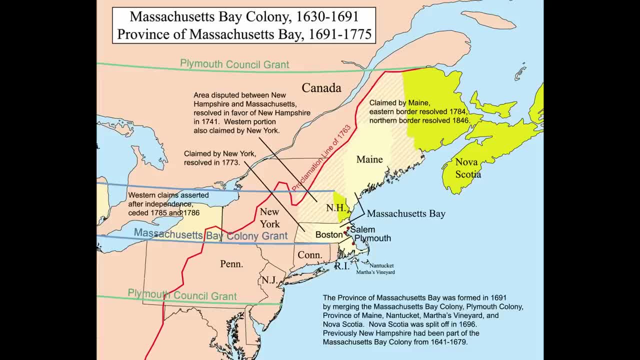 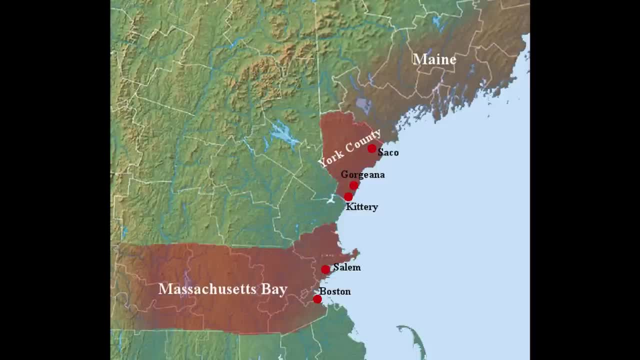 control of lands far to the north, including the colonies of new hampshire and maine, and one taking control of both. after two decades, new hampshire would split off again, leaving the new province of massachusetts bay physically divided into two by new hampshire's short coastline. a number of colonies were briefly unified into 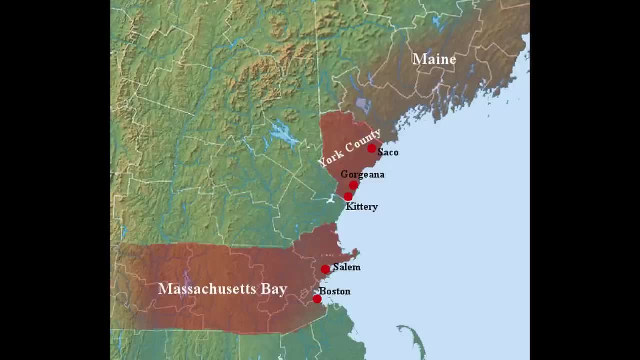 the unpopular dominion of new england, but after its breakup a few years later, maine remained a part of massachusetts, and would be so for the next century and a half. they called it yorkshire county, later shortened to york county, which is what the southernmost county of maine is. 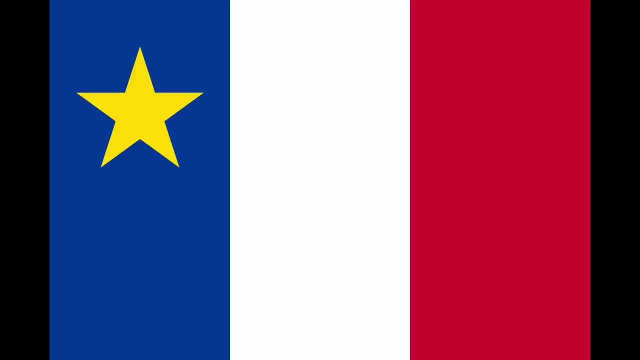 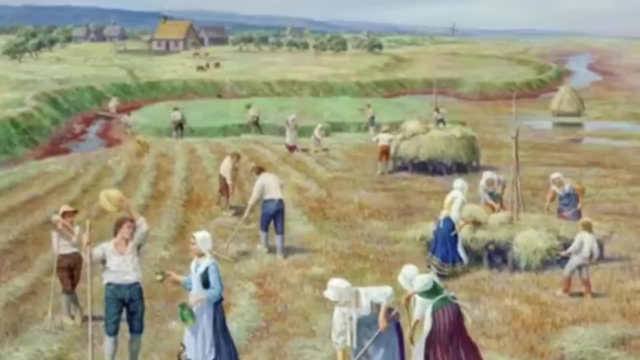 still called today acadia, which had been founded in maine but moved across the bay of fundy, had grown in population, with french acadian settlements spreading across what is today nova scotia, new brunswick and prince edward island and approaching york county. the region was on the periphery of french, british and native american control. as english settlers expanded inland throughout new england, war broke out between english colonists and native people, known as king phillips war, considered the bloodiest war in american history. proportional to the population at the time, it eventually resulted in the british conquering more indigenous. 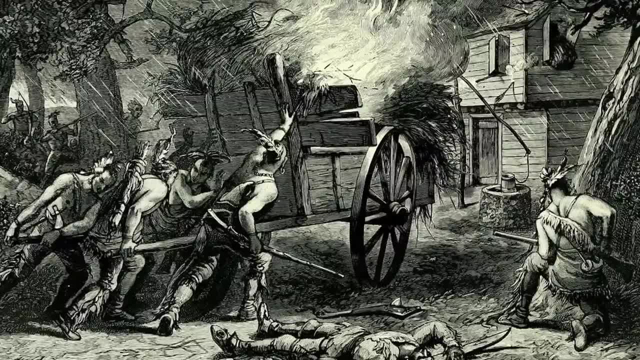 lands. after the war, the native people of the region became increasingly worried about british expansion as well as the growing power of the iroquois confederacy to the west. native tribes from lake champlain all the way to newfoundland unified into a powerful union called the wabanaki. 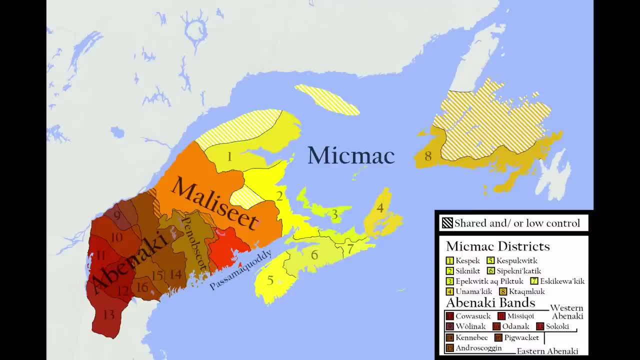 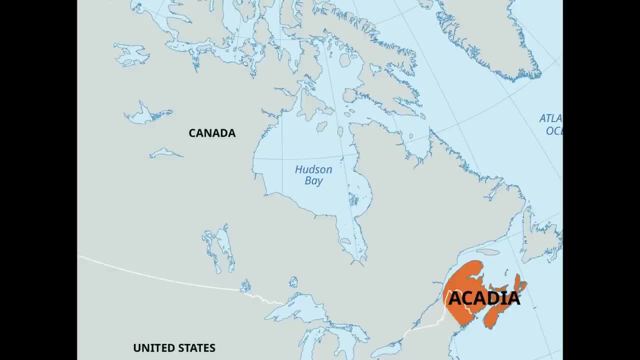 or donland confederacy aligned themselves with the french of acadia, separated from the french colony of canada along the st lawrence river. the acadians had developed their own distinct culture and national identity, but throughout the early 1700s britain launched a series of 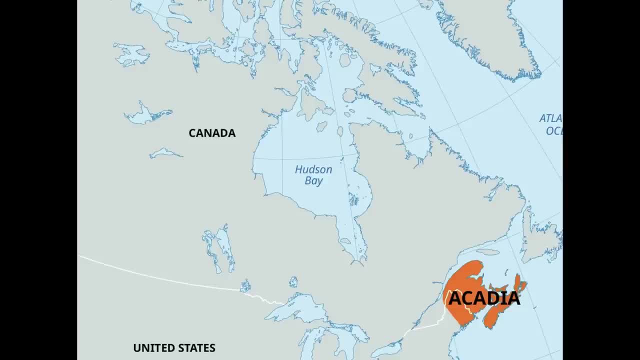 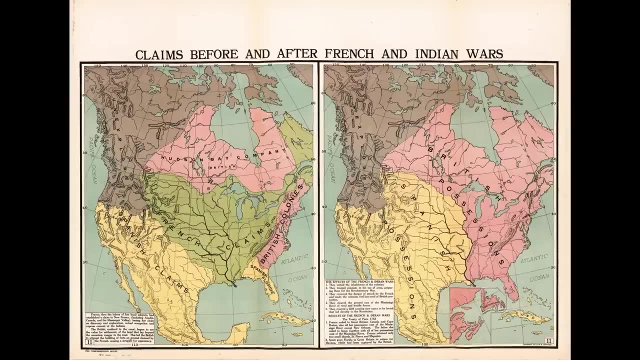 attacks on the colony, capturing the capital city of port royal. by the end of the french and indian war between the two empires in 1763, britain took control of all the french colonies east of the mississippi, including acadia and their ally, the wabanaki. 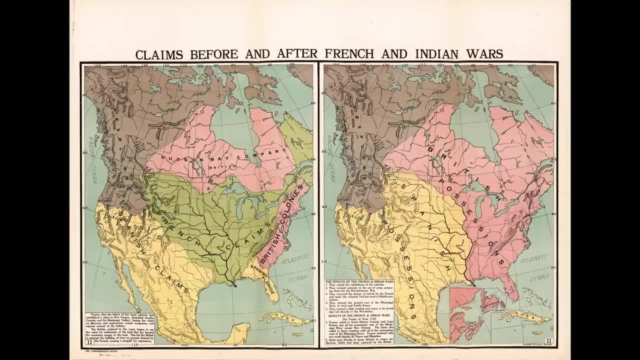 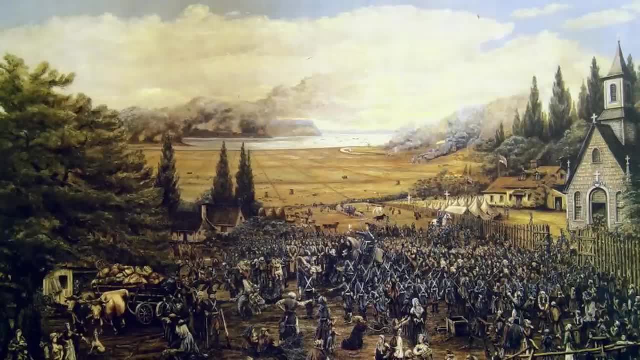 confederacy lost effective control of the region. britain began a brutal and violent expulsion of the acadians, in which thousands died and most were forced from the colony. many left for louisiana, a former french colony, where they had linguistic ties and settled in the swamps and bayous west. 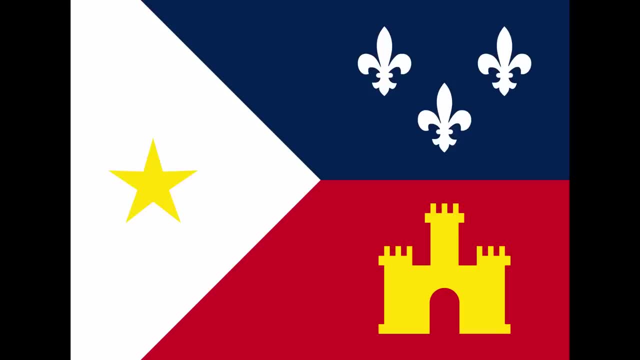 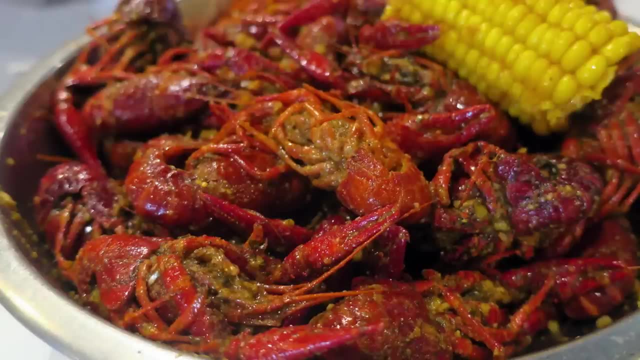 forming a unique cultural identity, dialect of french and style of cuisine influenced by the region, the name acadian changing to cajun. only around a fifth of the acadians successfully remained in hiding within acadia from the british many who'd lived along the saint john river in what. 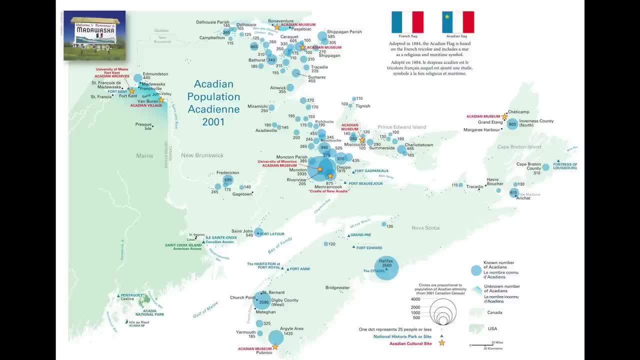 was now the colony of nova scotia and later to be split off into new brunswick, fled to the upper reaches of the region, founding towns and was now the acadian region of the north of maine. massachusetts began to send more settlers north to yorkshire and many others left for new brunswick. 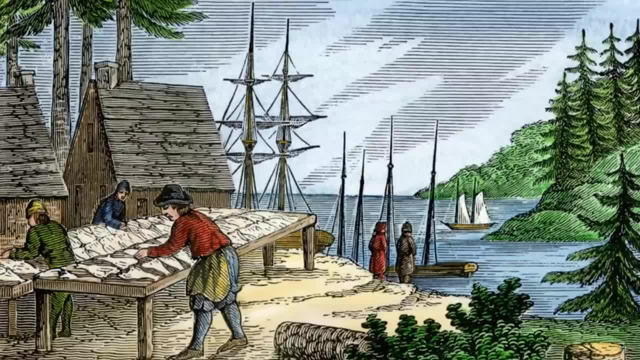 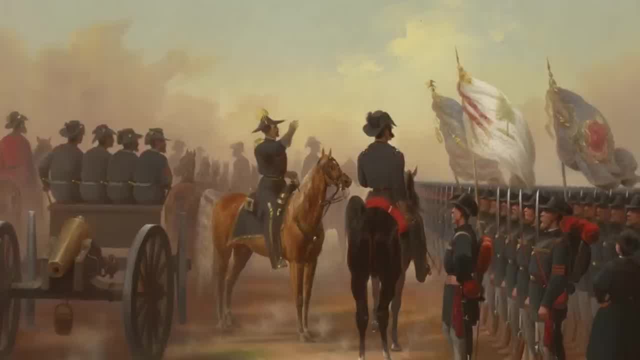 as they fled to the upper reaches of the region, founding towns and what is now the acadian region of the north of maine County, offering free plots of land, and the region's population began to grow rapidly. When the Revolutionary War broke out, this northern part of Massachusetts was strongly 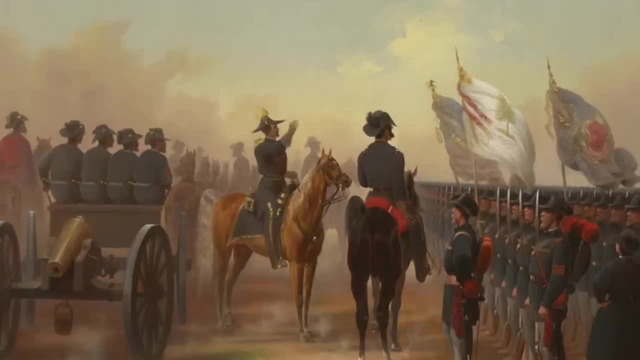 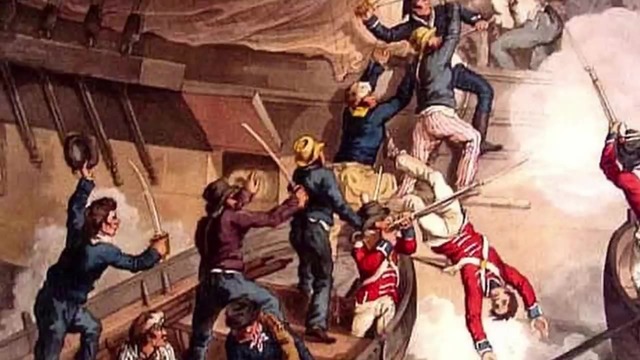 in favor of independence. Close to British Canada, it was home to the Battle of Machias, the war's first naval battle. Britain occupied parts of the county, calling it the Colony of New Ireland, and burned down the town of Falmouth, sitting on Casco Bay. After the war's end. 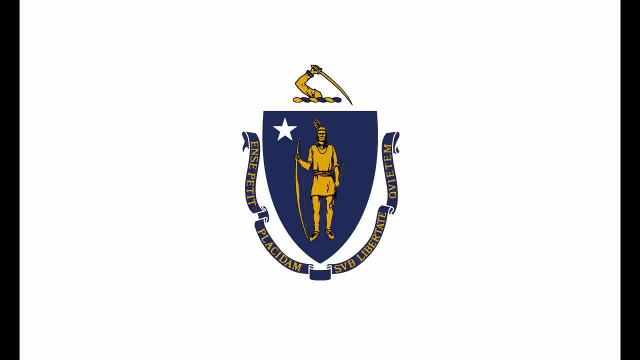 Falmouth would be rebuilt and renamed Portland. When the Revolutionary War ended, Massachusetts ratified the Constitution and joined the United States on February 6, 1788, becoming the sixth state to join the Union. But the Treaty of Paris, which ended the conflict, left the borders between: 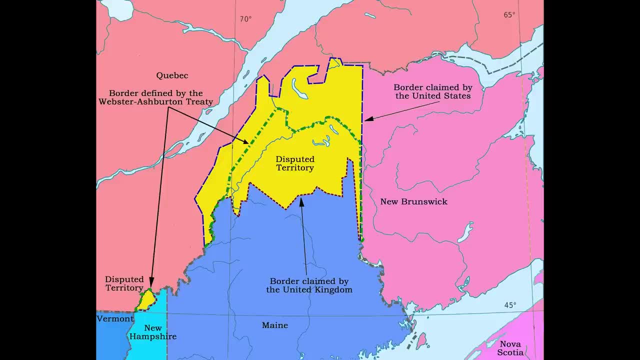 Maine and British Canada unclear: Britain claimed lands deep into the northern and eastern parts of the region, while the United States claimed that Massachusetts extended far closer to the St Lawrence River than Maine does today. It was difficult for Massachusetts to govern the physically separated former Colony of Maine. 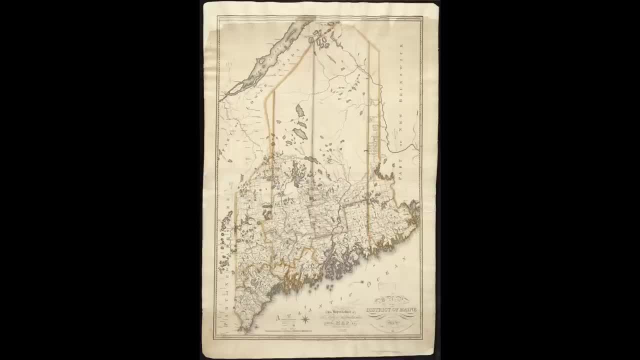 and almost immediately locals began calling for it to become a separate state. To make governance easier, Massachusetts gave the region, which they named the District of Maine, a local government. The district grew rapidly, tripling in population from 1785 to 1800,. 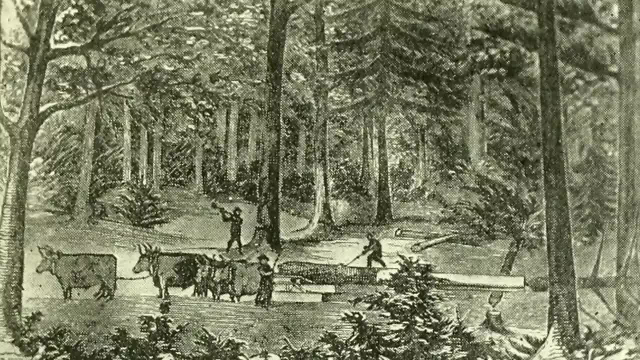 as settlers, mostly of English descent, moved north from Massachusetts. By 1800, the district would be home to 150,000 people, and it would double within the next two decades alone. The district thrived as poor settlers moved in, buying up land in the near interior of the state. 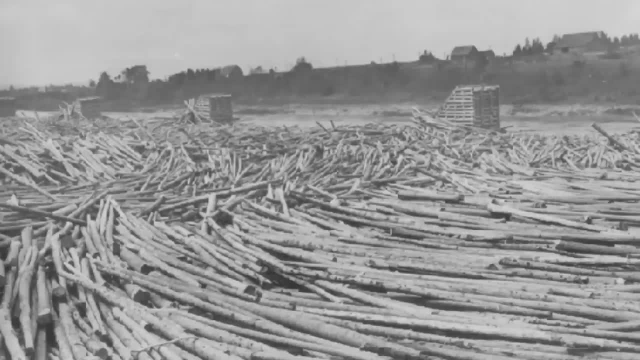 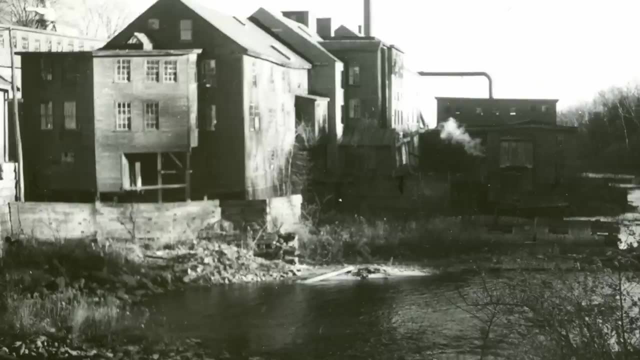 Lumber mills sprung up along rivers and industrial towns developed around them. Bangor became a major center of logging and in just a few decades became the largest lumber port in the world. Lumberjacks logged the District of Maine's rich forests and in Bangor and other 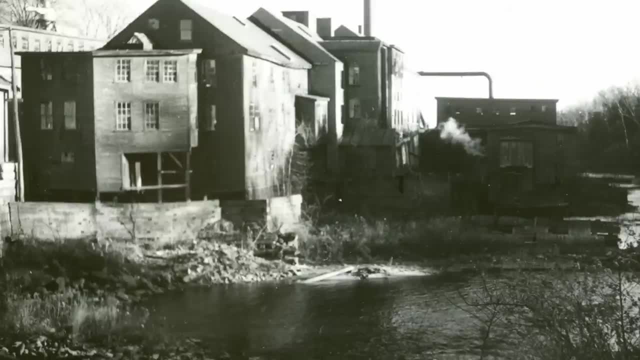 interior river towns, sawmills processed the logs, shipping the wood from there downstream to the coast, from where it was shipped to ports across the country and the world. Coastal cities like the Bay of Islands. the Bay of Islands and the Bay of Islands were the most much-needed sites for logging. 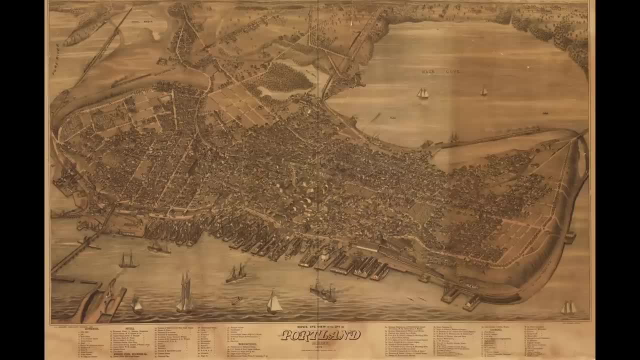 Coastal cities like the Bay of Islands. the Bay of Islands and the Bay of Islands were the most much-needed sites for logging. cities like Portland prospered and grew, trading goods from the interior with the rest of the US as well as global markets in Europe and the Caribbean, But as its population grew, a divide. 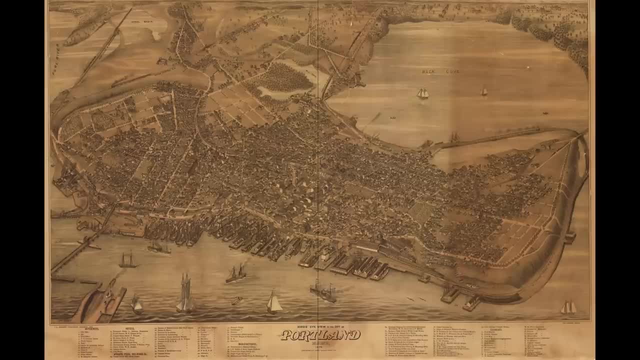 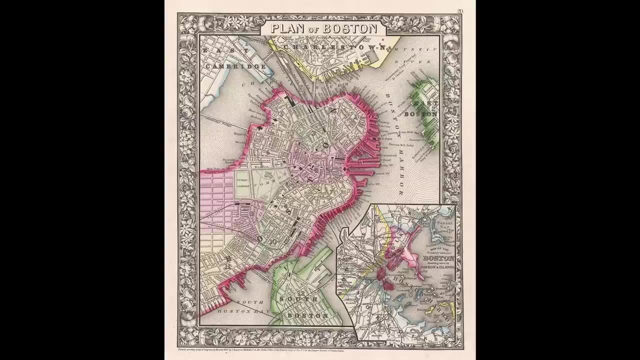 was growing as well. within the district, Coastal areas were dominated by trade and a wealthy merchant class which had close economic ties to Boston. Sitting on the edge of the country, Maine was quite vulnerable And in the colonial era it had made sense to many to have the protection of. 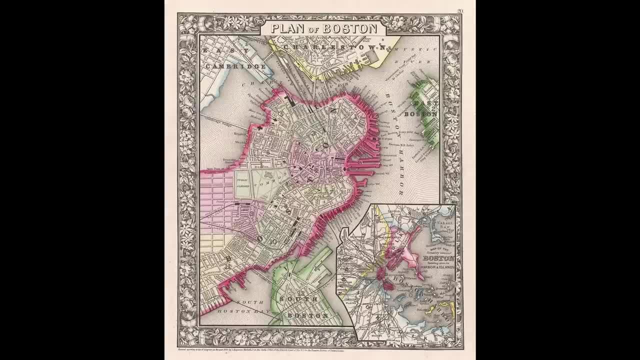 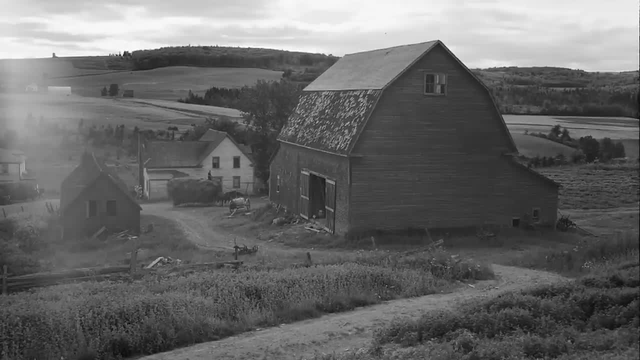 the powerful colony of Massachusetts Bay. But the Wabanaki and French were no longer a threat, and as the interior of the district grew, poor farmers and loggers living on the frontier increasingly felt that Boston did not represent their interests. Massachusetts and its politics. 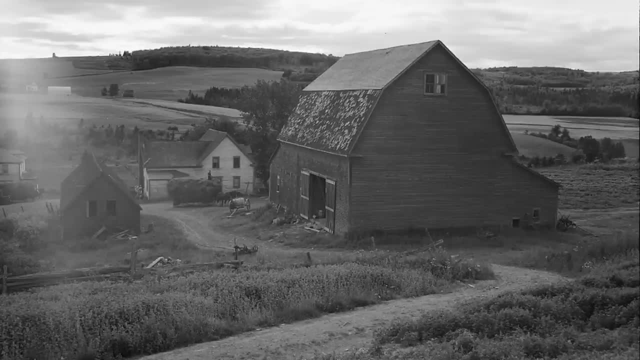 and religion was at the time dominated by a wealthy urban elite that the poor settlers of the woods and hills of the Maine frontier felt disconnected from. At the same time, the district of Maine was physically disconnected from the rest of Massachusetts and now had a large 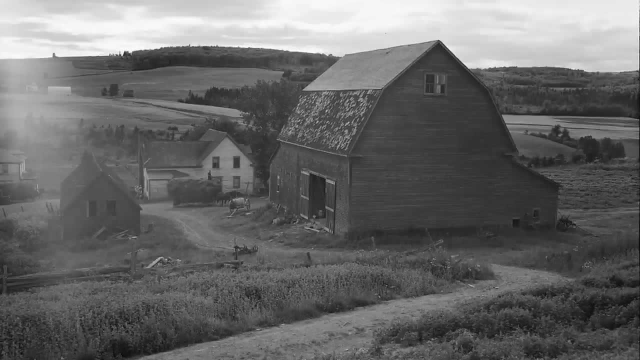 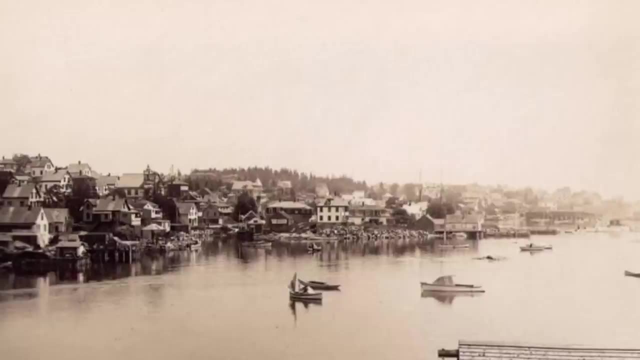 number of people living on the mainland. The state of Massachusetts was a place where the population could be made for statehood, But on the coast poor towns had close economic ties with Boston and typically supported remaining in the state. War between Britain and France caused 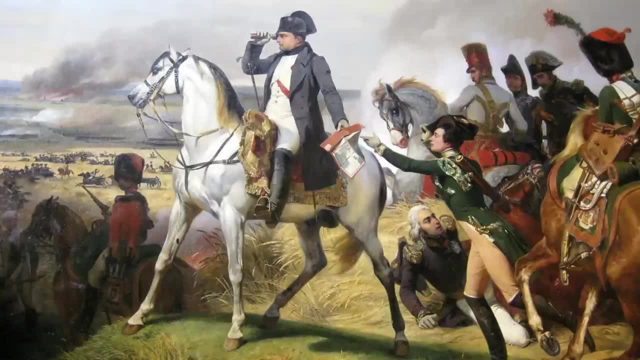 rising tensions in North America. The US was neutral and wanted to continue trading with both countries, but each wanted to stop American trade with their enemy. Britain blockaded American ships, even capturing crews of American sailors and forcing them into the British Navy. And 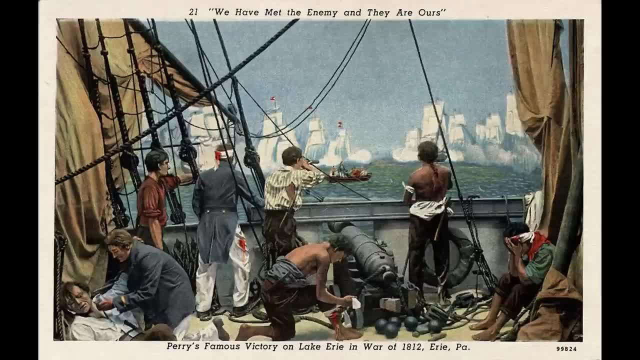 eventually, war broke out between the two countries, The war of 1812.. New England in particular was dependent on trade with Britain's colonies in Canada and the Caribbean, and the region's merchants opposed the war and the resulting ban on trade with Britain. Many New England merchants continued to illegally trade with 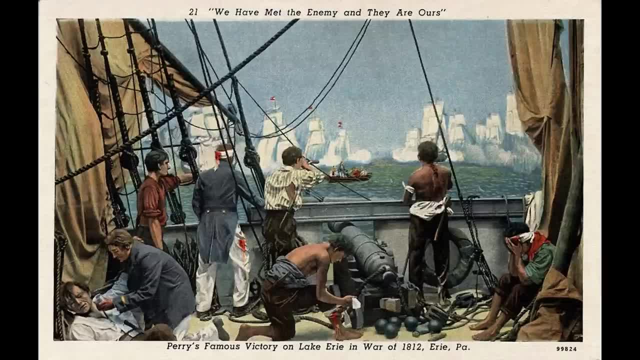 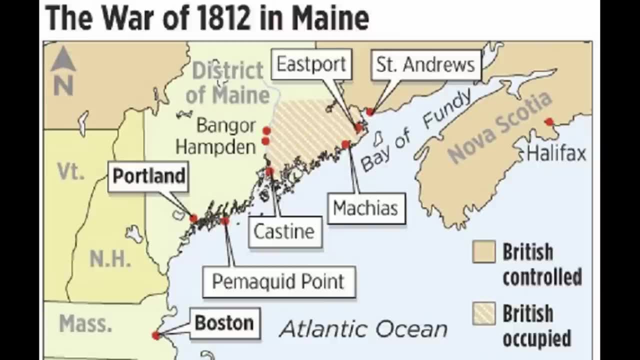 Britain during the war, and the Massachusetts state government was seen to be backing them. When British troops invaded Maine, again trying to establish a colony of New Ireland, Massachusetts did little to protect it. Britain was eventually pushed out, but their failure to defend the 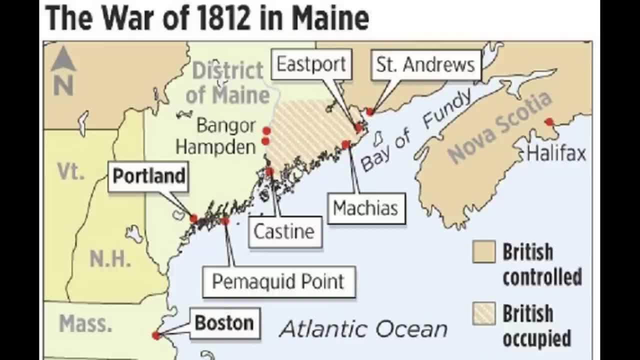 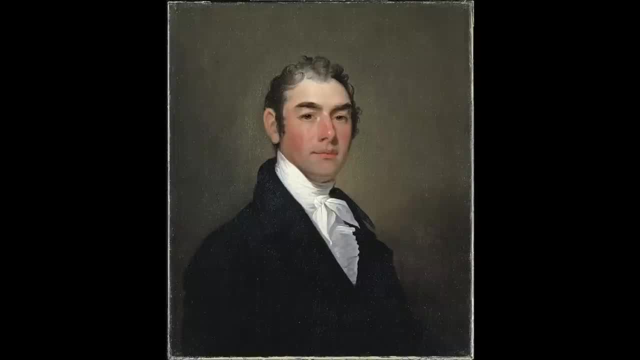 district had made support for independence from Massachusetts much more popular in Maine. William King, a merchant and state senator, became a major leader of the movement for statehood. In 1819,, after a number of successful referendums, the Massachusetts state government voted to allow. Maine to split from Massachusetts. Approval from Congress. the final step for statehood should have been simple, but it got wrapped up in the most controversial issue of the era, one that would eventually lead to civil war As the country was expanding west. 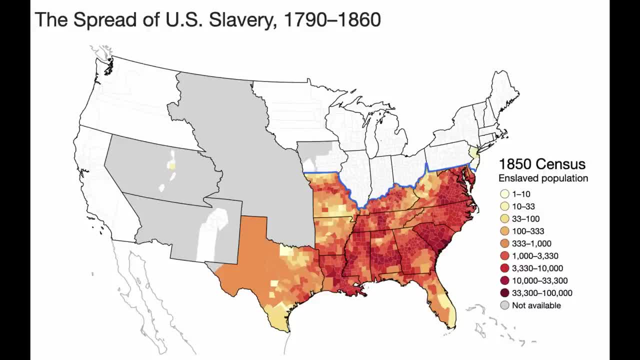 whether or not slavery would be expanded to newly added states became a major issue, as the addition of new states could shift the balance of power in the Senate one way or another, either for or against the horrible practice Many pro-abolition northerners 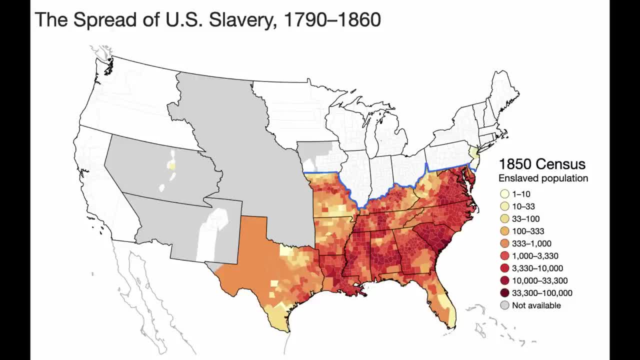 believed slavery should not be allowed to spread to new states, while many southerners believed new states should be permitted to allow it. Whether or not slavery was allowed to expand would likely tip the balance of power either for or against it in Congress, but neither faction. 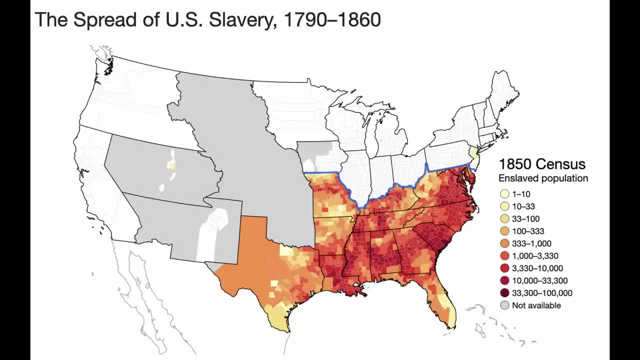 had enough support to do so. The New England state government, which was the first state to move the issue their way. It wasn't a problem in Maine. the abolitionist district didn't want to allow slavery within its borders should it gain statehood. but in Missouri, where there were a 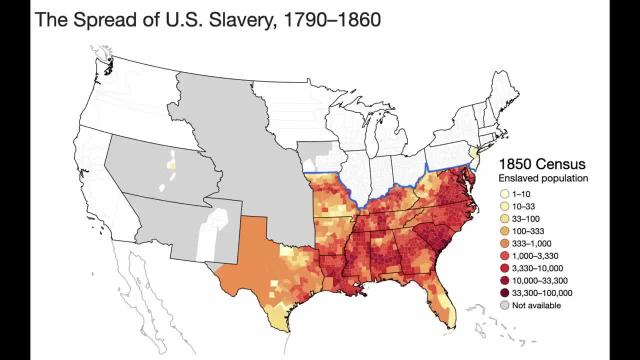 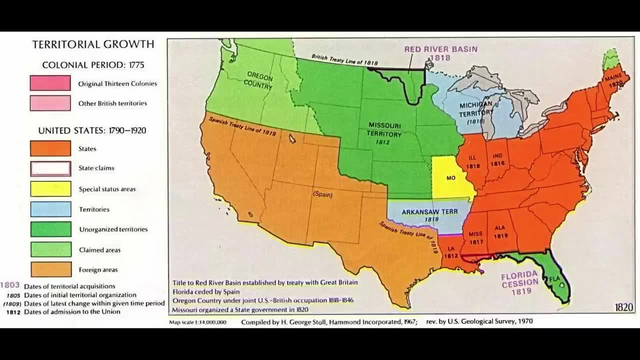 number of people living in slavery. it became an issue Because both were applying for statehood at the same time. some proposed adding both together as a compromise: one free state and one slave state. Eventually, what was known as the Missouri Compromise passed, allowing Missouri to 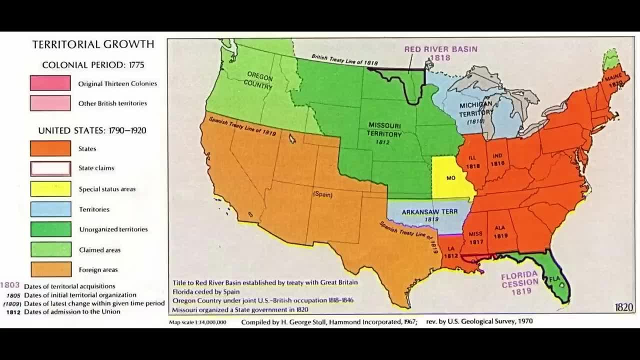 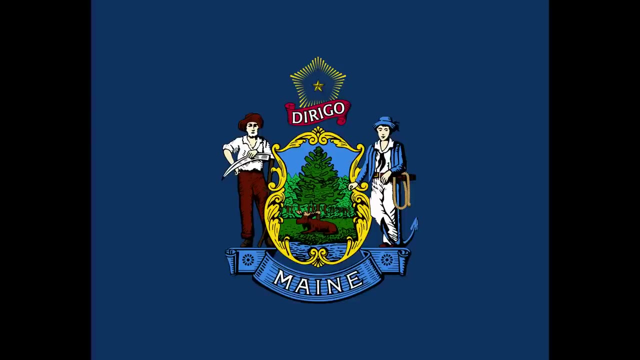 enter as a slave state and Maine as a free state and banning the extension of slavery to the state. On March 15, 1820, Maine was admitted to the Union, becoming the 23rd state, with William King, a leader of the statehood movement, its first governor. But the circumstances of its victory 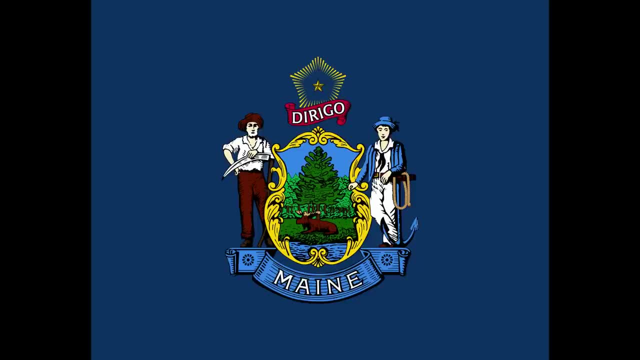 and a decades-long push for statehood soured the wind in the pro-abolition state. If anything, the Missouri Compromise simply pushed the issue of slavery further down the road. In just a few decades, civil war would erupt. Maine remained with the Union during the war. 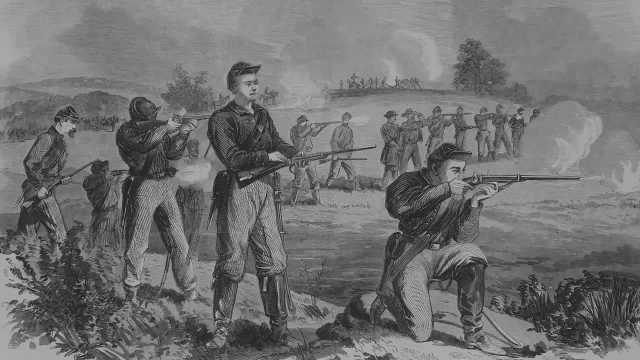 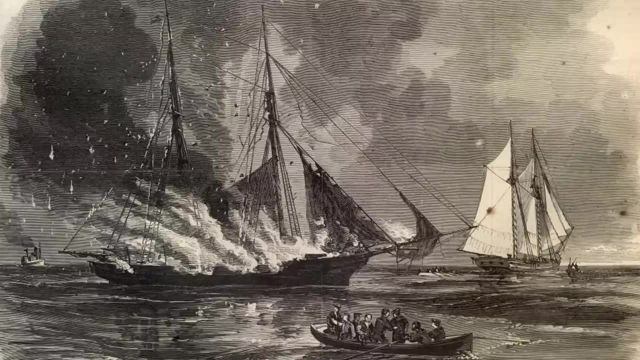 and 73,000 Mainers enlisted in the Union Army, more proportionally to its population than any other state. The state was actually home to one small naval battle, the Battle of Portland Harbor, where Confederate naval ships attacked a few fishing ships in Portland Harbor Not long after. 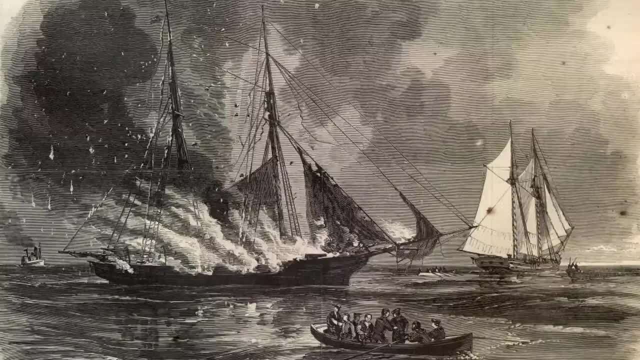 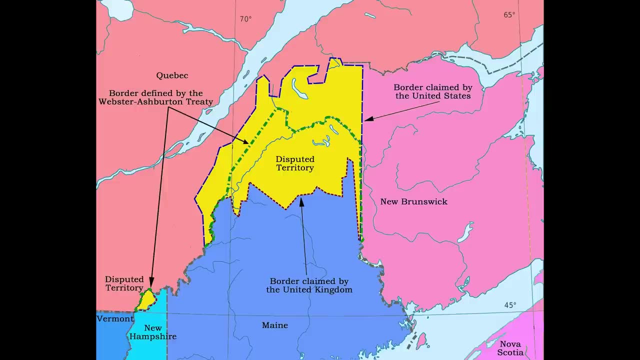 statehood, the capital was moved inland from Portland to Augusta, a small town on the Kennebec River. The long-standing border dispute between the statehood movement and the statehood movement over the northern part of the state, bloodless but tense, had been known as the Aroostook War. 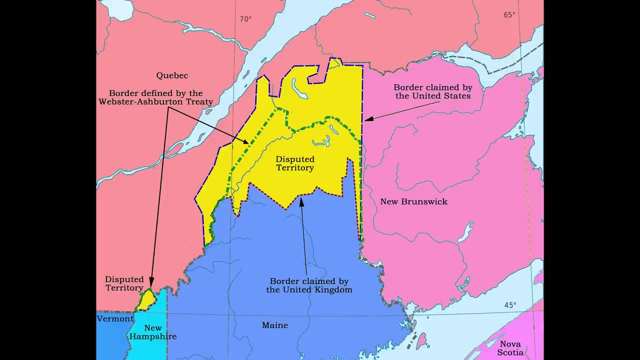 In 1842, the two countries settled it, drawing the border. the US and Canada currently have partway between their two claims. A number of important political figures from this era hailed from Maine, such as House Speaker James Blaine and Lincoln's first Vice President, Hannibal Hamlin, Maine. 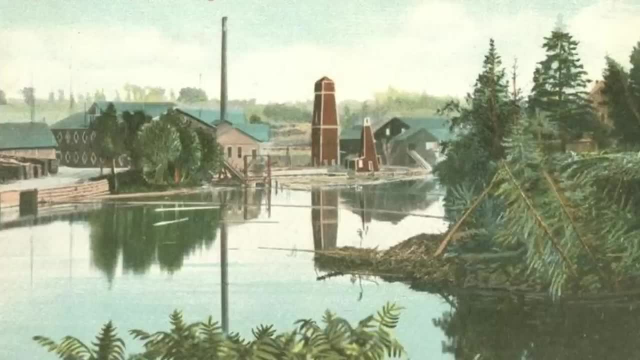 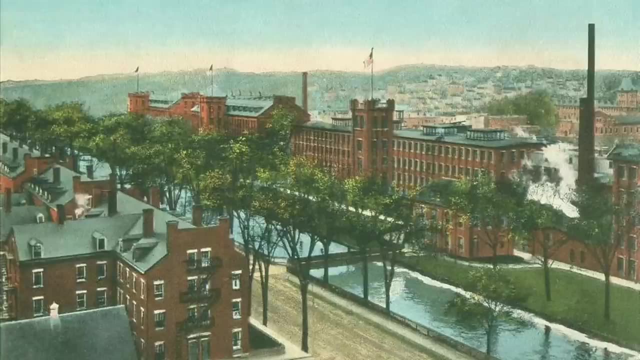 continued to grow fairly rapidly, especially as industry came to towns along waterfalls of the river. Bangor became known as the lumber capital of the world, Lewiston, a major textile producer with the dawn of the Industrial Revolution in New England, and Portland, an important port city. 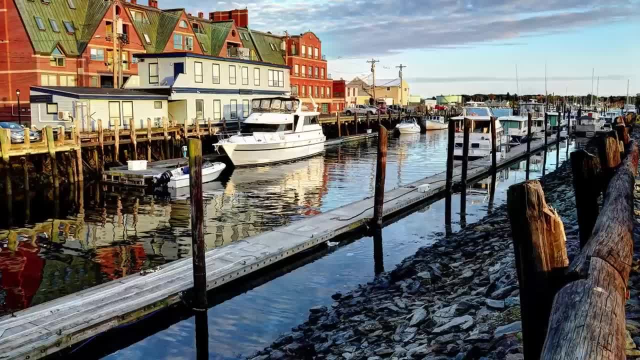 With the St Lawrence River freezing in the winter, a railroad from Montreal to Portland allowed the city to become the most important port city for Canada for much of the year, which helped it grow significantly. Shipbuilding became a major industry in coastal cities like 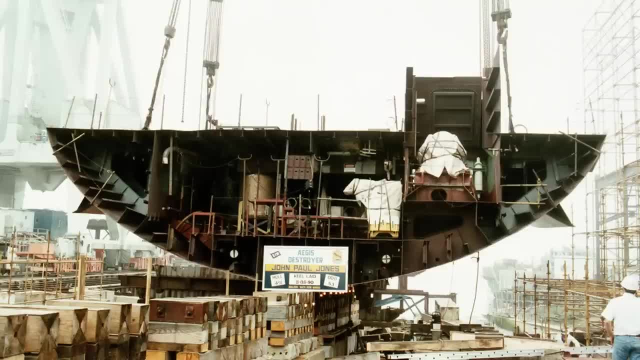 Bath, especially as the US ramped up international trade. Rich forests provided abundant timber, and raging rivers powered a thriving milling industry. Many people were farmers who grew just enough food to feed themselves and their families on small farms, and potato farming grew in the Acadian region of the St John Valley. Quarrying was important and, as always, fishing. 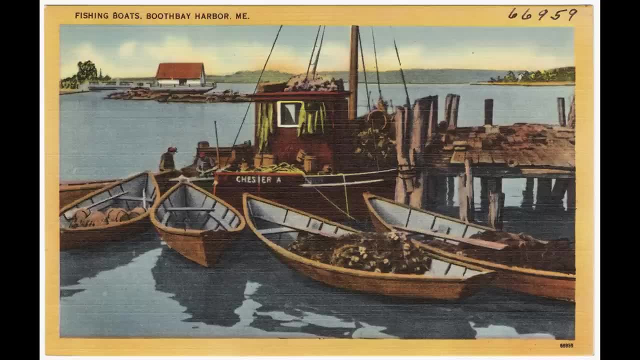 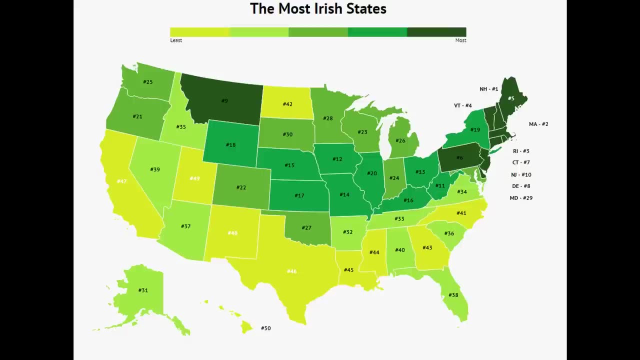 was a dominant industry At one point. a fifth of all fish produced in the US came from Maine. As the state's industries grew, immigrants came in. Many Irish immigrants fleeing the Great Famine arrived in the state joining an existing population mostly descended from. 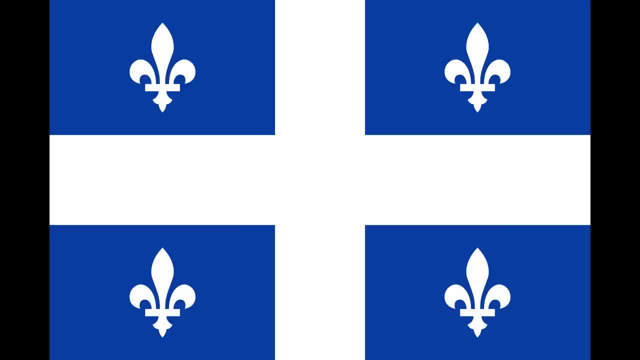 English and Acadian colonists. A large number of immigrants, though, came from just to the north. With its Acadian history, Maine already had significant French heritage and, as it industrialized, provided promising jobs close by. While some of these immigrants 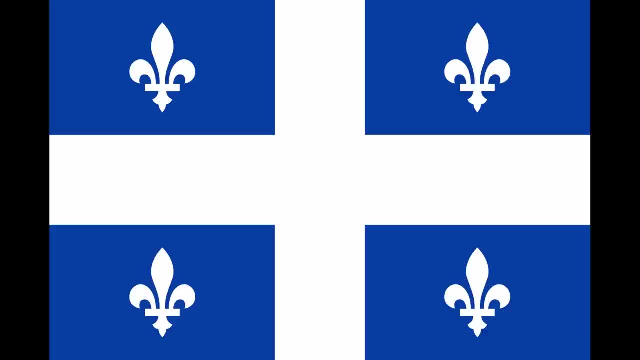 were Acadians. most were Quebecois, French Canadians coming from the still French-speaking but culturally distinct region of Quebec. Instead of staying near the border like the Acadians, many went south to industrial cities to work in the textile, lumber and paper mills. Lewiston in particular attracted a large number of French-Canadian immigrants. Maine's population growth slowed over time as the country expanded. west Mainers often packed up and tried their luck westward flocking to states like Ohio and Minnesota, As gold rushes and a booming timber industry drove settlers to the west coast. 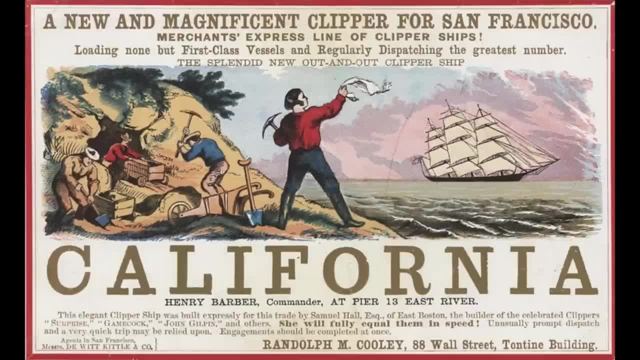 a large number of Mainers left for California, Oregon and Washington, as they were often already experienced in logging and could board ships leaving frequently from the state's ports. The state's industrial importance continued during the World Wars, when it became an important center of shipbuilding. 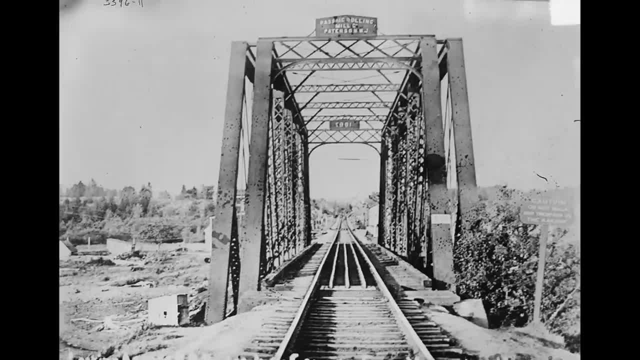 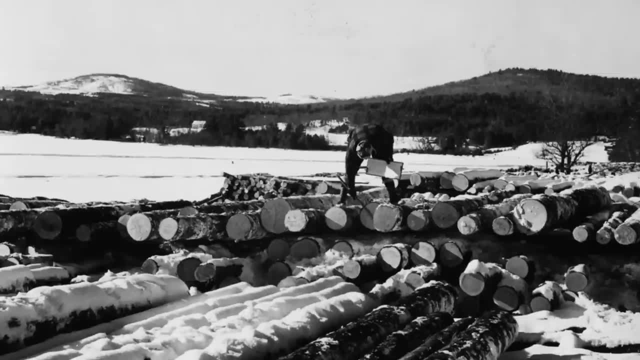 During World War I, a rail bridge at the border town of Vanceboro was bombed by German spies hoping to cut supply lines. Following the end of the war, the state went through several major economic changes. While paper milling and shipbuilding remained strong industry in. 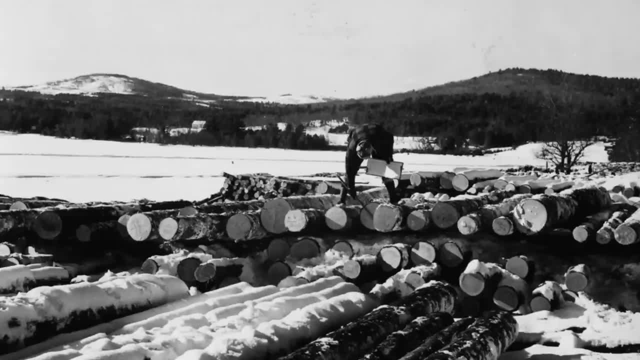 general declined as textile mills in particular left for other parts of the country and the world. It became difficult for smaller farmers to compete with the newer, large-scale industrial farms in Mainers left rural parts of the state. as agricultural jobs dried up, The state successfully. 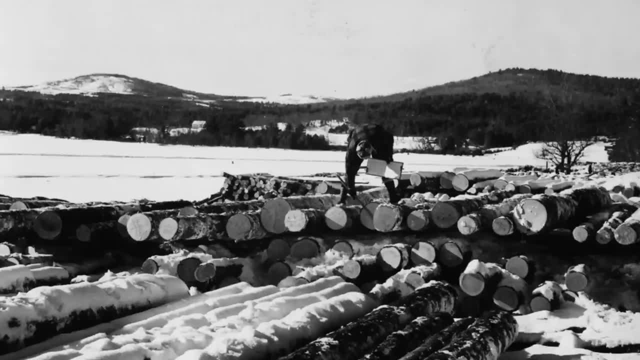 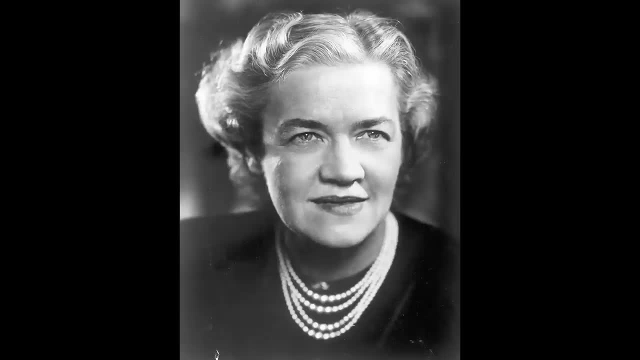 focused on cleaning up its rivers, which had faced significant pollution from the mills that lined them. Several prominent politicians rose to power in Maine in this post-war era, such as Margaret Chase Smith, who became the first woman in American history to serve in both the House of 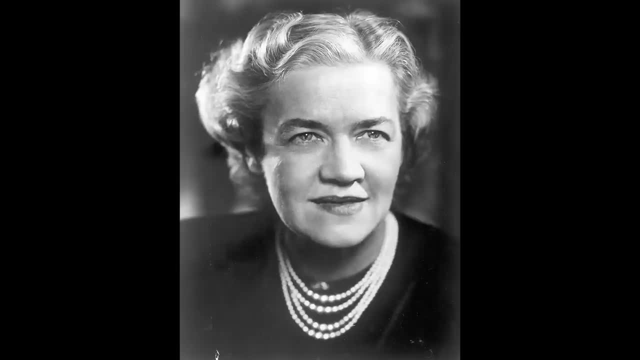 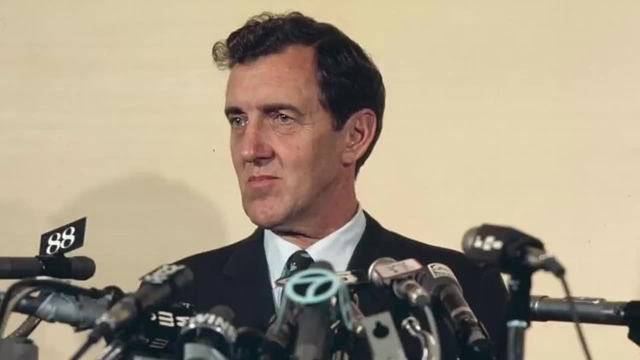 Representatives and the Senate. One of Maine's most influential politicians, though, was Ed Muskie, who was elected governor in a surprising upset before serving two decades in the Senate, narrowly losing the Vice Presidency in 1968 as Hubert Humphrey's running mate and serving as Jimmy. Carter's Secretary of State. While industry declined, tourism grew. Maine had always been a major vacation destination, but once it became connected to the interstate highway system, roads like the Maine Turnpike made it significantly easier for vacationers from Massachusetts and other parts of the Northeast to visit the state or buy up second homes. 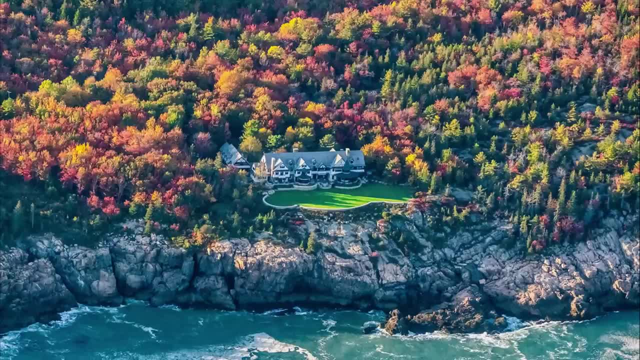 Its rural landscape, beautiful scenery and proximity to major cities made it an appealable place to visit. It was also a great place to visit when you were in the middle of the country, especially for people from the city hoping to find a rural escape, who found the 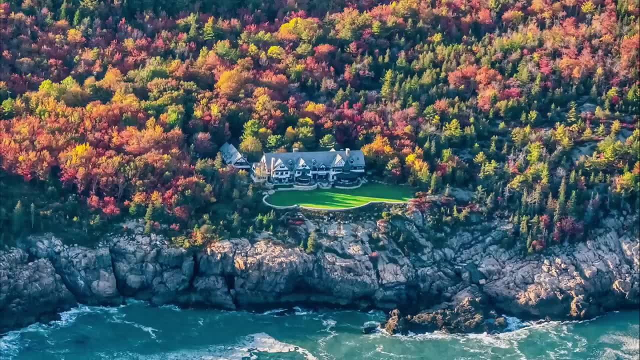 state's lifestyle. attractive, Wealthy families from the Northeast, like the Rockefellers and Bushes, were just a few of the many who bought second homes in the state. At the same time, though, most of the state's full-time residents are working class employed in industries like fishing. 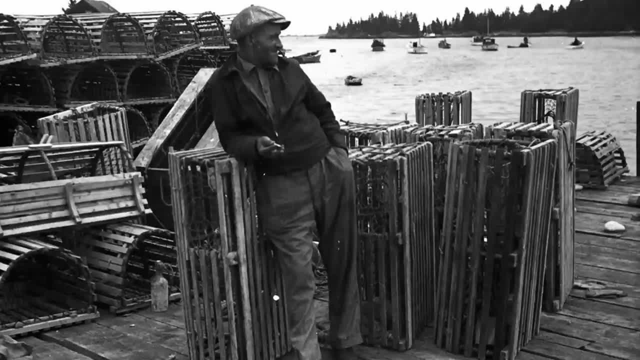 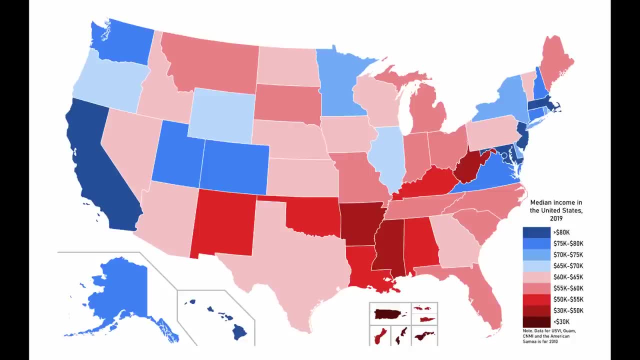 and logging. In this sense, it's an outlier as well. The state faces real problems with poverty and though it's roughly in the middle of the pack as a whole today, it has by far the lowest median household income of any Northeastern state. You have to go as far south as North Carolina. 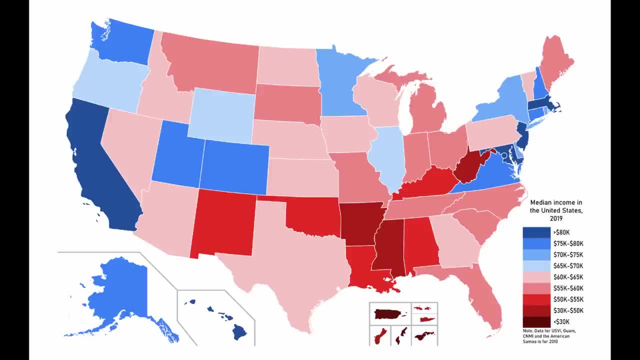 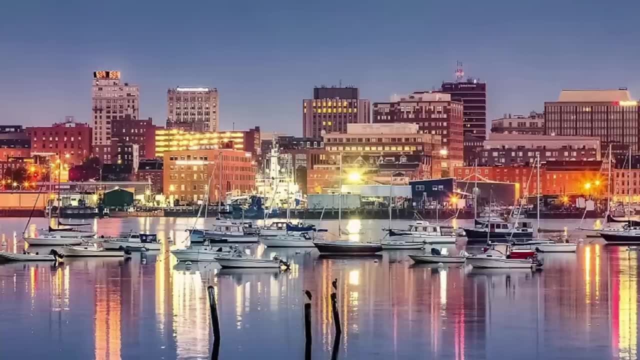 before you find a state on the Atlantic coast with a median income lower than Maine's. Maine's largest city and urban area by far is Portland, home to 205,000 people in it, and its suburbs, With just 66,000 people in its city, limits only the largest cities of Wyoming. 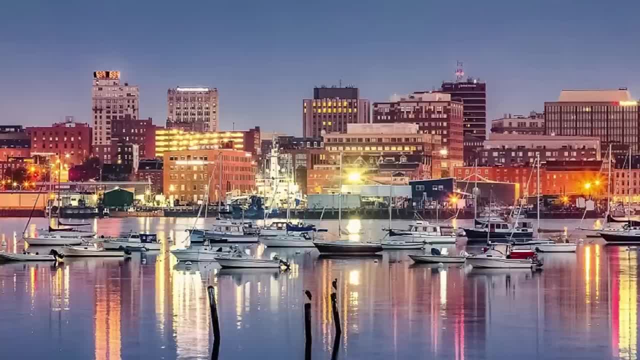 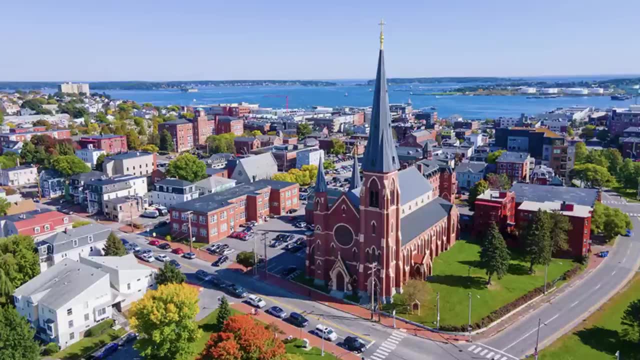 West Virginia and Vermont are home to fewer people than Portland. It's a blend of old and new, a historic port city revolving around a harbor on Casco, home to older brick buildings and more modern high-rises. It's nestled on a peninsula in Casco. 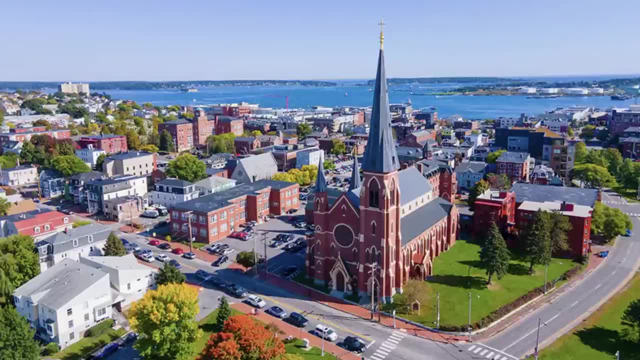 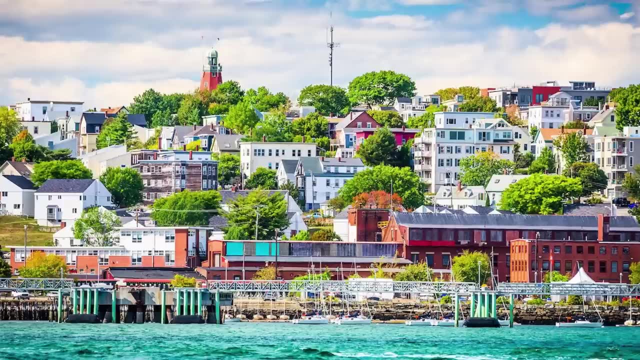 Bay in southern Maine and is surrounded by water. The Foer River, home to the port which the city is centered on, sits to the south and an almost fully enclosed bay called Back Cove lies to the north. It's a city of peninsulas, islands, forests and hills. Its suburbs are hemmed. 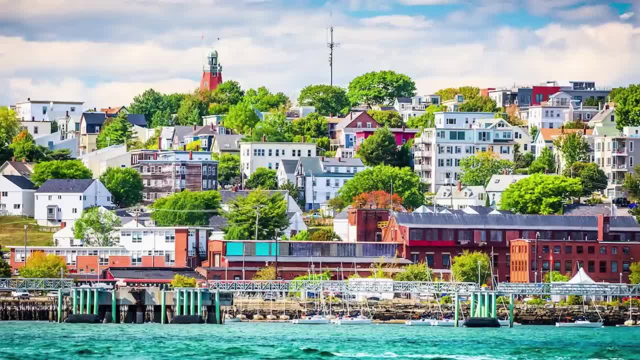 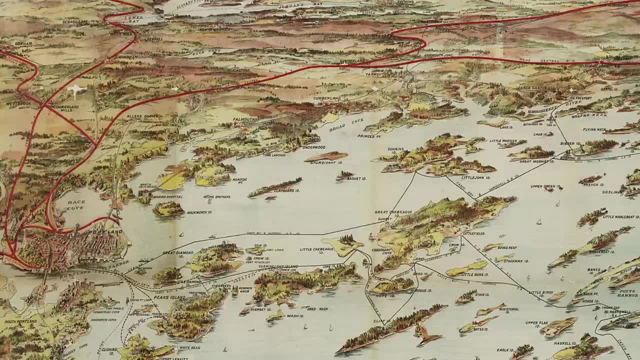 in by woodlands, but the city is spread to cover several other points and peninsulas, as well as a number of islands in the bay, such as Peaks Island and Great Diamond Island, which can only be accessed by boat. It's the smaller and older of the country's two Portlands, though it's often overshadowed by the. much larger city of Portland, Oregon. Portland Maine, named after an island off the coast of England, is older than its west coast cousin by over 200 years. As the story goes, two of the Oregon city's founders wanted to name it after their hometowns. One was from Boston and the 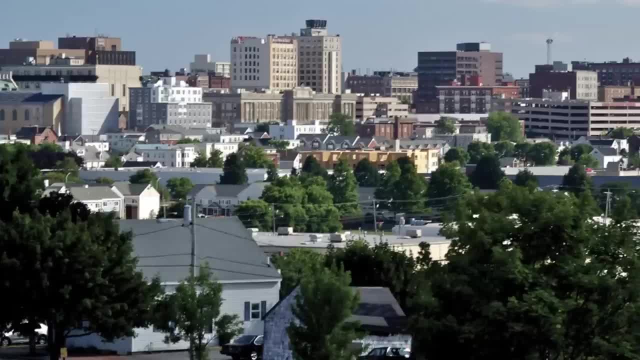 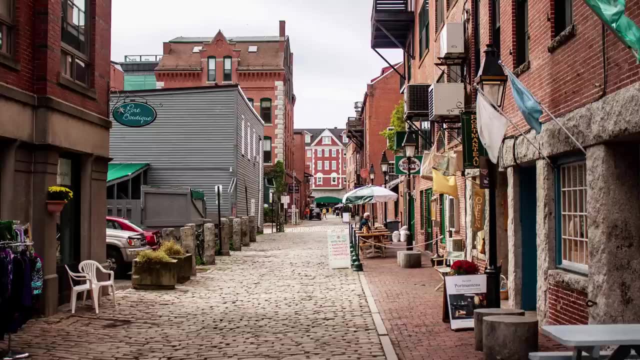 other from Portland and it got its name after the Mainer won a coin toss. The fastest growing. portland is a beautiful and historic city with a strong maritime tradition, delicious seafood and historic architecture. The state's capital, Augusta, is one of the country's smallest state. 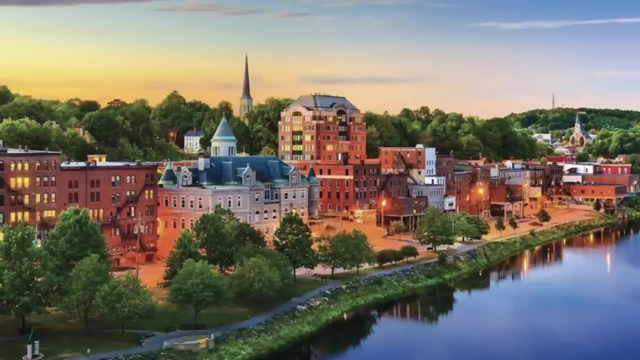 capitals Home to just 18,000 people. only the capital cities of Pierre, South Dakota and Montpelier, Vermont, have fewer residents. It's home to a small but scenic downtown along the Kennebec River and a beautiful capitol building set right against a forested hillside. 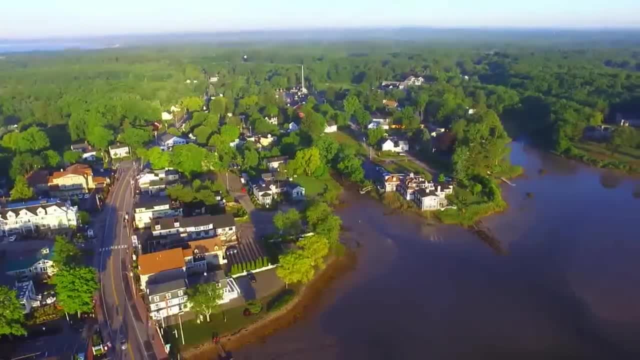 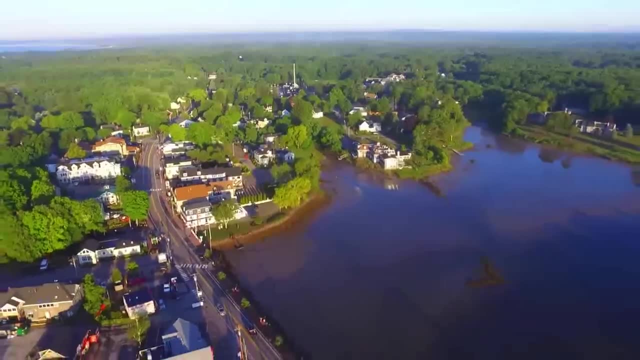 In terms of race, Maine is the least diverse state in the country. 92% of Mainers are white. the largest proportion of any state in the country. around 3% are multiracial, 2% Latino and 1% each are Black and Asian American. 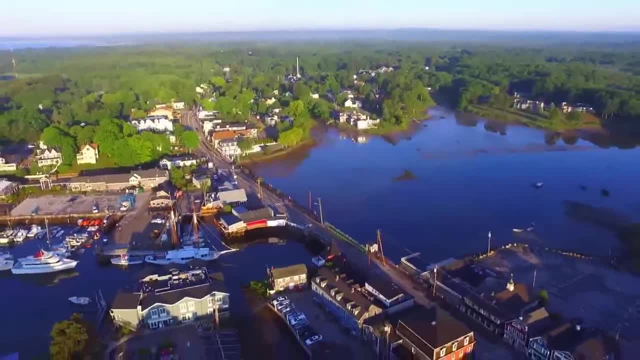 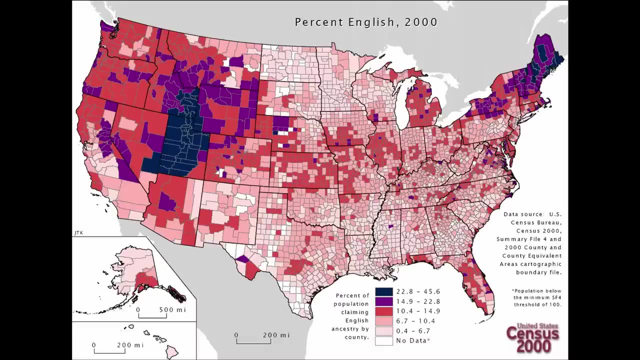 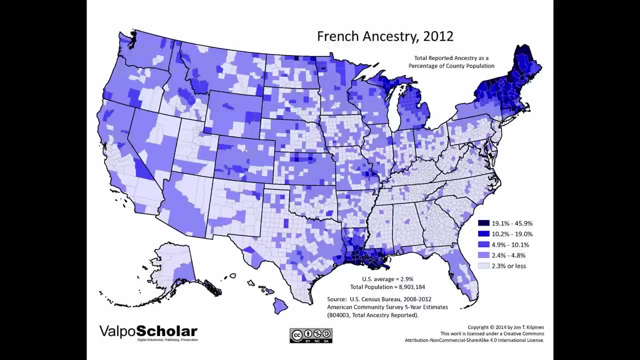 Most Mainers primarily trace their ancestry to either England, France or Ireland. It's one of just three states where English Americans are reported to be the most common ancestry group, though the numbers of Americans with ancestors from England are thought to be very undercounted If self-reported French and French-Canadian ancestry were combined. 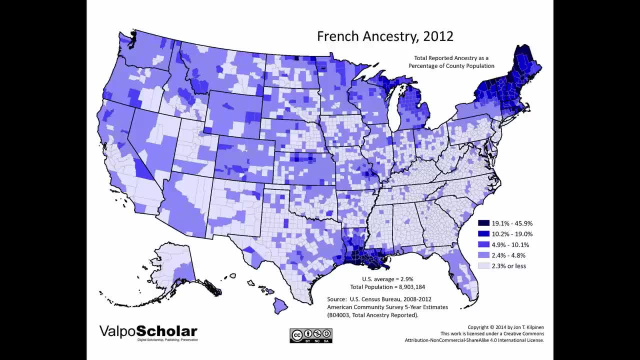 French-Americans would be the most common ancestry group. The largest ancestry group in the state is the Montparnasse-Maine group, with a fifth of Mainers tracing their ancestry to France mostly from the state's Acadian population, as well as later immigration from Quebec. The state has the highest proportion of French. 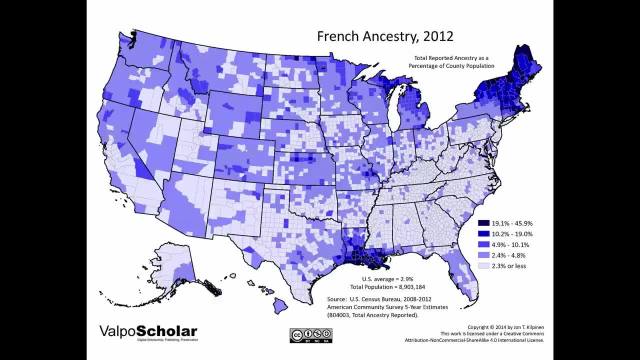 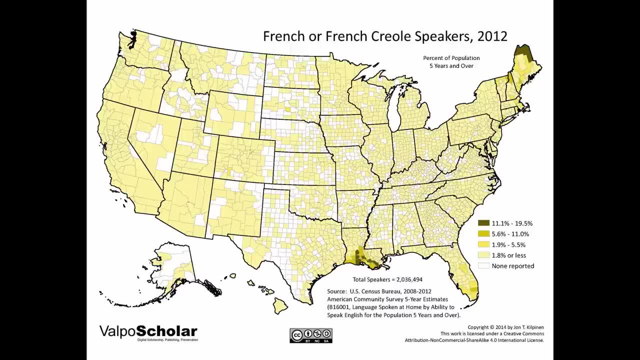 Americans in the country, even more so than Louisiana, and is home to the highest proportion of French speakers as well, with nearly 4% of the state speaking the language at home. The state has not been a major destination for immigrants in recent years. 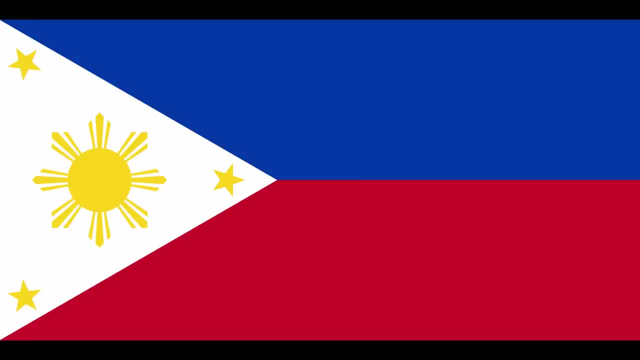 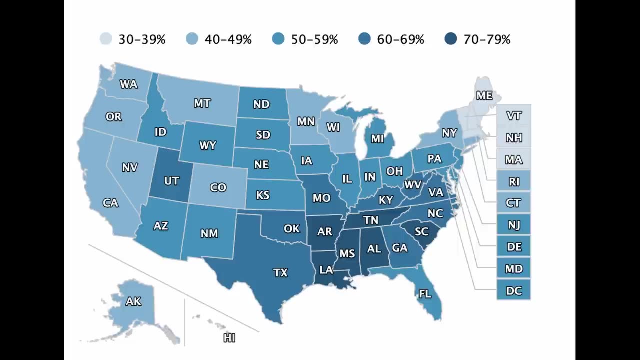 and though it's received some immigration from countries like Somalia and the Philippines, most immigrants to the state are from just across the border in Canada. Like much of New England, Maine is one of the least religious states in the country. Around a third of the population is not religious and only 20% of Mainers attend church regularly. 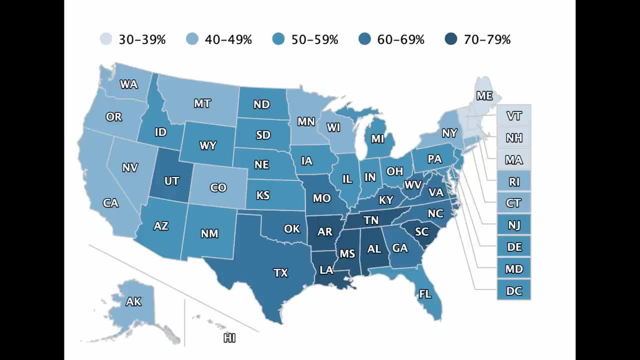 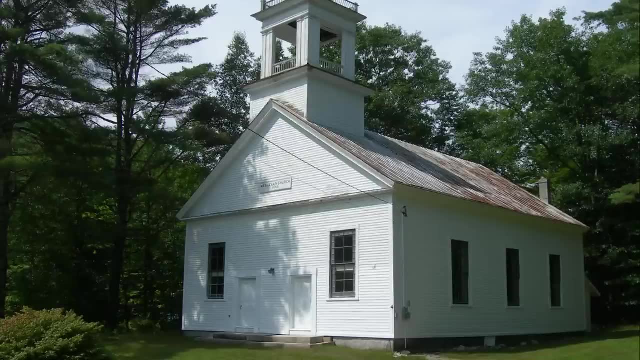 tied for the second-lowest rate with New Hampshire and surpassed by only Vermont. Most Mainers are Christian, the majority Protestant, in particular Mainline Protestant, but it has a fairly large Catholic population as well. About a fifth of the state's residents are 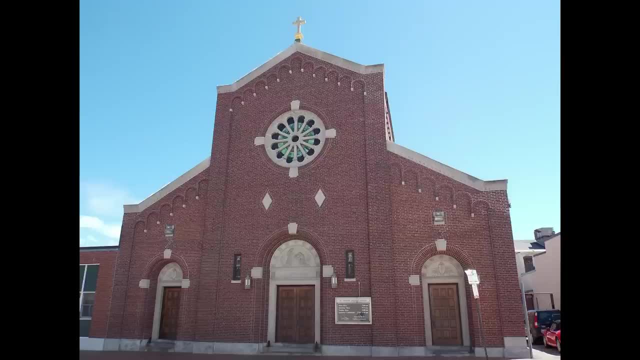 Catholic and about a third of the state's residents are Catholic, and about a third of the state's residents are Christian, in large part due to the state's significant French and Irish heritage. On top of that, it has one of the country's largest populations of residents. 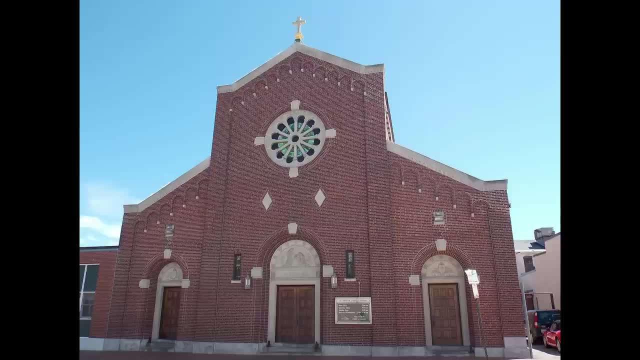 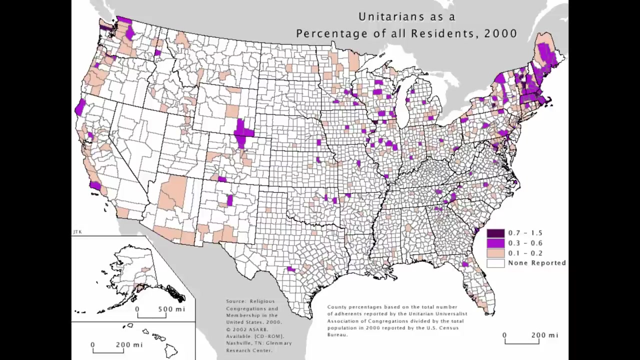 who practice faiths other than Christianity, Judaism, Islam, Hinduism, Buddhism or any of the other major world religions, at about 5% of the population, According to the Pew Research Center. these are mostly members of the non-Trinitarian Unitarian Church, though many 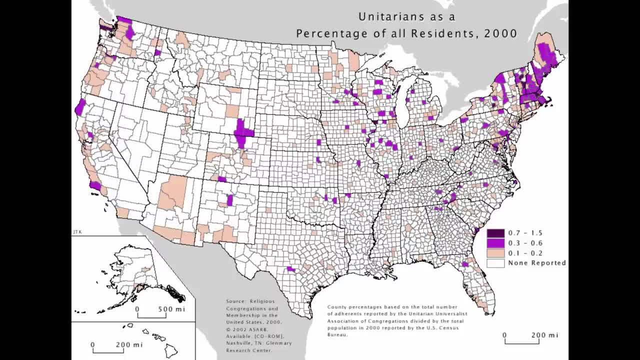 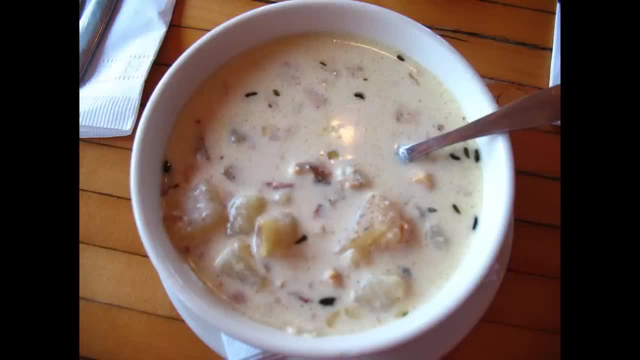 of them would likely consider themselves Christian as well as followers of various New Age faiths. The state is home to many different unique foods. Unsurprisingly, it has some of the best seafood in the country, like oysters and clam chowder, but it's most famous for lobster. 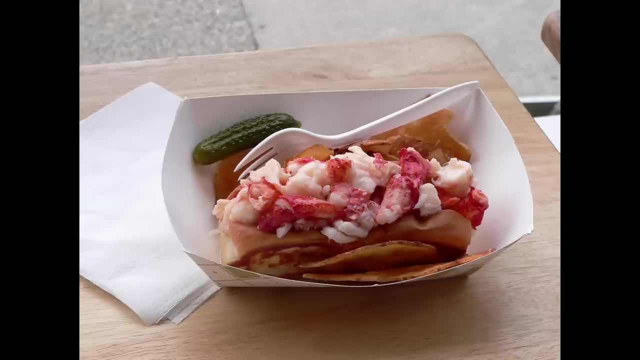 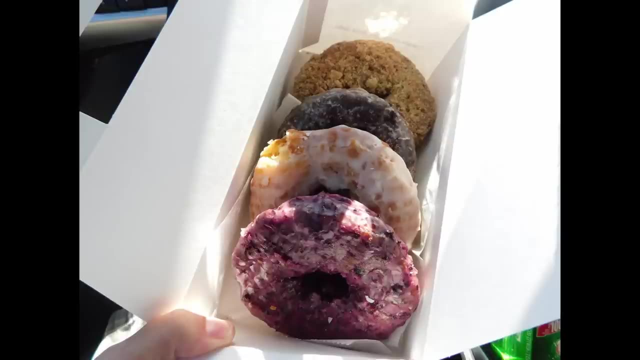 its largest export. Though it wasn't invented there, the lobster rolls become a Maine staple, Though something like doughnuts are thought to have originated centuries ago in Germany or the Netherlands. the classic American ring-shaped doughnut came out of Maine, A 16-year-old ship. 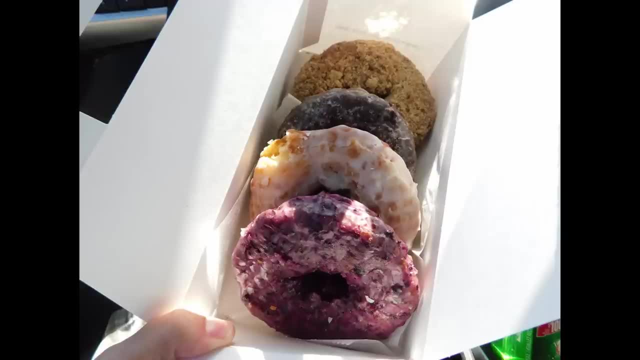 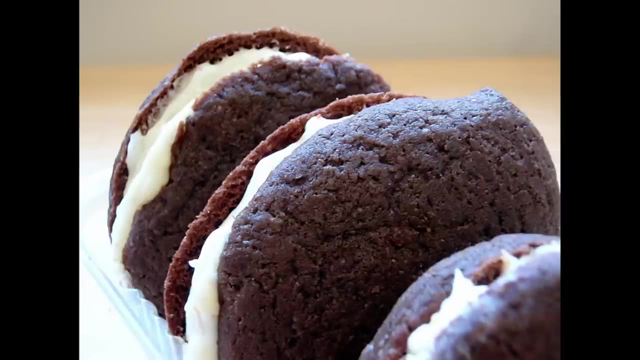 crewman named Hanson Gregory claims to have punched a hole in a doughnut for the first time while on board a ship and spread his method from there to local bakers. Whoopie pies are a classic Maine dessert and moxie is a regional soda that's very popular within the state. They have their 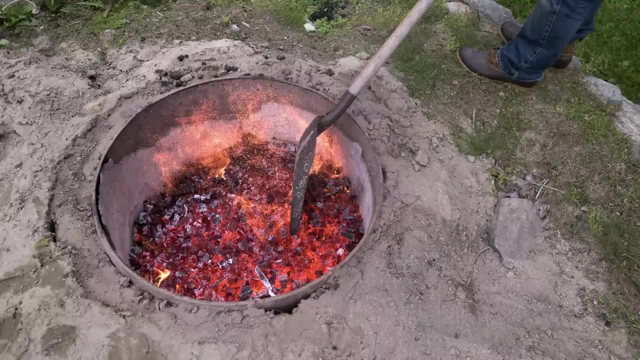 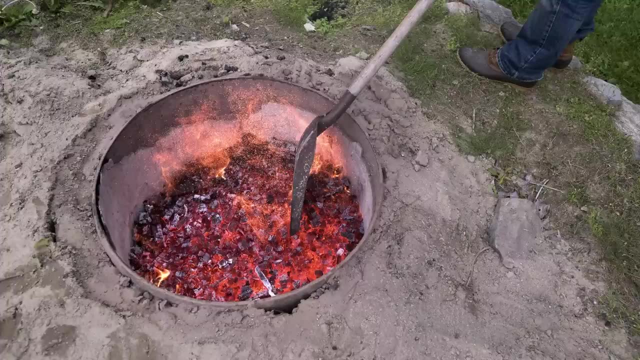 own variety of baked beans which are cooked in a pit in the ground, called bean-hole beans. Mainers speak with a very unique accent and dialect of English. It's similar to other New England accents but can get pretty strong and distinct, especially the further you go into the. Down East Writers like Henry Wadsworth Longfellow and EB White. the author of Charlotte's Web, were born in Maine, as is Stephen King, who sets many of his books in the state. The state has no major league sports teams and its residents tend to root for Boston-based teams. Its largest newspaper. 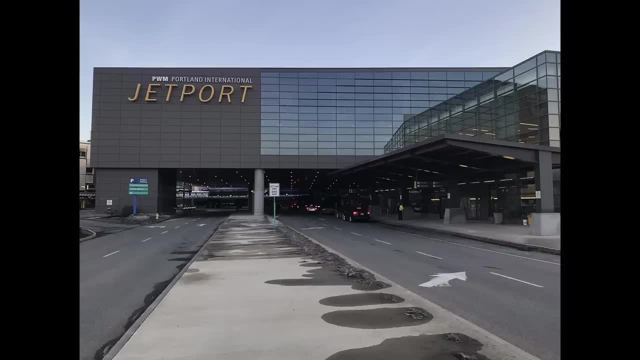 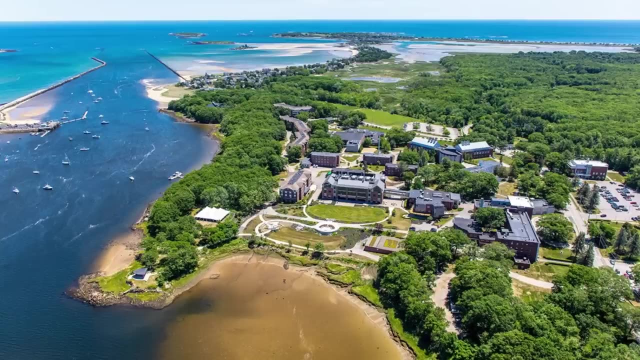 is the Portland Press-Herald, and its busiest airports are the Portland International Jetport and the Bangor International Airport. Major colleges include the University of New England, with campuses in Biddeford and Portland, the University of Maine, which sits in the town. 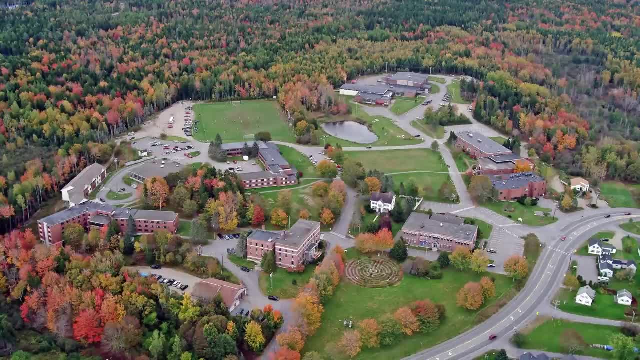 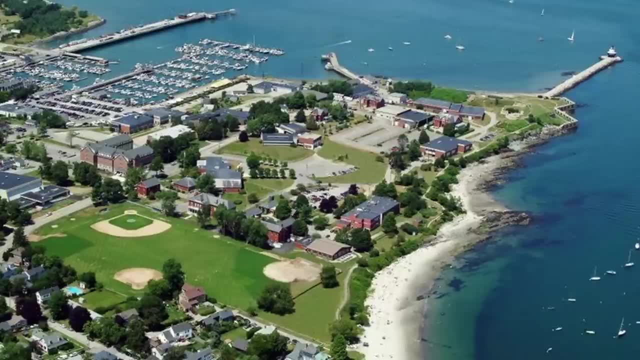 of Orono, on an island in the Penobscot River outside of Bangor. the University of Southern Maine, with three campuses across the region and Southern Maine Community College in South Portland. It's also home to a number of smaller or well-known liberal arts colleges. 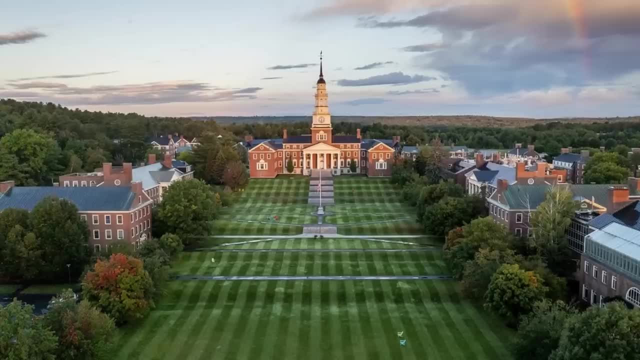 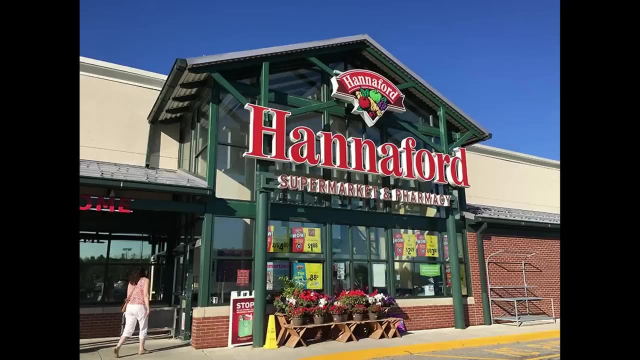 like Bowdoin in Brunswick, Bates in Lewiston and Colby in Waterville. Major companies headquartered in Maine include the Baker Company, New England supermarket chain, Hannaford and LL Bean. It's the only state in the entire Northeast that's home to a national. 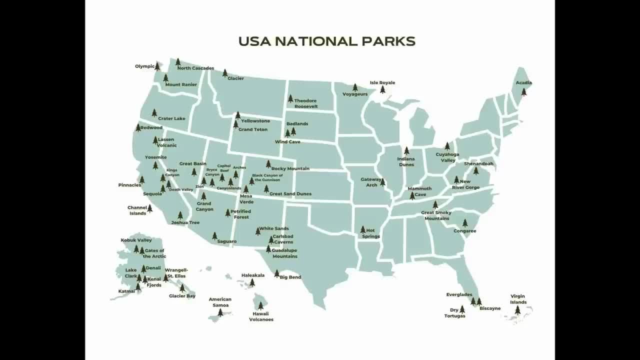 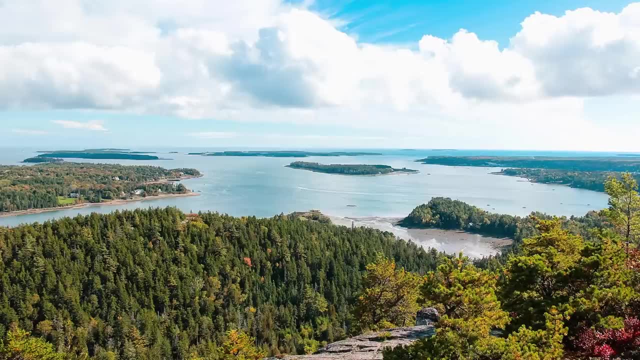 park. Acadia National Park is a beautiful park located mostly on Mount Desert Island, as well as the islands and peninsulas, and it is home to Cadillac Mountain, the tallest mountain on the Atlantic coast of the US. National parks are few and far between in the Eastern US and with many 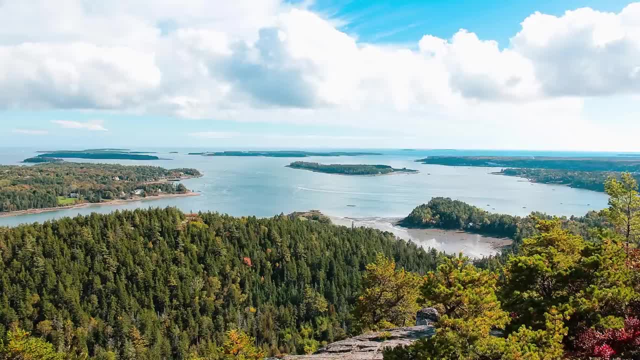 major cities a weekend trip away. Acadia draws millions of visitors to the state. It's the fifth most visited out of the country's 63 national parks, bringing in nearly 4 million people a year. Some famous Mainers include Stephen King, Milton Bradley, Anna Kendrick, Patrick Dempsey and Henry. 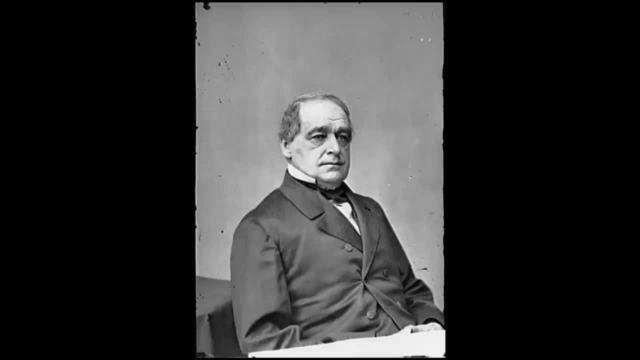 Wadsworth. Longfellow Presidents have as of yet come from Maine, though it has been home to several influential political figures throughout history. Hannibal Hamlin had represented the state in the House and Senate and served as governor before he became Abraham Lincoln's vice president. 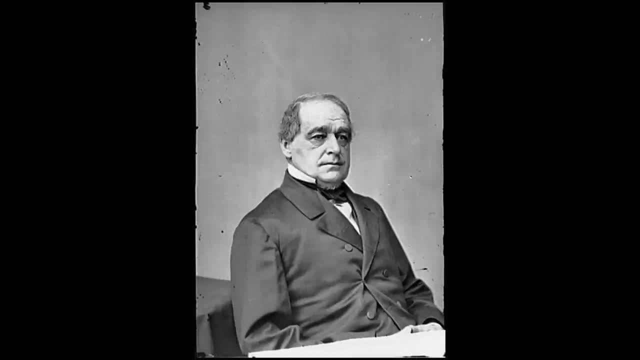 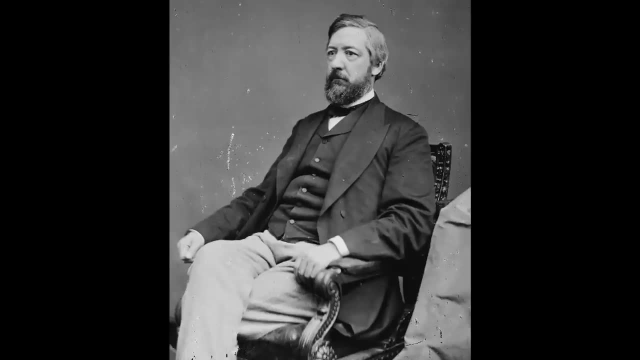 though he was replaced on the ballot for re-election after one term. Speaker of the House, James Blaine later represented the state in the Senate, served twice as Secretary of State and became the Republican nominee for president, though he lost to Grover Cleveland. 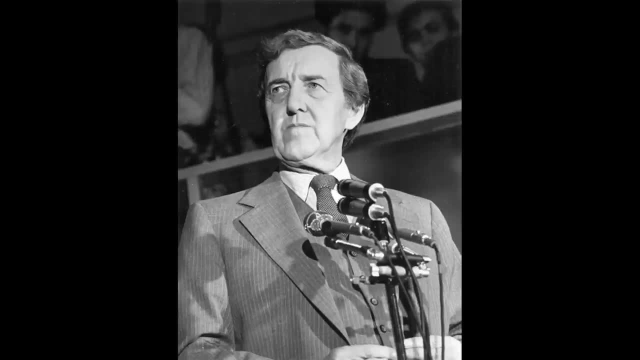 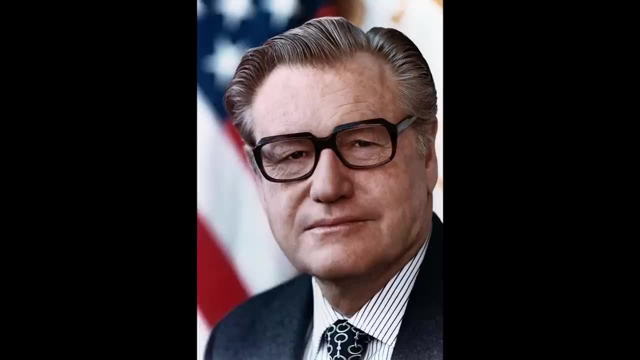 And Ed Muskie was governor, senator, secretary of state and the Democratic president. He was the Democratic nominee for vice president in 1968, losing to Richard Nixon and Spiro Agnew. On top of that, New York Governor Nelson Rockefeller, who led an influential faction. 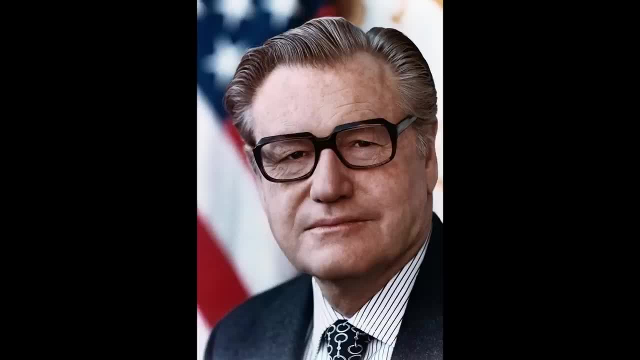 of liberal, so-called Rockefeller Republicans throughout the mid-20th century, serving as Gerald Ford's vice president, based his political career out of New York but was born in Bar Harbor where his family vacationed. Another wealthy and influential political family- the Bush family. 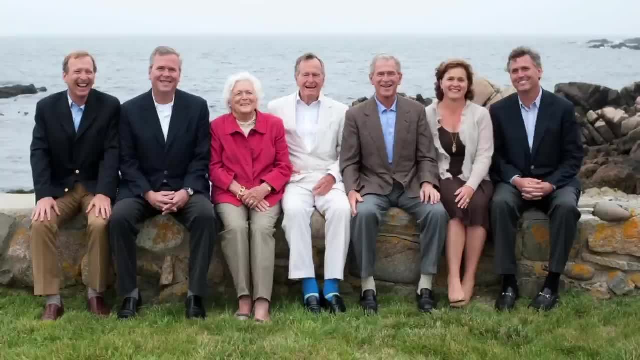 which produced two presidents, built their political careers out of Connecticut and Texas, but spent significant time at Walker's Point, a family estate in Kennebunkport which served as a summer White House of sorts during George HW Bush's presidency. 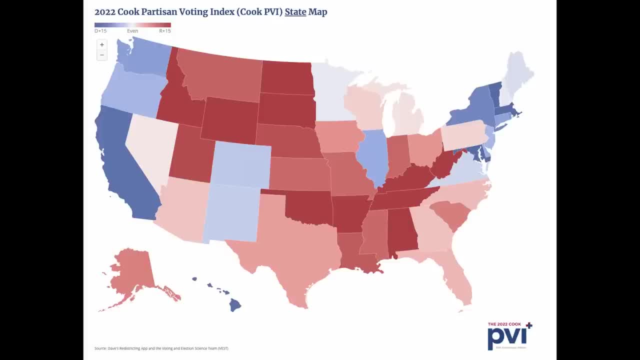 Maine is politically one of the most moderate states in the country and has a strong independence streak. Its politics are arguably some of the most unique in the US. Its Cook Partisan Voting Index, or PVI, is D plus 2, meaning that in a given year 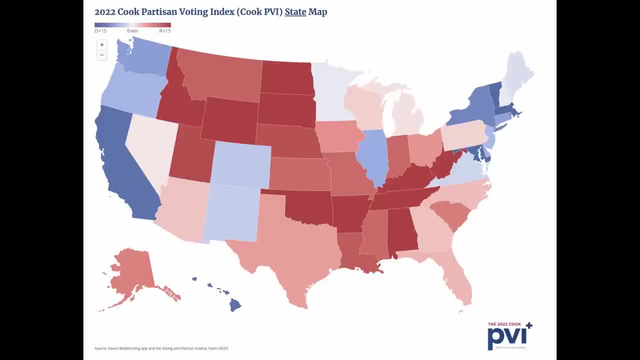 the state outperforms the Democratic nominee by only 2% on average. For reference, the classic swing state of Pennsylvania has the same lean towards the Republican Party. The state voted for Republicans by large margins until 1992, when it became a safe blue state. It was one of just two states where third-party candidate Ross 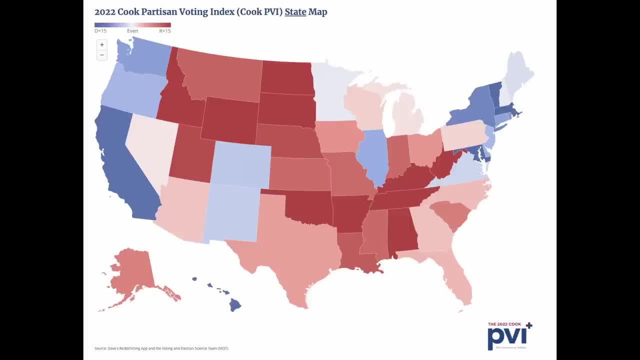 Perot came in second place and Green Party candidate Ralph Nader broke 5% of the vote in 2000,, as did Libertarian Gary Johnson in 2016.. Since 2016,, the state has become much more competitive. Maine was the first-ever state to implement a vote of 5% in 2016.. Maine was the first-ever state to 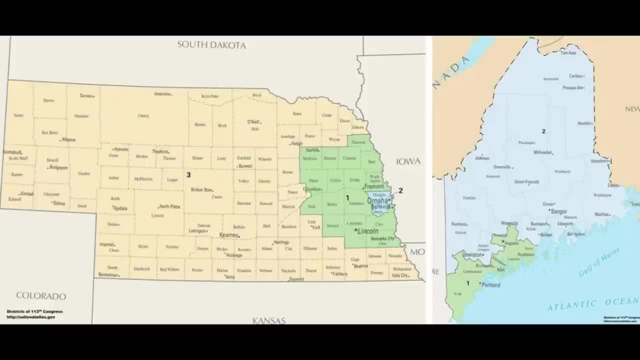 implement a vote of 5% in 2016.. Maine was the first-ever state to implement a vote of 5% in 2016.. Maine was the first-ever state to implement ranked-choice voting and, along with Nebraska, is one of just two states that splits their electoral college votes by congressional district. 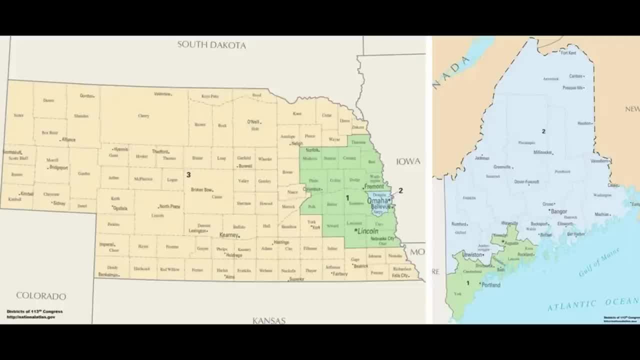 Maine currently has four electoral votes. It gives two to the winner of the state overall and one each to the winner of each respective district. Because of this, it split its electoral votes in both 2016 and 2020, with Clinton and Biden winning three votes each and Trump one vote. 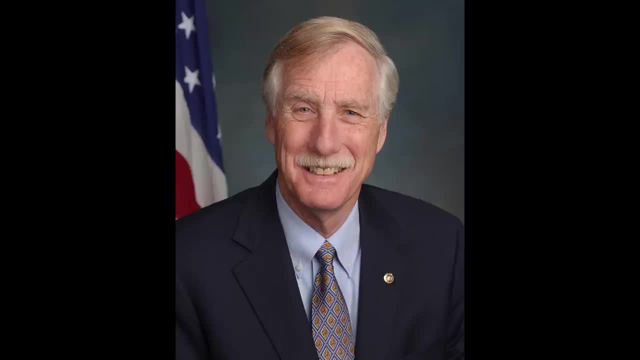 due to his wins in the state's second congressional district. It's one of just seven states who two senators are not part of the same political party, and one of just three represented by an independent senator. One of its senators, Angus King, is an independent who caucuses with the 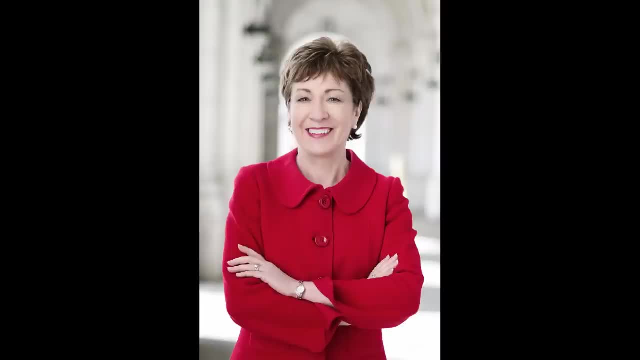 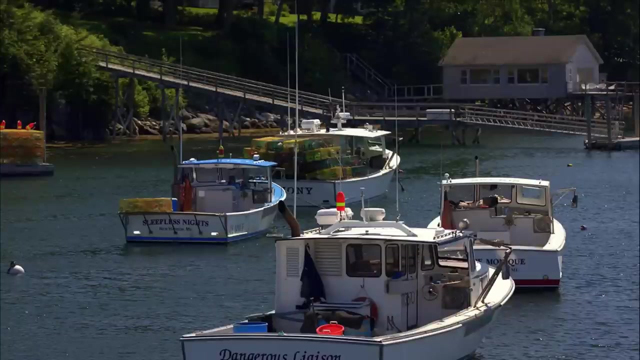 Democrats and the other, Susan Collins, is a Republican. Both are considered among the most ideologically moderate members of the Senate. Both of Maine's representatives in the House of Representatives are Democrats, as is its governor, Janet Mills. As this series goes deeper into the geography and history of the United States, I hope to provide 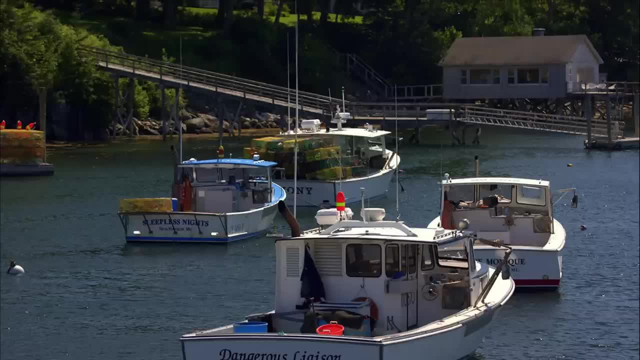 more insight into economic changes that have occurred across the country, in states like Maine and others. Economic concepts around finance and statistics can seem difficult to grasp, but there's a fun and easy way to learn more about them. Today's sponsor, Brilliant. 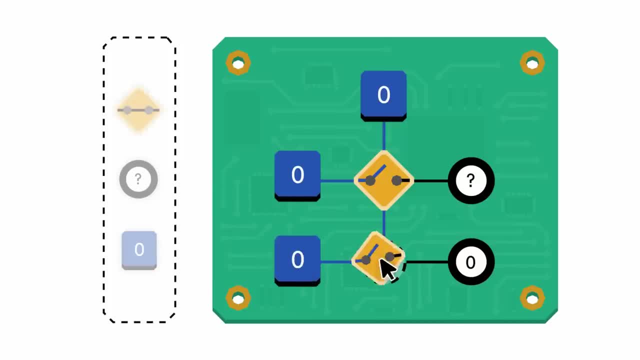 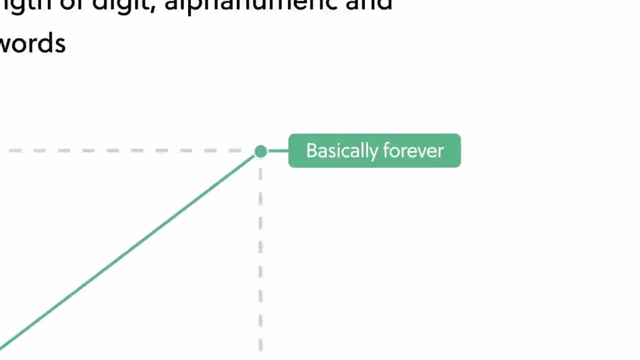 is the best way to learn data science, math and computer science in a fun and interactive way. Brilliant has thousands of courses available and adds new ones every month. It doesn't matter if you have lots of experience or are just getting started. Brilliant will customize their content. 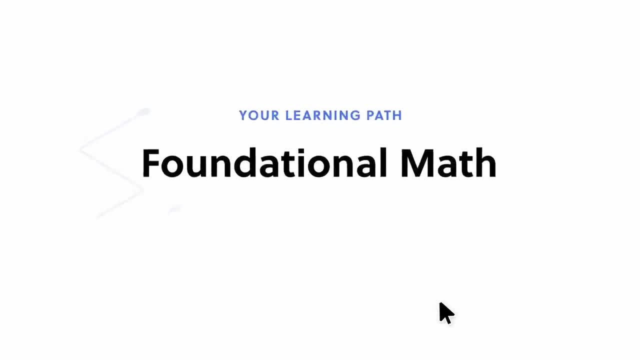 to fit your needs. If you're interested in learning more about data science and math, you'll want to take a look at their course and let you work at whatever pace works best for you. Data skills are only becoming more in demand, which is why I love their Data Analysis Fundamentals. 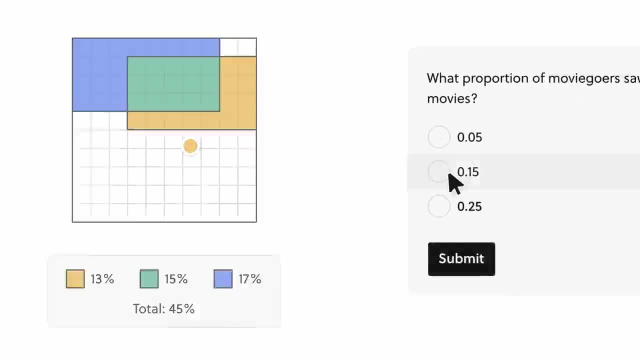 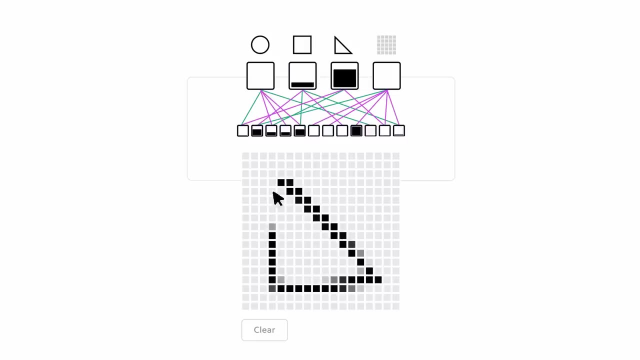 course. With just a few quick lessons, you get to analyze real data and draw interesting conclusions from it. This kind of analysis is a huge part of geography and is a strategy I use frequently when I'm making videos, for That is Interesting. The best part is my viewers get the first.